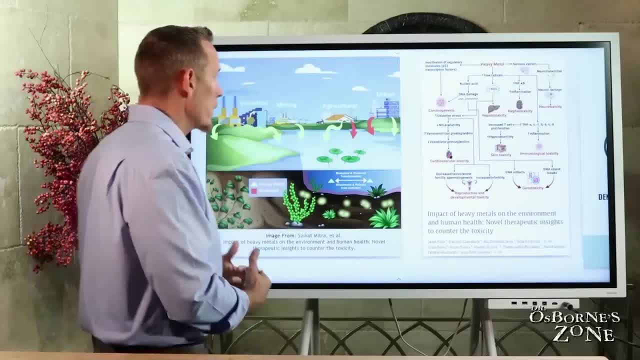 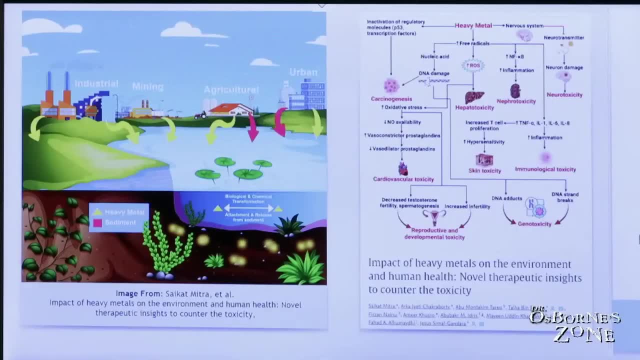 insecticides are contaminated, are produced with heavy metals, And then we have urban exposure. A classic example of this for those of you who remember Flint, Michigan, where the infrastructure of this town, where the pipes were lined or had lead that was leaching. 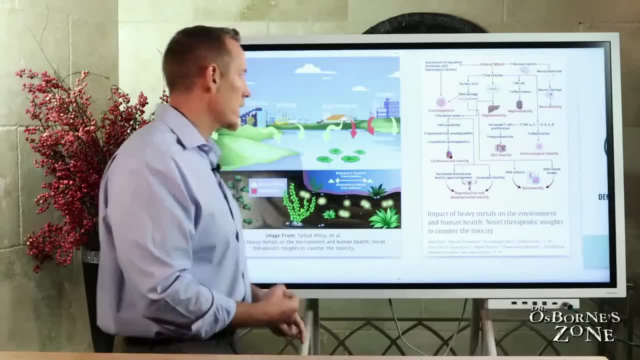 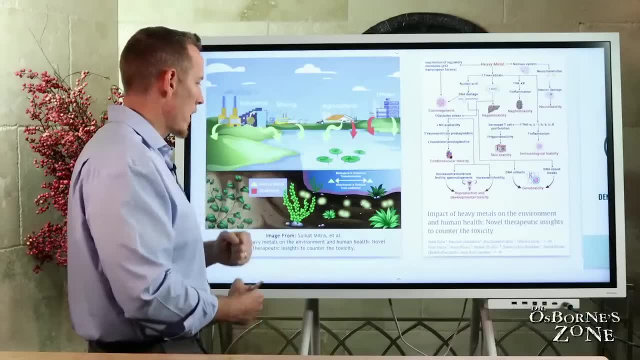 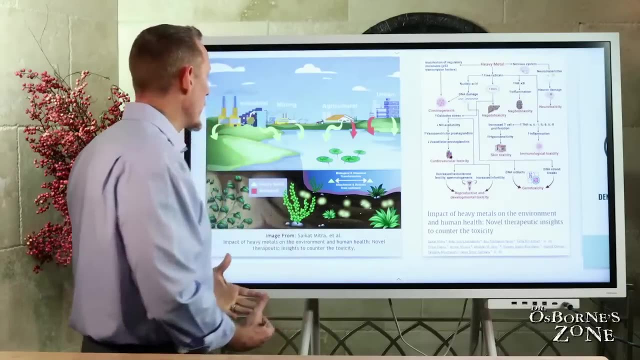 into the water supply, causing many, many folks in that city to become sick. So we've got all these potential areas where we're using metals in different processes. We use metals in things like generating batteries and computer parts, So they end up in our groundwater And that's what. 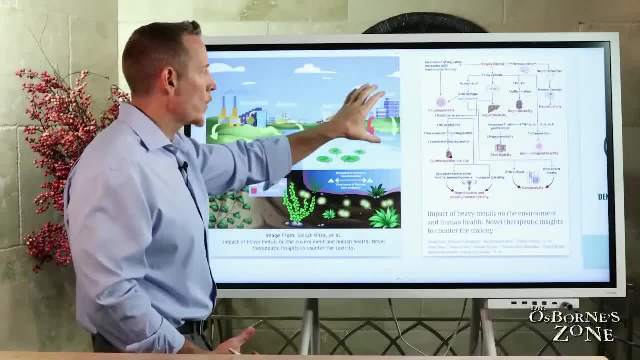 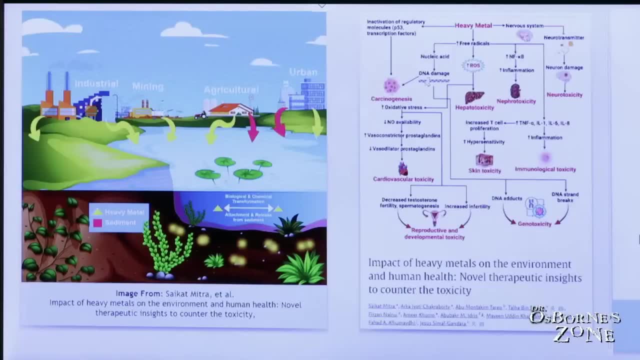 you know this is referring to is from all of these potential ways we can have exposure to metals. It's generally the technology generates a groundwater runoff, And so we end up with these metals being found in our rivers, in our lakes, in our rivers, in our rivers, in our lakes, in our 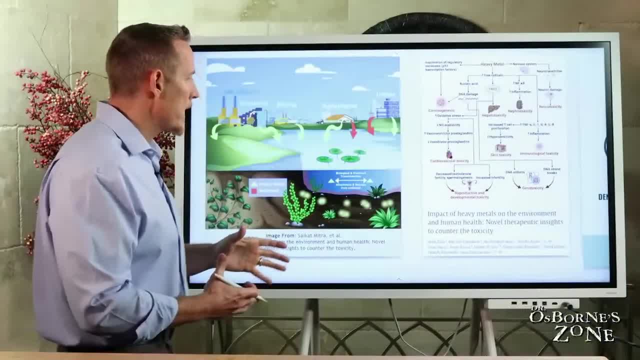 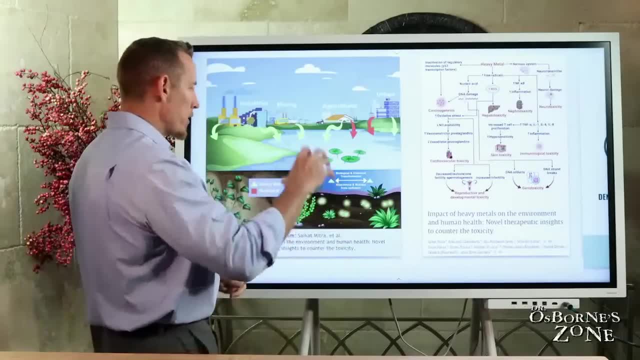 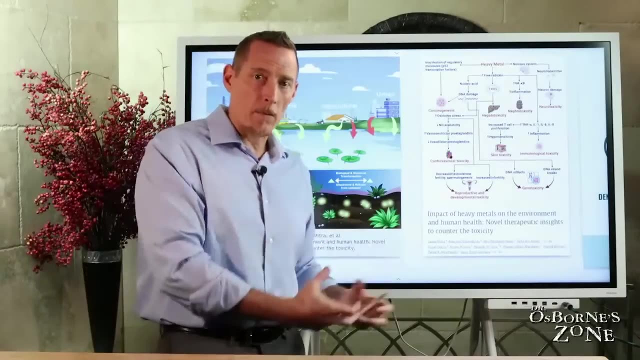 lakes, in our bodies of water, And so then we get biological and chemical transformation of these metals, And so many of them are from the water, you know, go into the sediment, into the soil, find their way into the plants, And then from the plants, find their way into the actual animals. 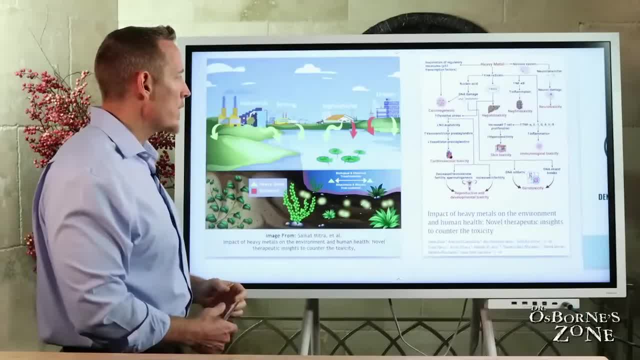 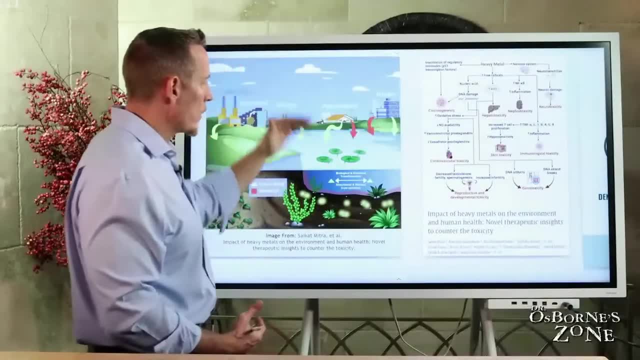 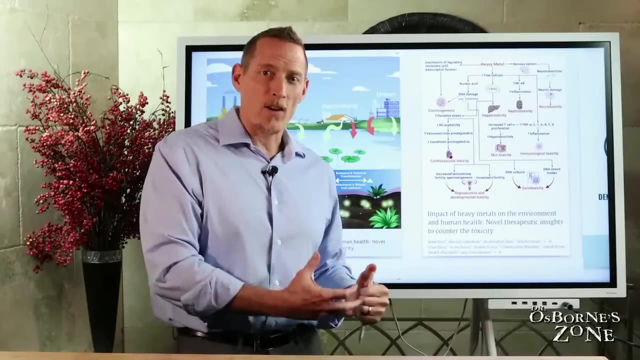 through consumption. And so this cycle of heavy metal exposure can go on and on, And so we get again, we get the byproducts of industry into our water and into the water supply, And so we get into our soil, And again, many of our plants are designed to grow in that very same soil, that's. 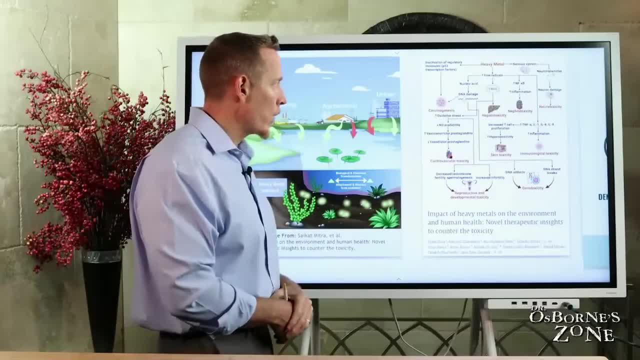 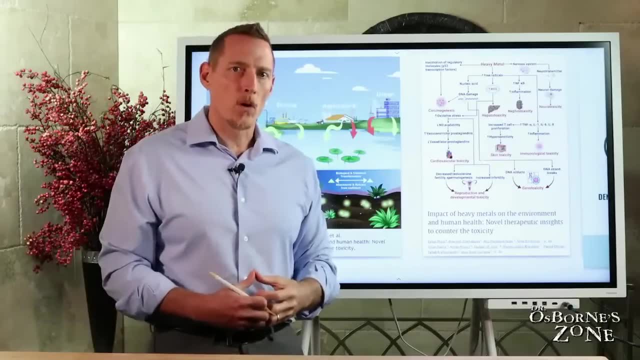 being contaminated with these metals, And so it ends up in our food supply as well. So our exposure is pretty ubiquitous. at this point, If you live in modern, civilized area of the world, your exposure to toxic metals is pretty much an imminent thing. It's something that you're going to want to be. 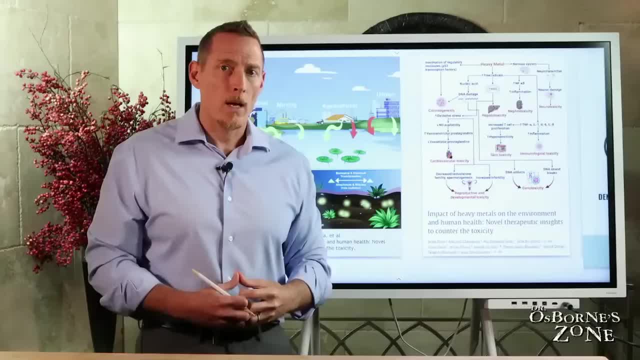 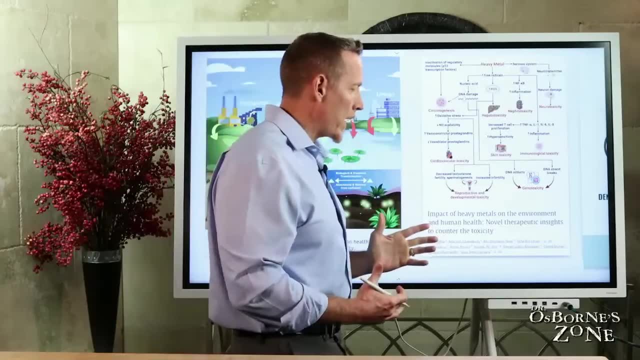 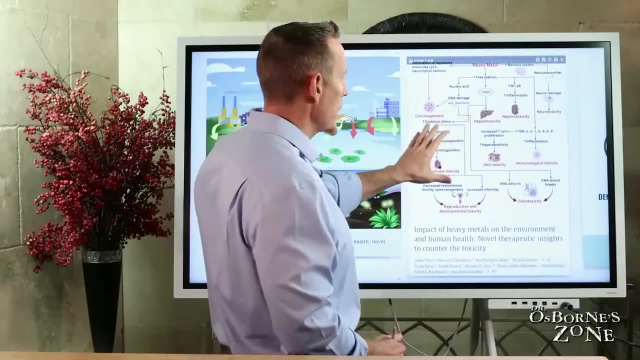 concerned about and that you're going to want to do as much to protect yourself as you possibly can, And we'll talk about some of those mechanisms of protection here shortly Now. why should we be concerned about heavy metals? What's the danger in being exposed? Well, let's take a look at this diagram again from: 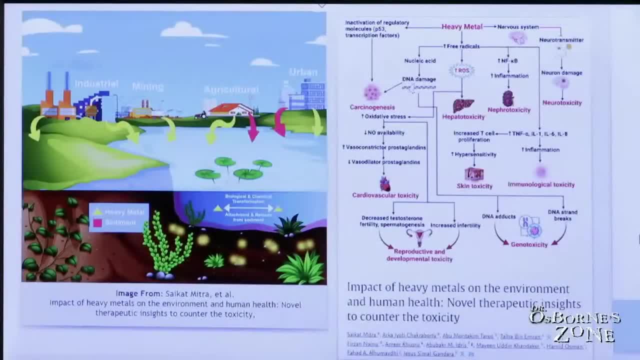 the same research review on the topic, But you can see here at the top. heavy metals can impact a number of different systems in the body. We have impact on the nervous system. A lot of the side effects of heavy metals actually impact or affect the brain and the nerves, or 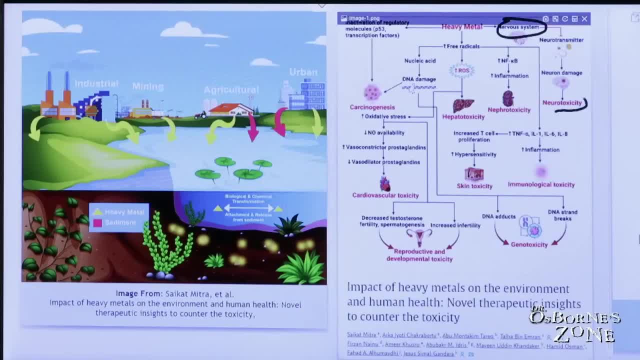 neurotransmitter production, leading to neurotoxicity, And we'll dive into some of those symptoms here shortly. We also have heavy metals that can actually impact your kidneys, And so we get this what's called nephrotoxicity right. So damage to the kidneys directly. 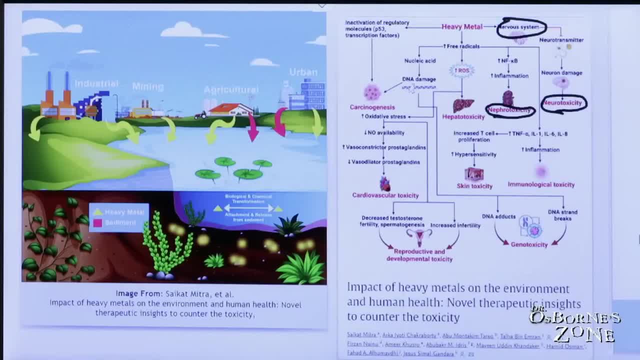 Perfect example: lead is very nephrotoxic. We have the hepatotoxicity. This refers to the liver, The hepatotoxicity again to the liver. So for those of you who maybe didn't take biology or anatomy, in physiology hepato refers to liver, nephro refers to kidney, And then over here. 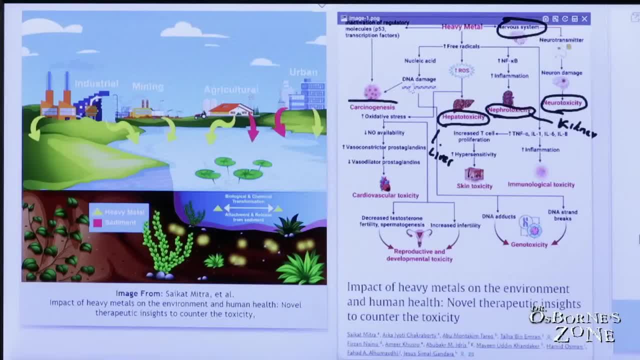 on this side of the equation, we have carcinogenesis. This is cancer, right? So these are carcinogens. They can drive the process of cancer by driving the process of oxidative stress- Oxidative stress, if you've heard the term. free radicals, many of these metals. 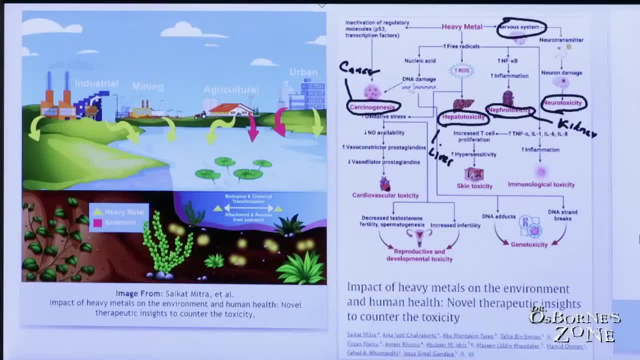 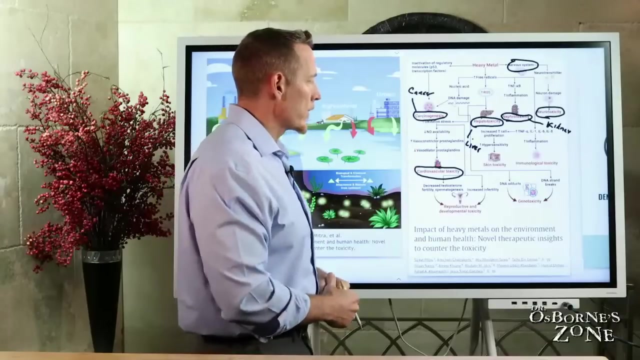 behave and act as free radicals, leading to, again, oxidative stress that can create or potentiate cancer. We also have cardiovascular or heart toxicity, And this has to do with metals interfering with a number of the different chemicals that help regulate vasoconstriction and vasodilation of the arteries in the blood system or in the circulatory. 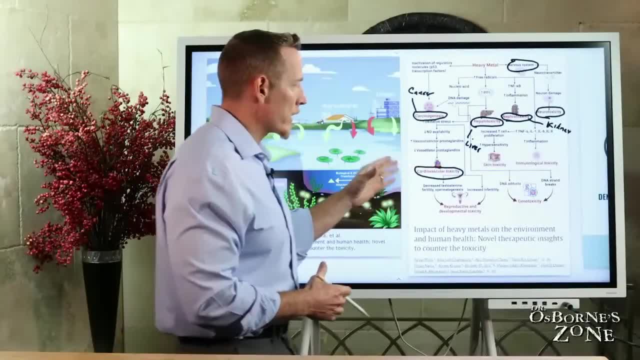 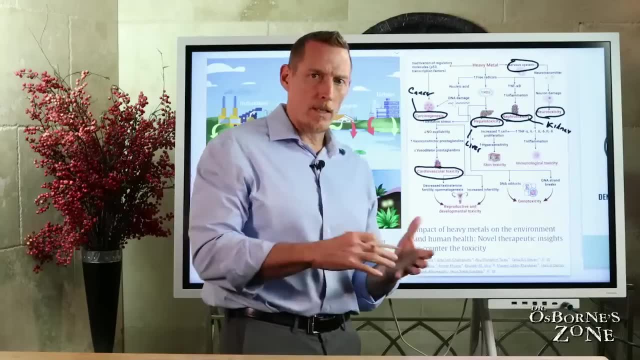 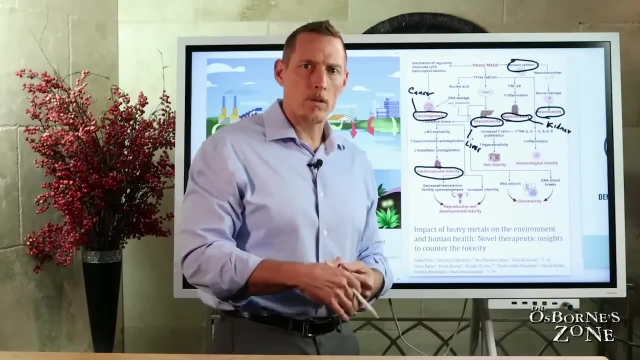 system, And so this can lead to things like high blood pressure Again. another example we see is blood toxicity having the capacity to do this. Some of the metals actually interfere, like cadmium and lead, and arsenic can actually interfere with calcium and magnesium and potassium. 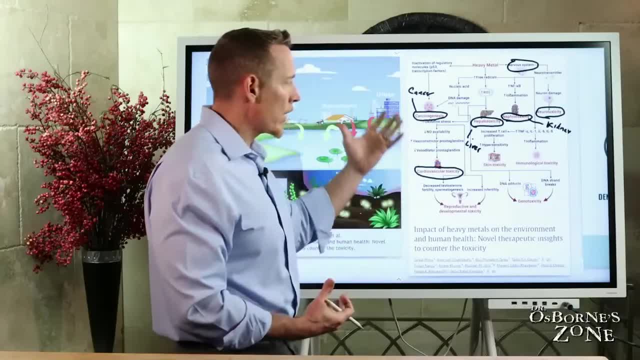 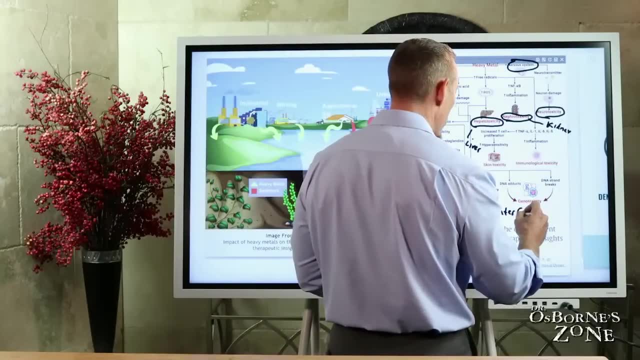 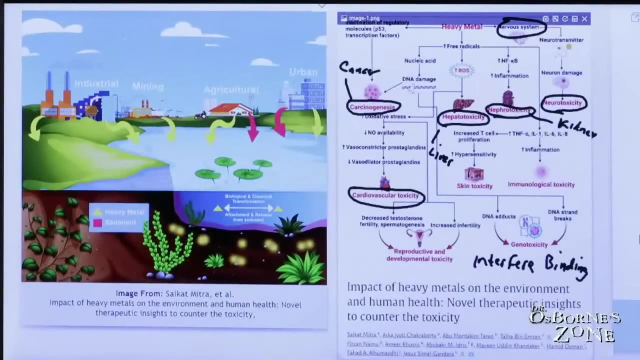 and their functions. As a matter of fact, one of the reasons metals are toxic is because of that and it's not listed on this diagram, but they actually interfere, compete for binding sites from other minerals, So binding of magnesium and calcium and zinc, And so what happens to a lot of people? 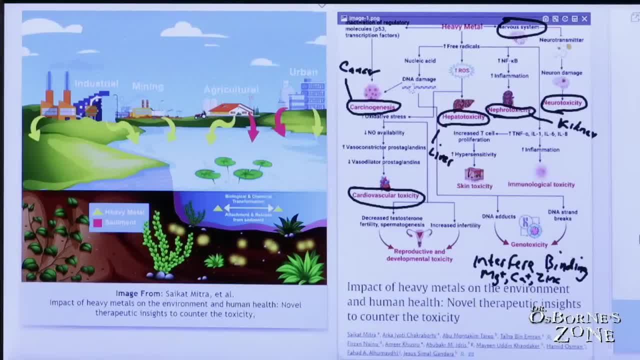 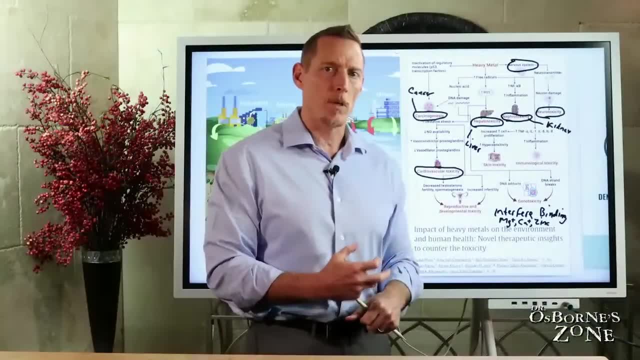 is when they're exposed chronic, chronically to heavy metals. these metals will interfere with the binding sites of these other minerals, leading to the symptoms of deficiency of those minerals. And so you add that to all these other potential impacts and effects, We also have metal. 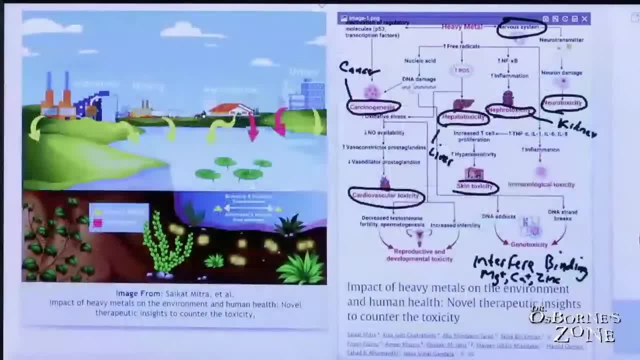 affecting the skin. So we can get rid of that, We can get rid of that, We can get rid of that. So we skin toxicity. a lot of the symptoms of metal exposure occur as inflammatory skin disorder, and then we can also get immunological toxicity. so this has to do with, you know, immunological. 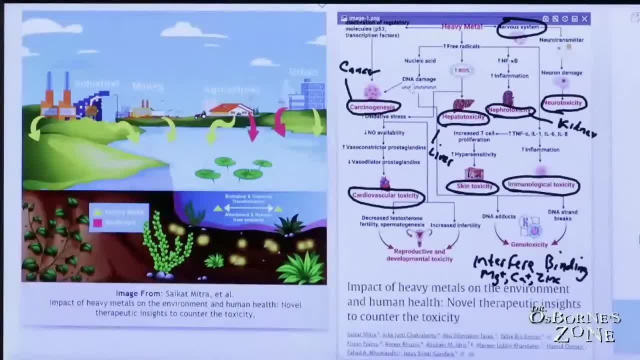 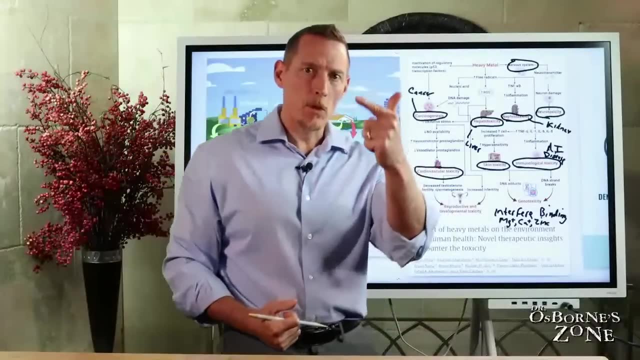 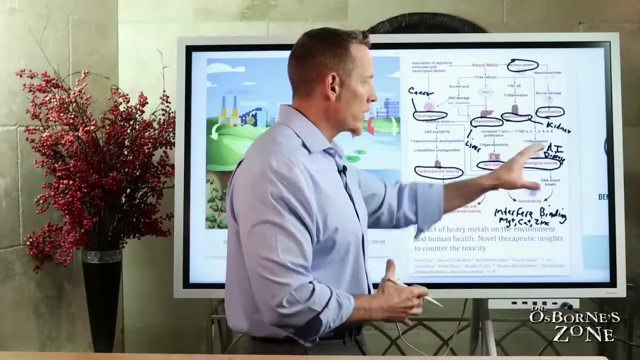 meaning the immune system, so an overreactive immune system. this is actually one of the triggers for autoimmune disease. so you know, if you ever heard me talk about you know the four primary drivers or primary triggers of autoimmune processes. you know food chemicals, microbial imbalance and number four is nutritional deficit. well, heavy metals fit the bill of the chemical. 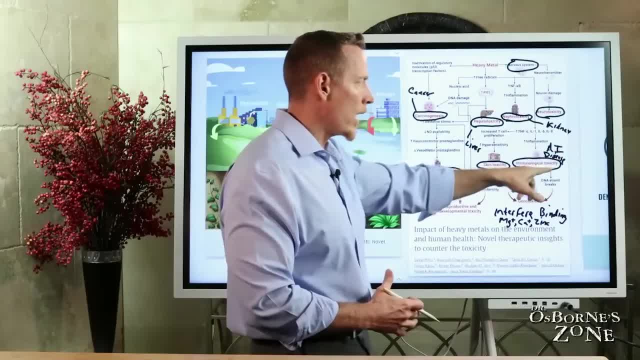 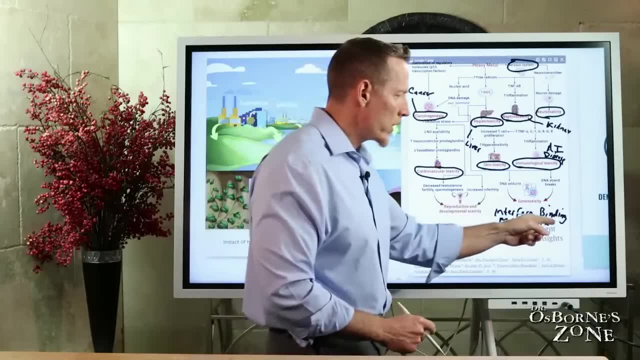 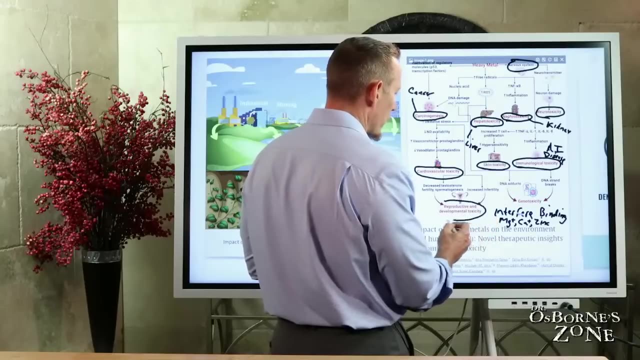 category, we consider these toxic chemicals. so, as a driver, as a category, they drive autoimmune disease, but they also drive it nutritionally because they interfere with nutrients doing their job okay. so we also know that metals can affect the reproductive system. so metals can impact fertility both in men and in women. we get, you can see, here- 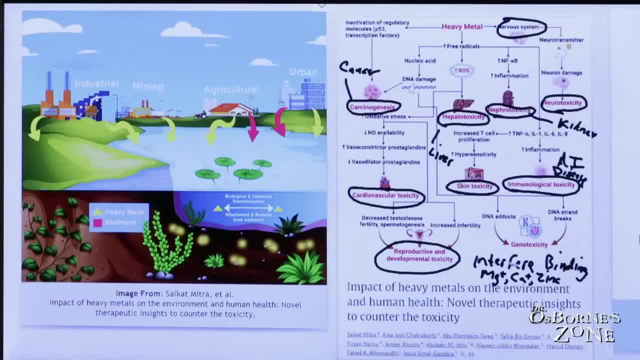 decreased testosterone in men and decreased spermatogenesis, so can be a very big problem in terms of fertility. and then we have genotoxicity. we know metals can actually do damage to dna, so dna strand breaks leads to damage to the genome, which makes it harder for cells to 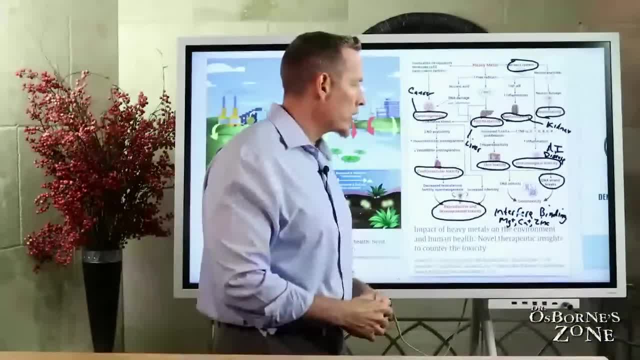 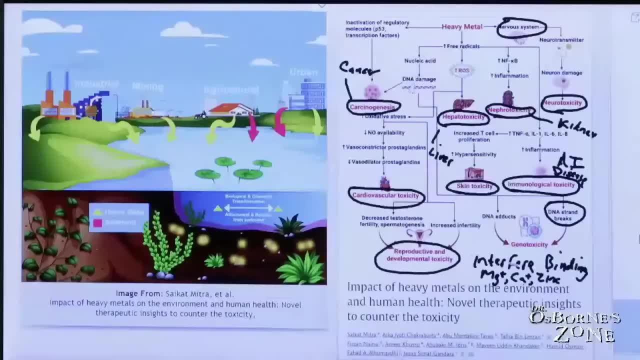 heal and replicate and maintain themselves, since we can get an increased risk for many problems that can cancer. this, this and this go kind of hand in hand, because genotoxicity can contribute to or increase the risk for developing carcinogenic problems or cancer-based problems as well. so these are kind of categorically the different systems that we know. heavy metals: 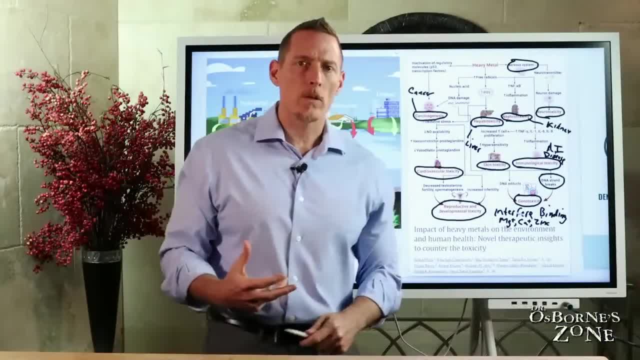 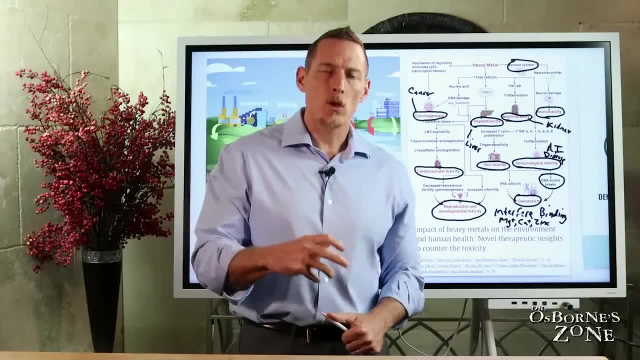 can actually impact. now i want to make a clear distinction with heavy metal, because there's there's kind of two ways people get exposed. there's heavy metal from an acute perspective, meaning you were exposed to massive quantities in a very short period of time and you actually are. 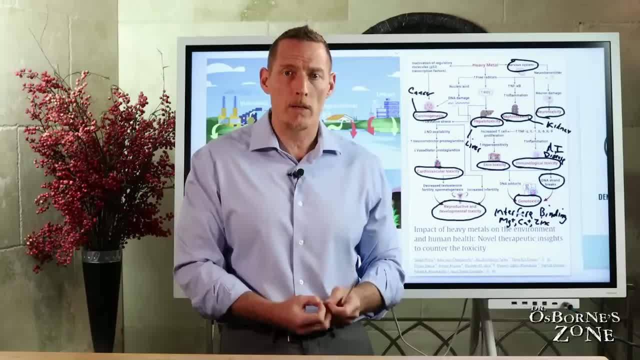 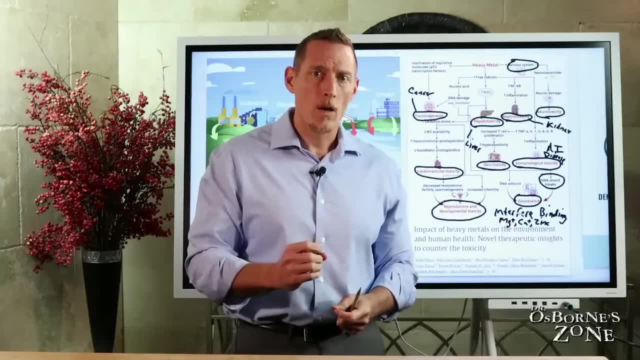 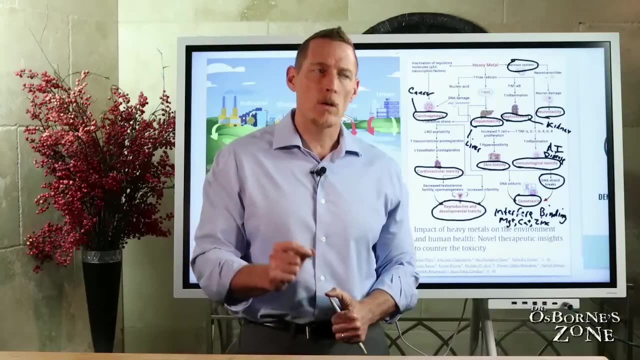 suffering with an acute poisoning. now, an acute poisoning of heavy metals can kill you. it they can be terminal acute poisoning, and what I'm really referring to here tonight with you are not those that suffer from acute poisoning who got mass exposure. we're talking about what's known as is a term. there's a term. 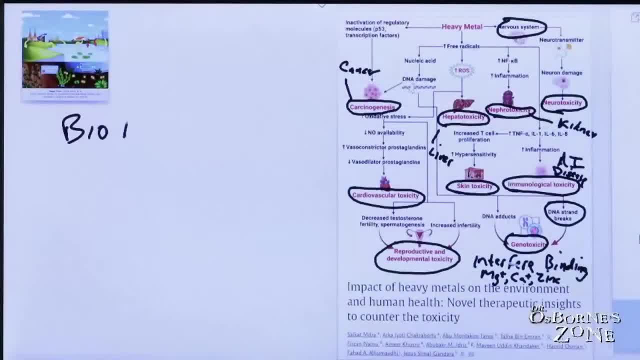 in research and science that's oftentimes used, and that term is bio accumulation. okay, meaning it, it's the slow dose which accumulates in your tissue or tissues. and it's the slow dose which accumulates in your tissue or tissues. and it's the slow dose which accumulates in your tissue or tissues. 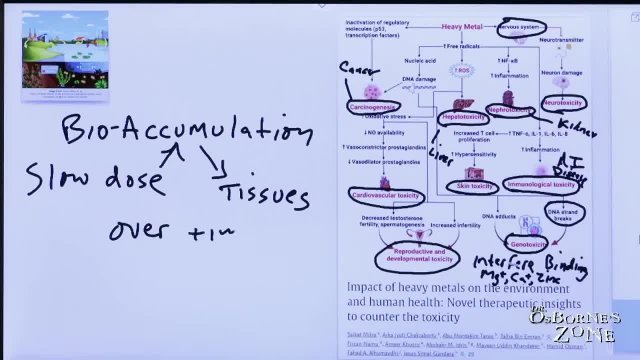 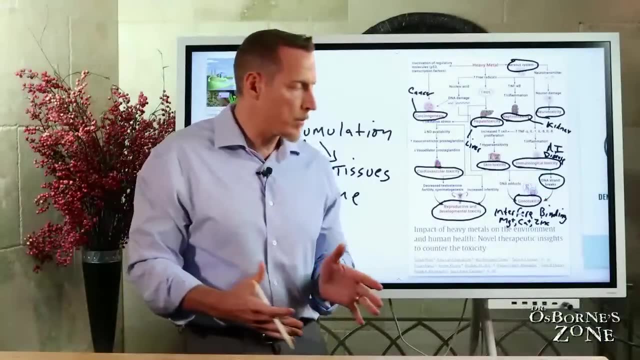 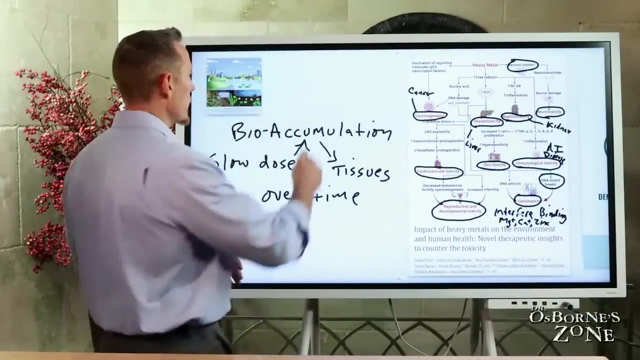 over time. so think of heavy metal, as we're talking about it tonight, as a slow poison, not a fast-acting poison, and so this is where you could be getting low levels or low dose exposure over many, many years. as a matter of fact, you know the, the baby boomer generation of our time we called. we call that that. 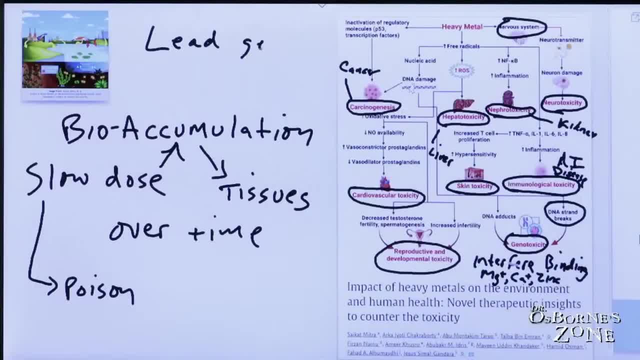 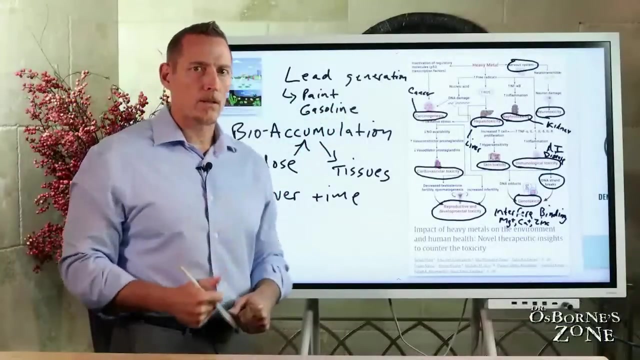 generation. you know the lead generation because they were exposed to lead in things like paint. remember the old paint contained lead as a pigment. they were exposed to lead in the gasoline. if you were born before you know 1975 ish, you may remember that there was actually leaded gasoline and unleaded gasoline as 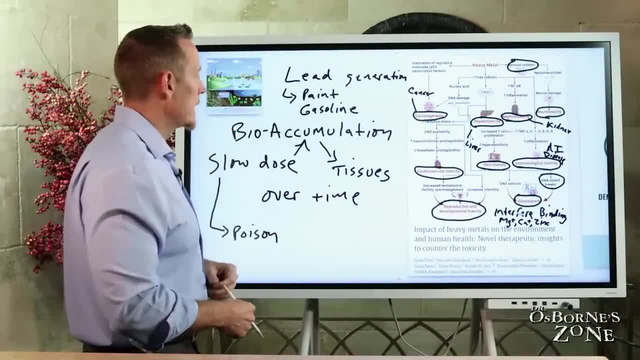 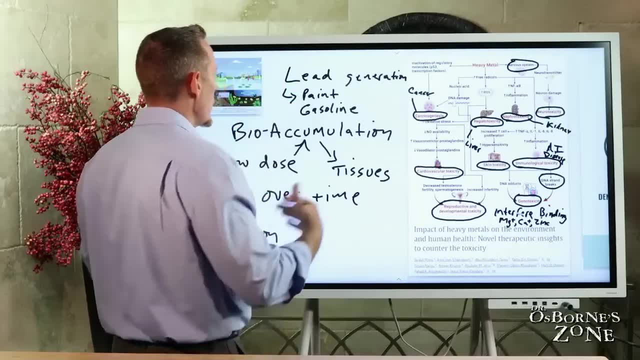 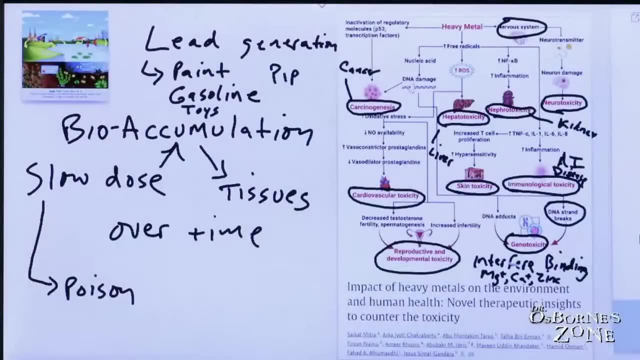 options to purchase and that's because they would put lead in the gasoline because of its it's a effect on the engine and so again, paint gasoline and he would find lady and toy was children's toys. we find laden pipes as parts in a solder for the pipes to put the pipes together. not so much lead. 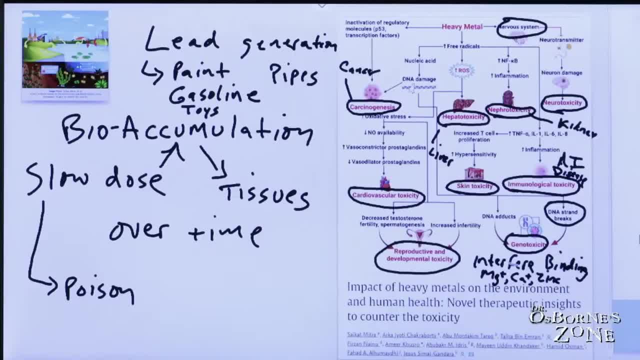 pipes per se, but the solder that held the pipes together- oftentimes it was- was a lead sensitists. so you had a lot of lead exposure in that generation and somebody honestly in saying nobody, but it was not not super common to see acute lead poisoning in somebody- lash it like a. 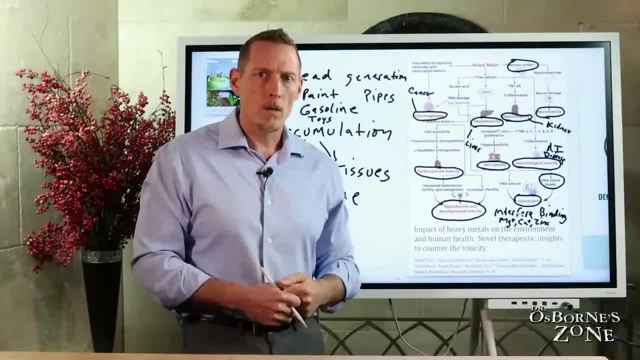 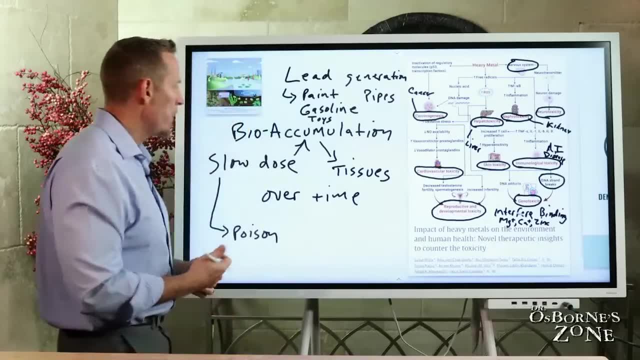 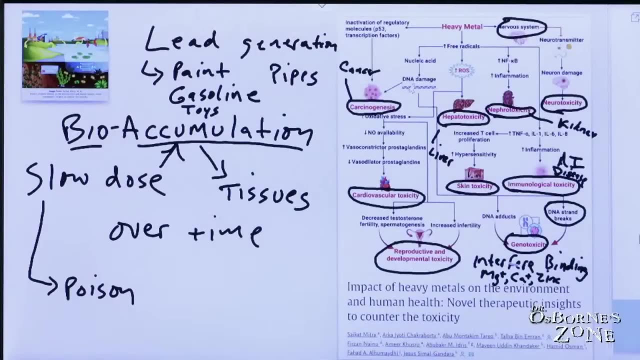 child who's eating paint off of the wall wall or chipping away at some. some painted toy then was getting really a high level of exposure and developed an acute toxicity poisoning. but the vast majority of that generation bioaccumulated the lead or bio accumulated their exposure to metal over time. so it's important to make that. 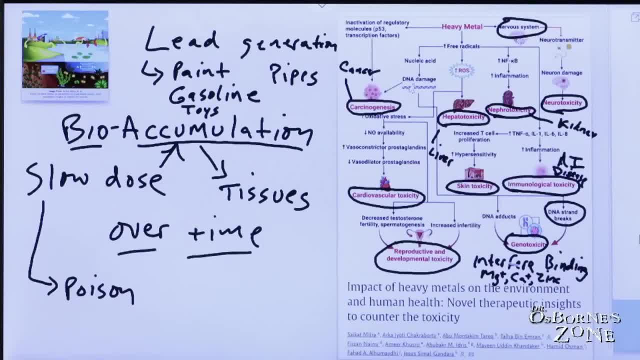 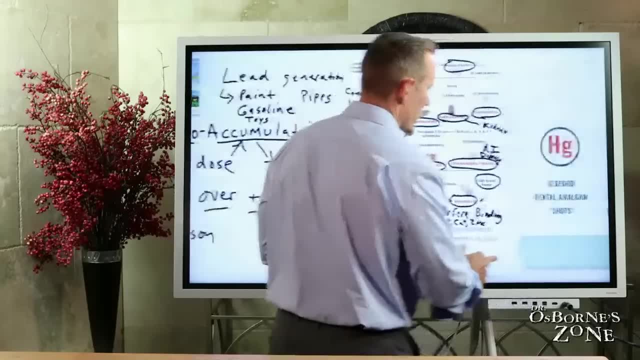 distinction, because you don't just wake up from bioaccumulation problems. this is a slow burn, it's a slow poison, so keep that in mind as we go through, as we go through, this today. so here's some of the most common toxic metals that we see. 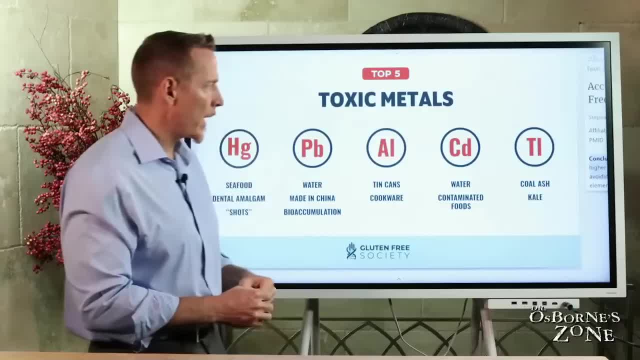 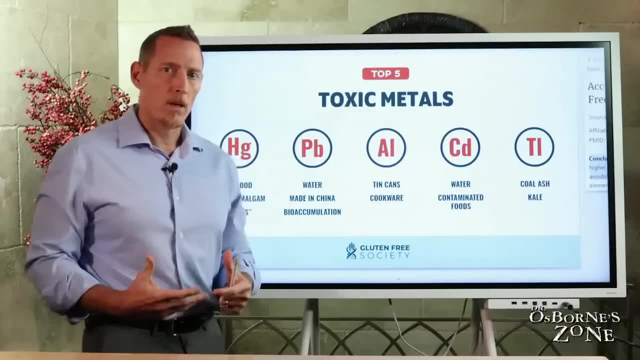 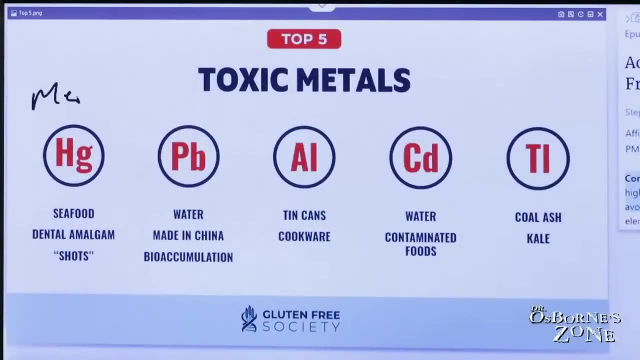 I'm not going to go through every single toxic metal, we just don't have the time or bandwidth to cover all of it, but these are some of the most common ones that I see and people that we actually test for: heavy metal exposure or heavy metal bioaccumulation, mercury- so HG is mercury and then we have lead here. PB. 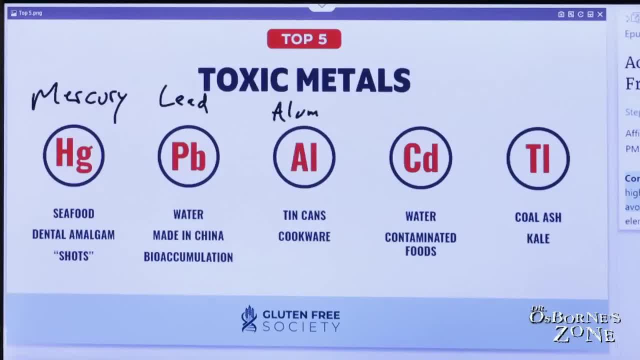 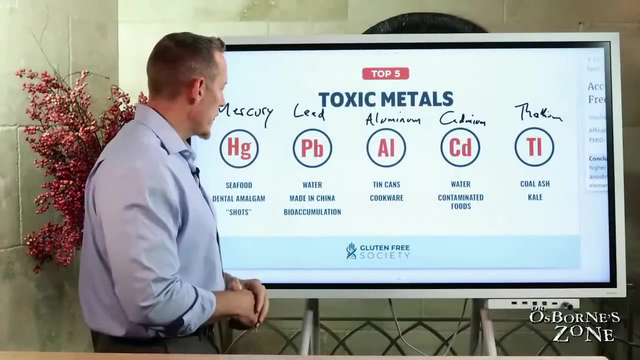 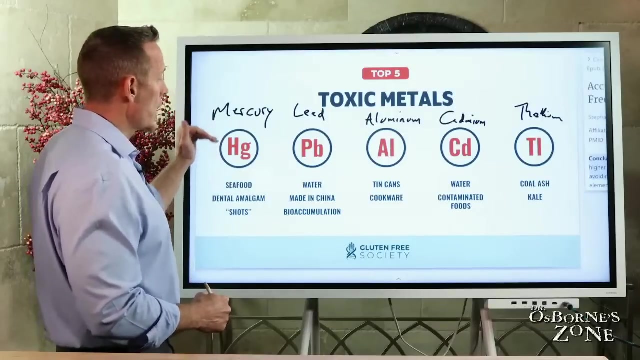 and then aluminum, cadmium and Thallium- that's an A. so these metals are some of the most common ones that we'll see and people today they come in and get actually testing done and so to give you an idea for where these exposures are commonly coming from with 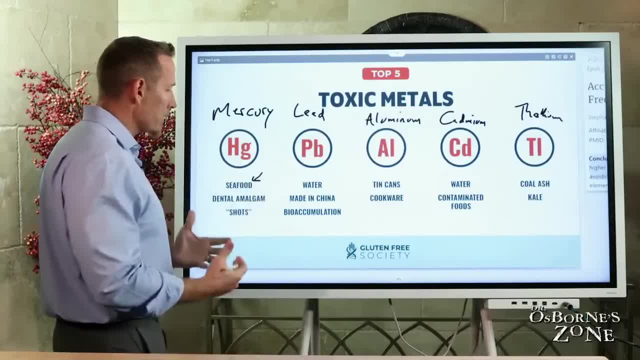 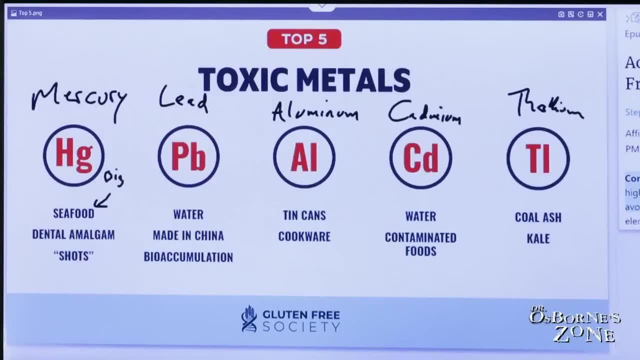 mercury, you know a lot of it is seafood and it's not all seafood. so I don't want to say don't ever eat seafood, but it's the bigger the fish, the more the potential for exposure. So the bigger the fish, the greater potential for quantity. Now some companies do mercury testing on their 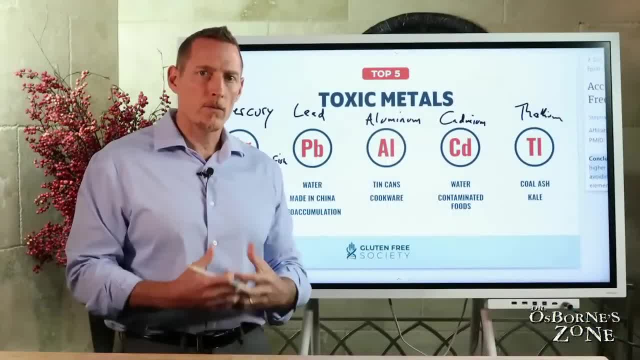 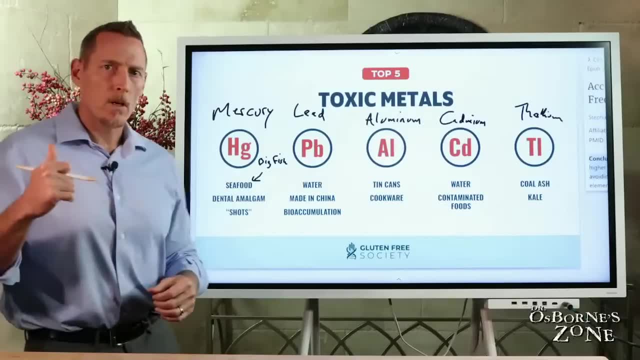 seafood and I would say, if you're in the market and you really like seafood or you're trying to follow a diet with a higher seafood quantity, go for smaller fish like anchovies and sardines. The smaller the fish, the less bioaccumulation of the metal from the, you know, from the ocean. 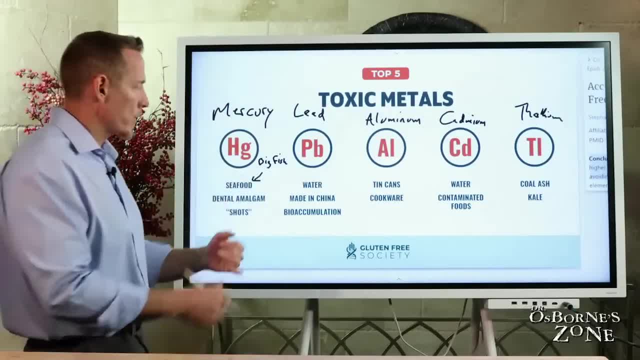 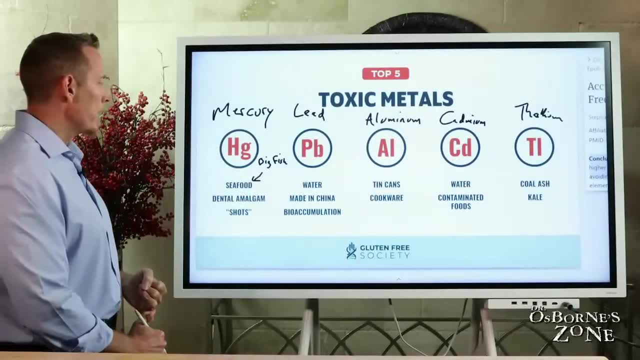 water runoff that they have. The bigger the fish, the more potential. So tuna would be a higher mercury-containing fish, salmon potentially higher in mercury, but don't necessarily need to avoid seafood per se, but just be aware again that that can be a source of exposure. 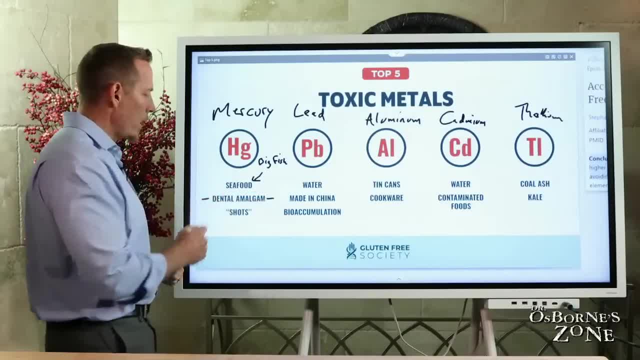 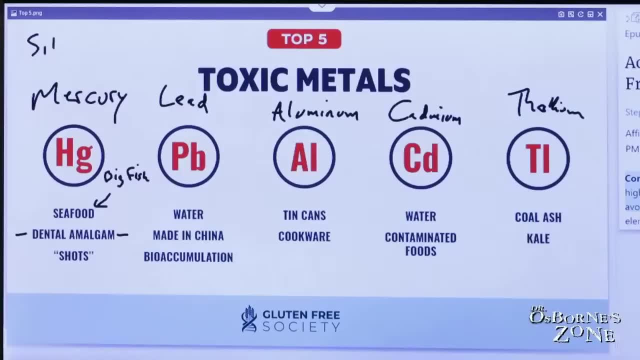 We also have dental amalgams. Now. this is becoming less true with the advancement of time, and what I mean by that is a lot of the original amalgams. the silver amalgams, or silver fillings, if you will, had mercury in them And so if you've had, you know again if you were born. 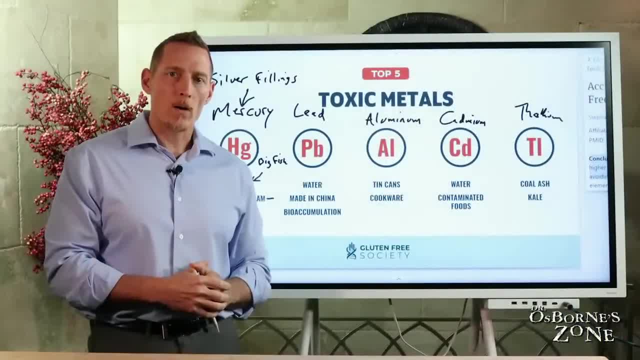 kind of 1970s or even prior, the likelihood that when you went to the dentist that your cavities would have been filled with a mercury-containing fish. that's a very, very high probability. So if you've had you know again if you were born kind of 1970s or even prior, the likelihood that 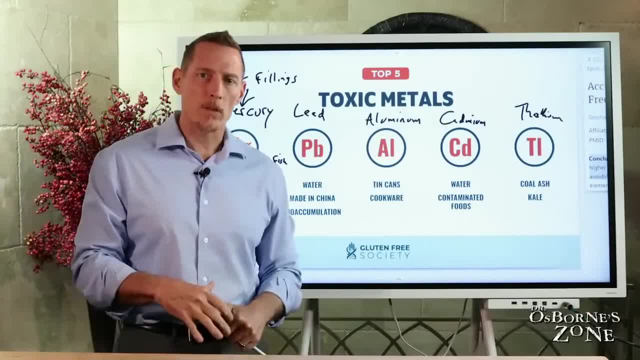 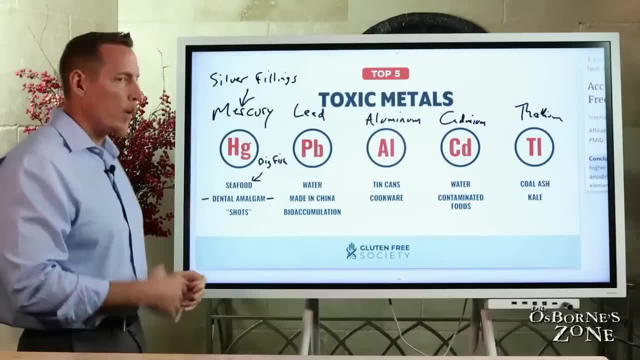 the silver filling, versus, say today, that you make them out of different types of composite materials. the likelihood that you had mercury put in your mouth is very high. So if you open your mouth- an easy way to know this- open your mouth, look in the mirror if you've got a bunch. 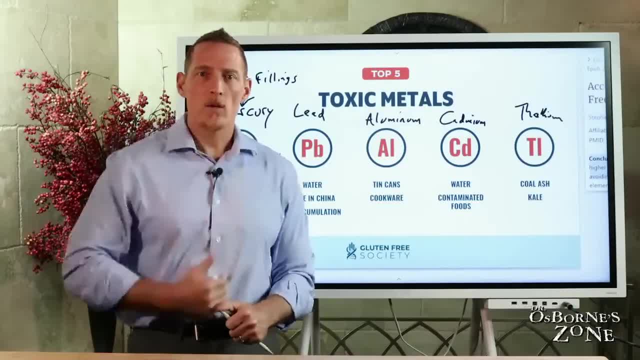 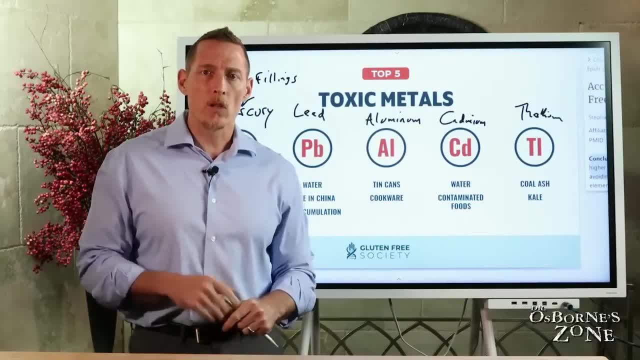 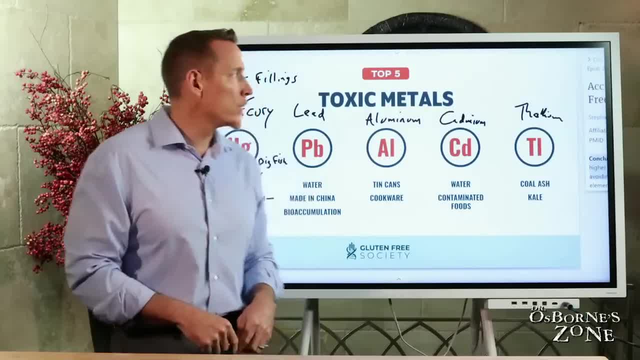 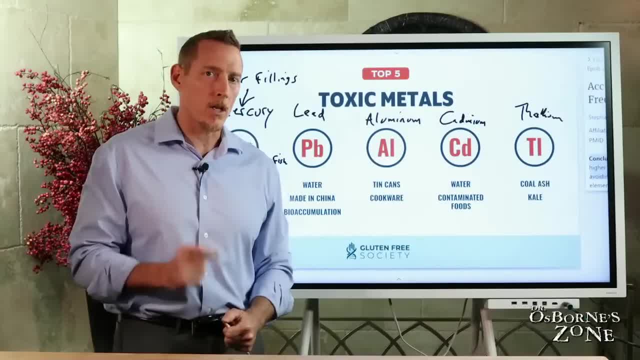 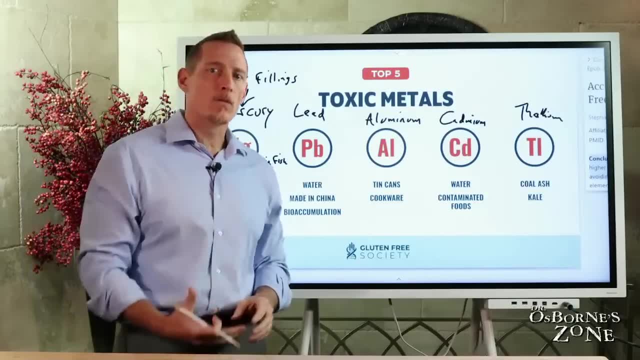 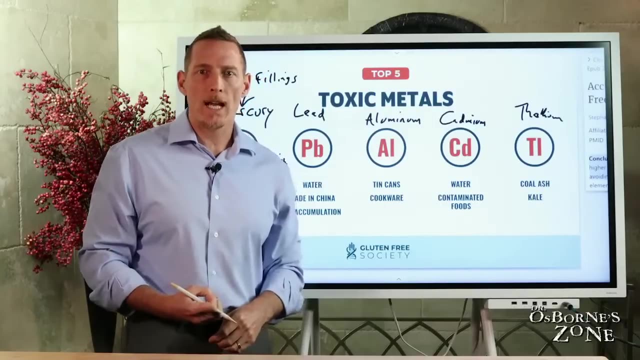 really well. So from a materials perspective, they did a fantastic job. And a lot of these fillings- even if you have them, they may be stable. I would say not every silver filling absolutely needs to be emergically or emergency-based removed tomorrow. So if you're looking at that, 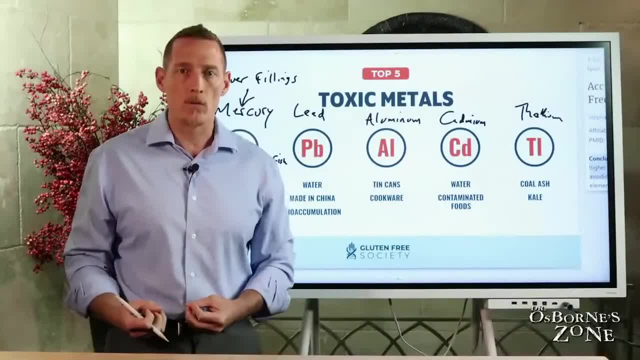 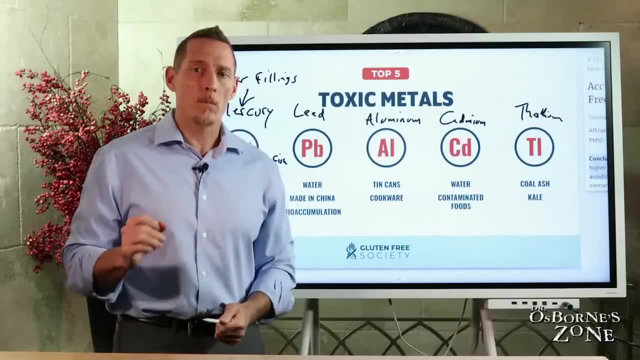 and you've got some silver fillings and you're like: should I or should I not have them, them removed? you know, my advice to anyone who's got silver fillings in their mouth is first, before you just go and remove them, test your body to make sure that mercury is even a problem for you. 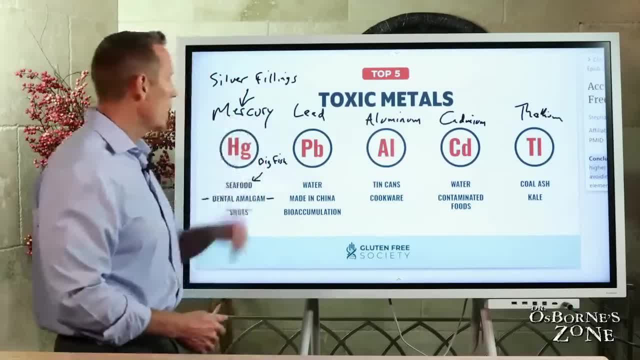 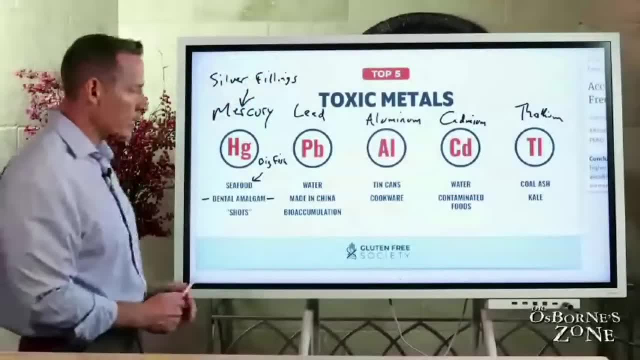 because if it's not, it may not be something that you prioritize. uh, you know, first, as a first line of something you need to go run out and can get really costly. i mean you can spend thousands of dollars having silver amalgams removed. plus, you need you know if you're going to do it. you need 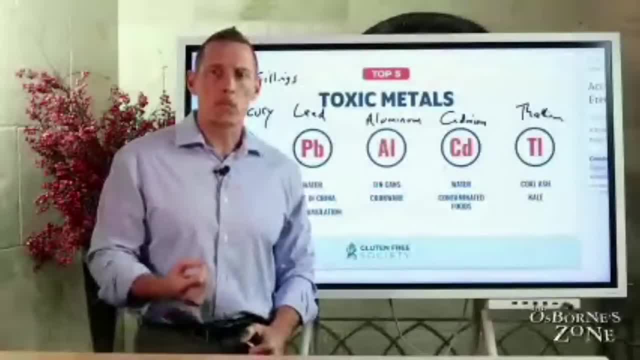 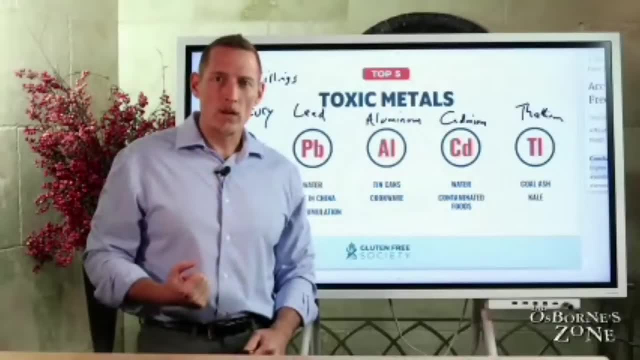 to find a good biological dentist who's well versed in the proper removal of those amalgams, because a lot of times what happens, uh, is they they pull you know, they pull them out but they don't protect you as they're pulling them out. remember, silver amalgams can be, are caustic and 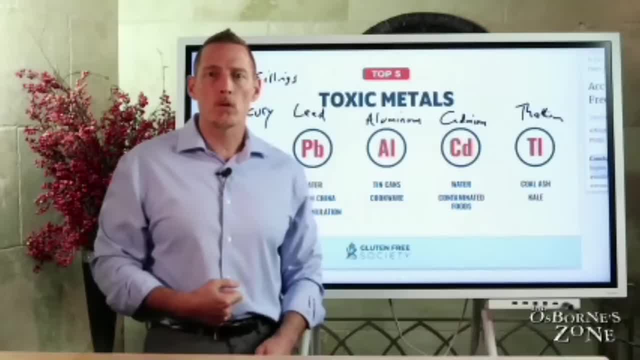 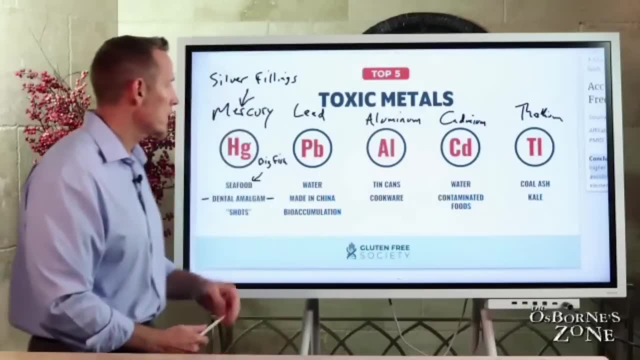 so once they break into them and crack them open, you can now be exposed to you know or swallow- accidentally- swallow a bolt- a bulk dose of mercury and that can make you sick. i've actually seen this happen to people where they worked with the dentist who didn't protect them properly. 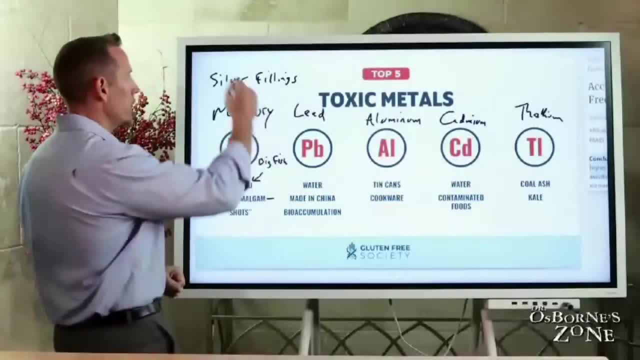 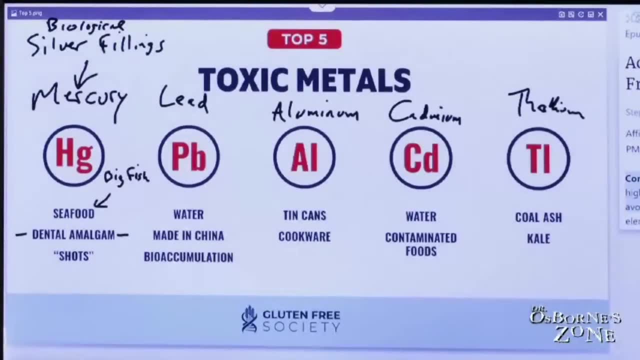 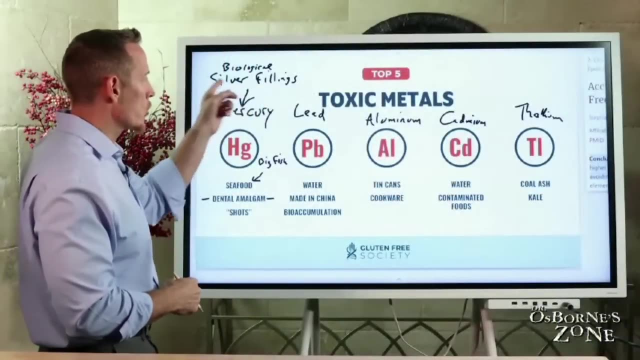 during the removal. so make sure you work with a biological dentist if you're gonna go and get these removed. um, or at the very least, work with the dentist, even if they're not registered, uh, with biological dentist associations, make sure they had a special training to properly remove. 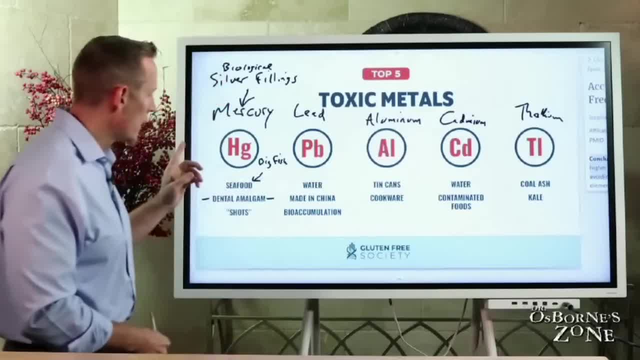 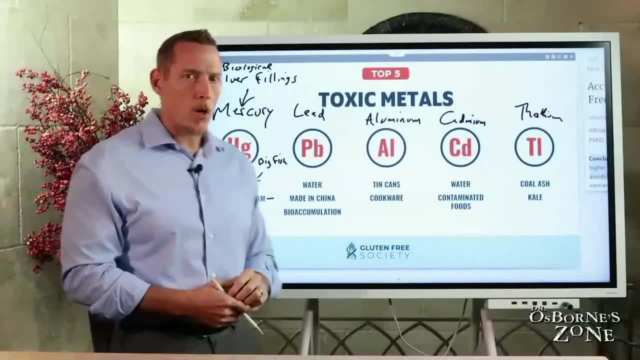 or safely remove mercury amalgams or silver amalgams, then the other place that we get it is shots. now this has somewhat changed, um, in the past few years where mercury used to be a, used to be in, like the, the flu shots, uh, that were given, and and a number of others, mmr and some of 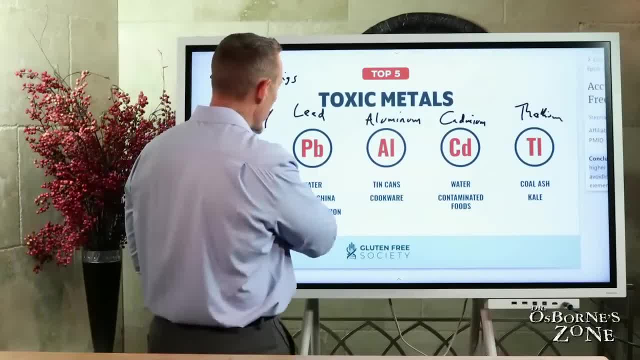 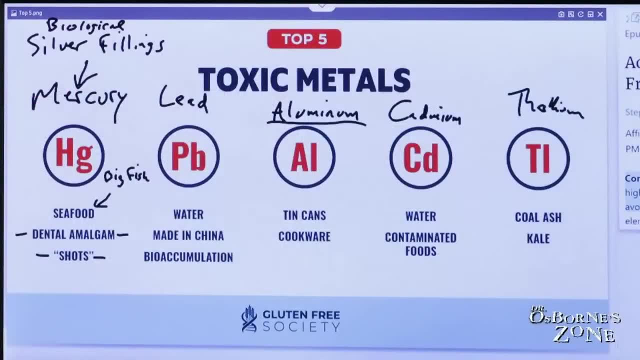 the others. but they've gone and replaced a lot of the shots that used to contain uh, mercury, and and then they've gone and replaced some of that with aluminum. so now you know that you you can check the inactive ingredient list on any of these and kind of see which ones contain. but just be be aware. 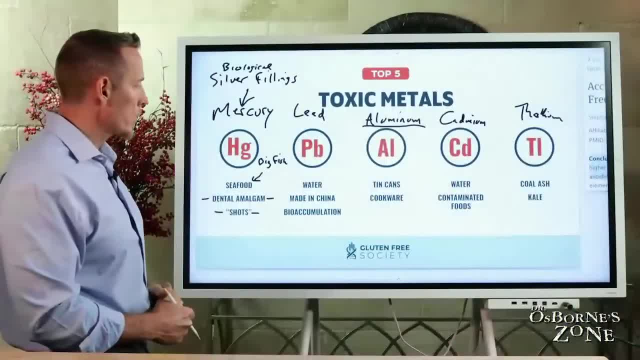 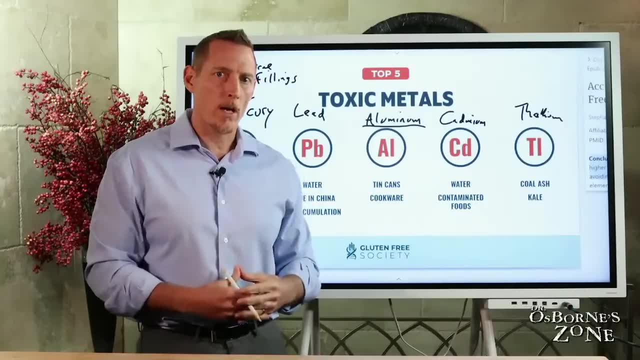 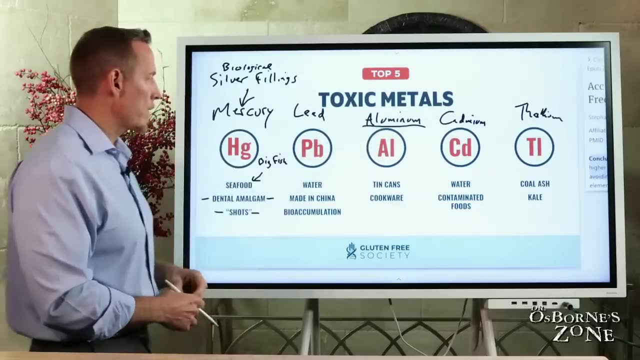 this is another one of the places where people get exposure. it's one of the reasons why, um, right now we're starting to question a lot of, you know, a lot of those generalized recommendations that have been put in place over the years, because, you know, this is actually one of the reasons are these: 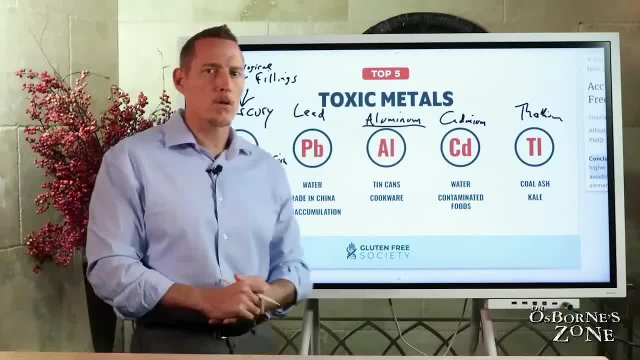 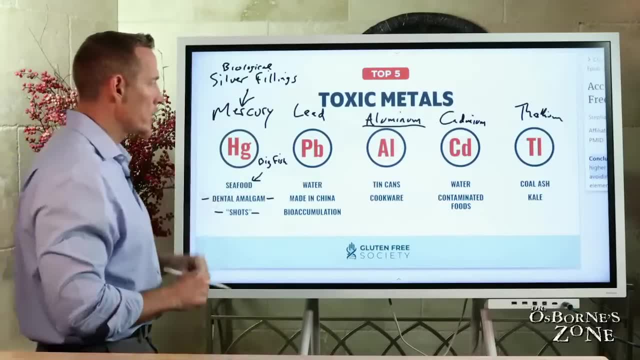 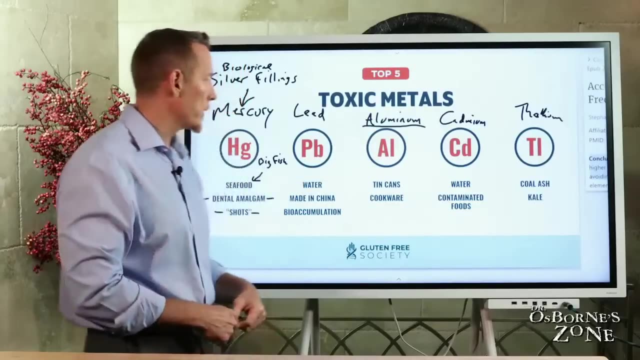 these heavy metal contaminants that are actually used on purpose and those are used as adjuvant agents to help stimulate the immune system, and so, again, many people, especially genetically susceptible individuals, can overreact to some of these, and this is why you can see some people getting injured. not everyone does, but many people. 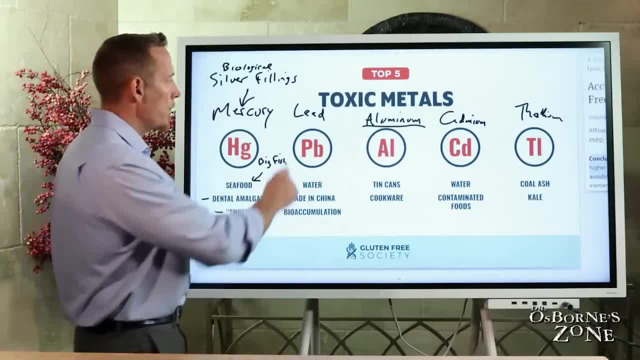 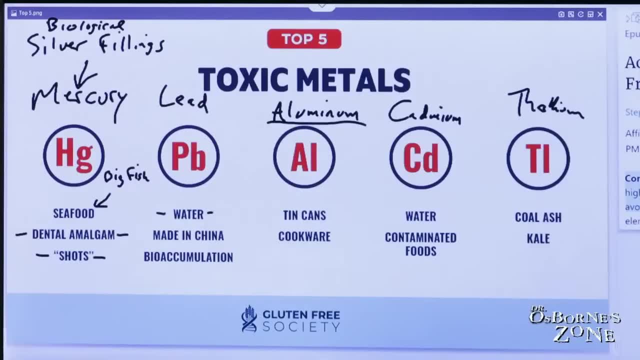 have been exposed to heavy metal contaminants over the years as a result of heavy metal contaminants. and then we have lead- lead. you know where do most people get their exposure today? predominantly water, and this is like the city water supply, depending on the age of the city's infrastructure, where 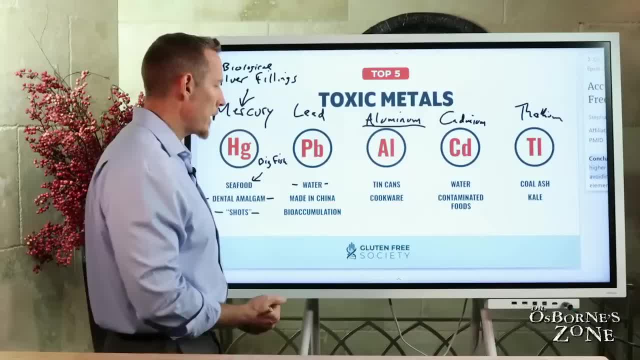 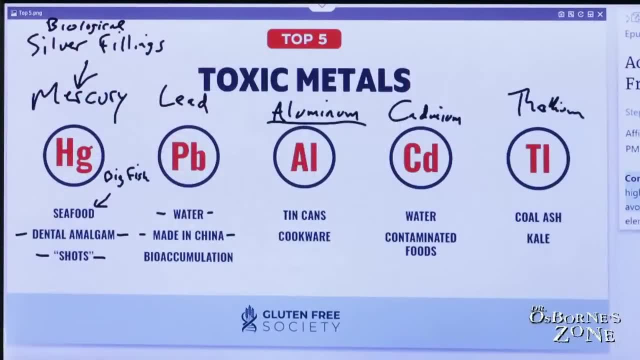 you're at again. i use flint michigan as the example there of a of an infrastructure that was lead contaminated. we also see, you know a lot of things that are made in china, and this is not just like pots, pans, cups and and other things. this could also be food. so we've got a lot of things that. 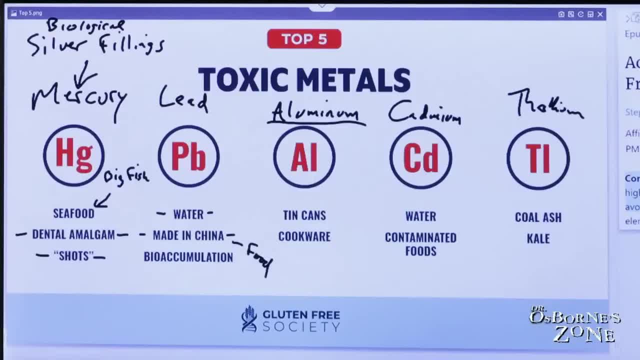 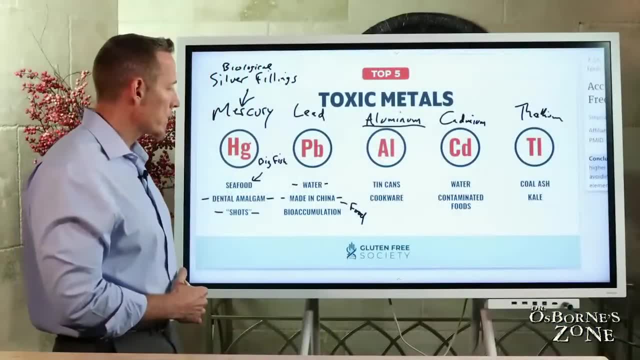 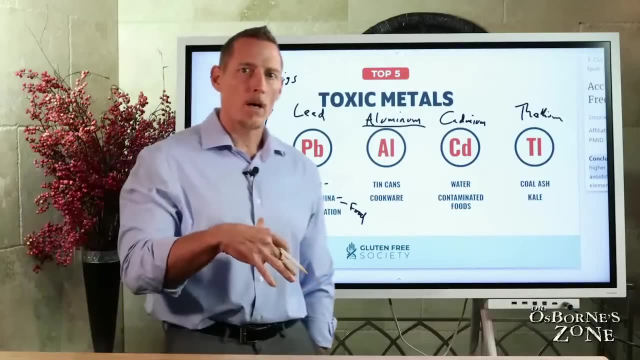 are made in china. so food, you know, food products, baby formula, perfect example. we've seen recalls of lead and baby cereals recalls because of lead toxicity or lead of an abundance of lead. so beware, made in china. you want to be really cautious because there's a reason why a lot of, uh, a lot. 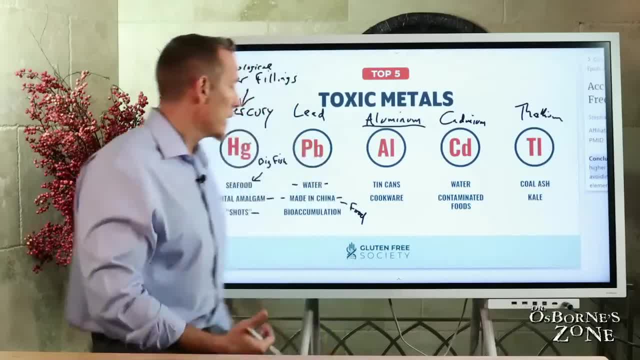 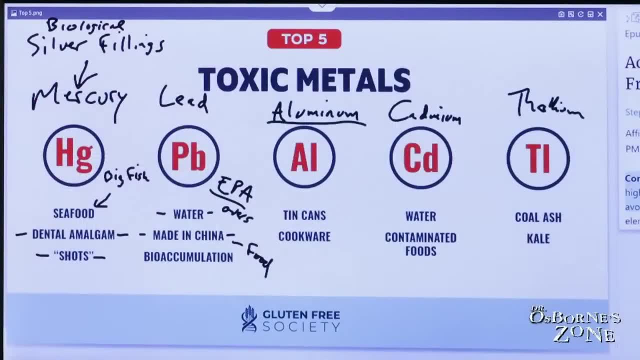 of companies have outsourced their businesses overseas. it's because there's less epa oversight. you know when you, when you go and do business where there's less oversight and you can import those products back into the country. there's just not the same oversight that you would have if those people had their factories over here. so a lot of companies skirt the oversight. 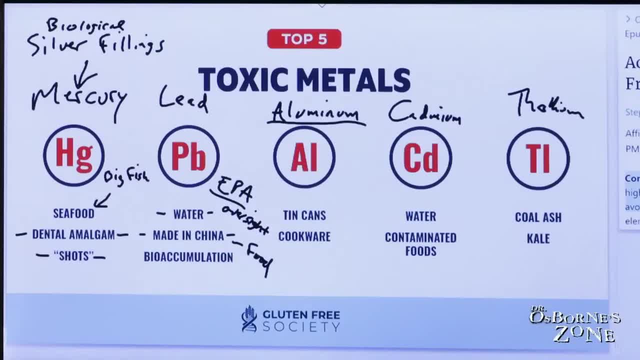 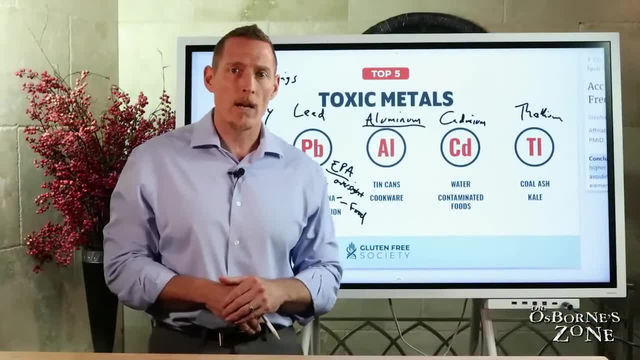 produce in china and bring back cheaper products that are contaminated with metal. so i'm you know. my advice is: if you're you know, if you're looking at food, don't buy made in china. if you're looking at pots and pans and other things that have the potential to be contaminated with, 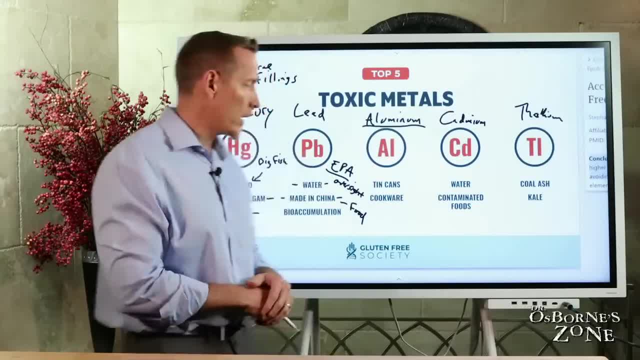 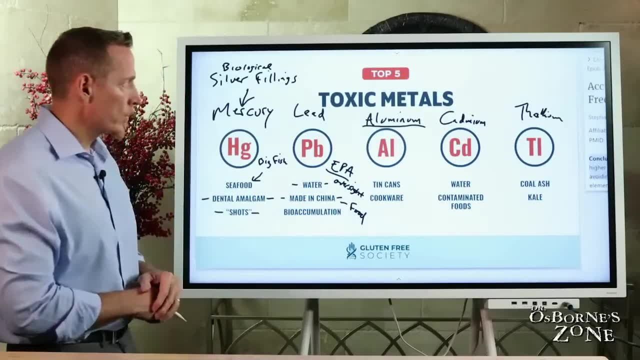 metal. you know it's better off by us, by american made or by european made, but but avoid, in my opinion. avoid this if you want to avoid lead. and then the last reason why we'll see lead, you know very common, has to do with the bioaccumulation, and i was talking about this. 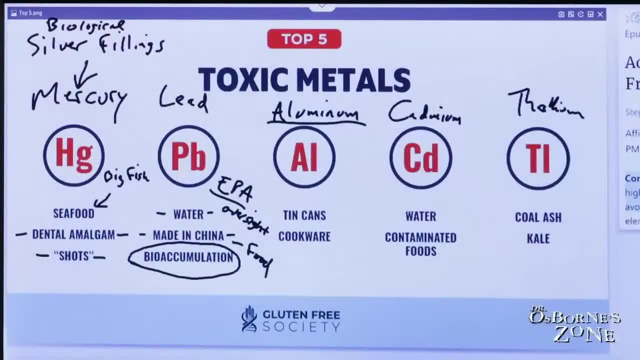 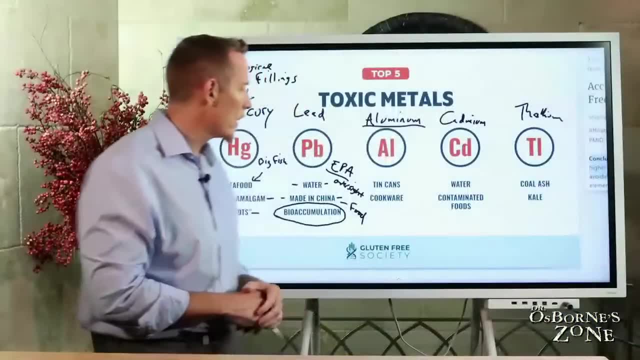 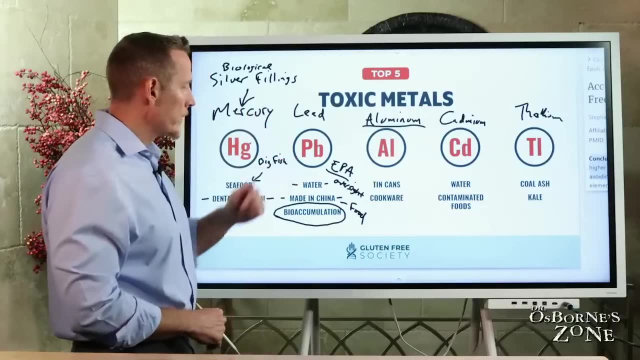 a moment ago. this is the chronic exposure of low doses of lead because historically as a nation we've used it in paints and gasoline and other as additives and other things, and so we've got this bioaccumulation that's occurred. i think it's important to say, too, that lead is one of the heavy 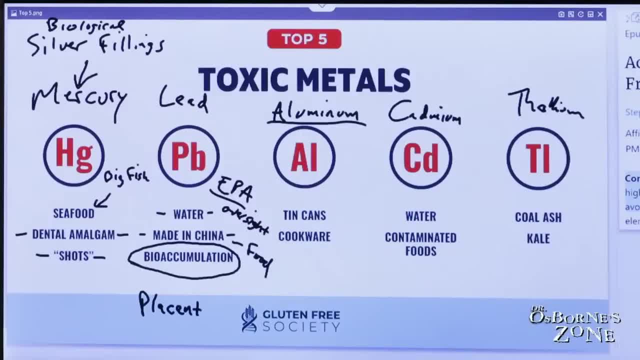 so if you are a pregnant mother and you are being exposed to lead, your baby is then going to be exposed to that lead, because lead can cross the placenta and and it can make your baby exposed and that can then start to accumulate even in utero in your baby. so you want to be aware and you want 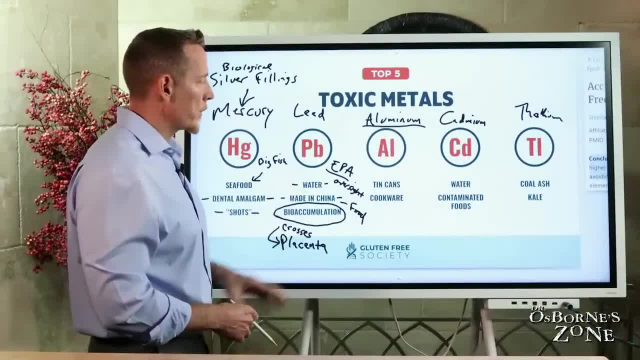 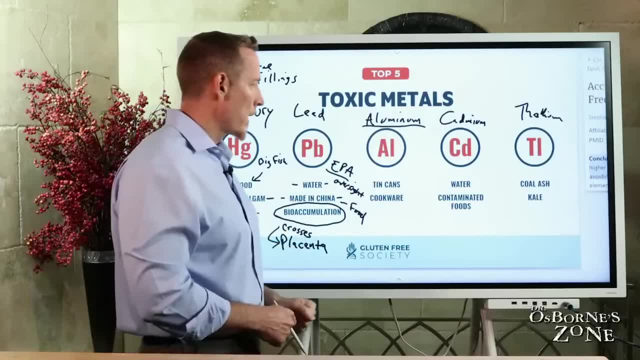 to be cautious, that you're doing everything you can to avoid exposure during pregnancy, ladies. and Again, it crosses the placenta, so you got to watch out. And then we have aluminum, And aluminum is used. I mean, the classic is foil right. 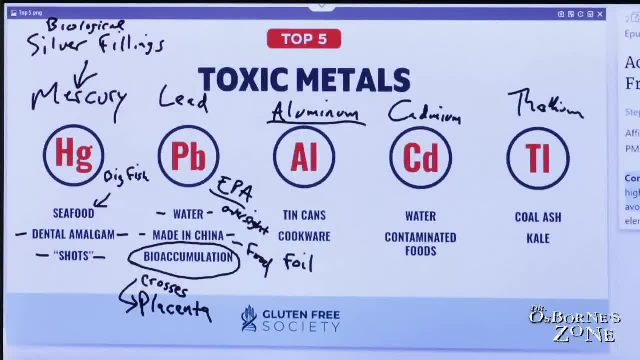 So aluminum foil a lot of people use to cook or bake with, but you also have tin cans and other forms of cookware that are aluminum-based, And so, again, high-quality cast iron, high-quality stainless steel would be better options. 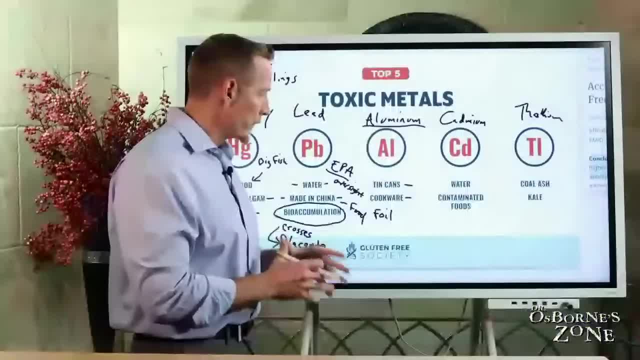 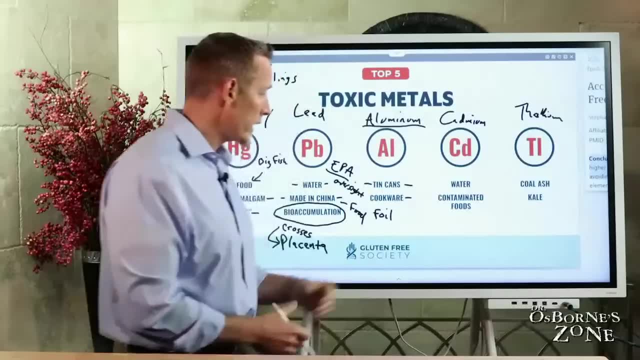 in my opinion, if we're talking about aluminum-free types of cookware, Again, don't drink out of tin cans. I mean, a lot of people do, I don't. I don't recommend it. Try to avoid that and try to avoid having your food cooked directly on the foil. 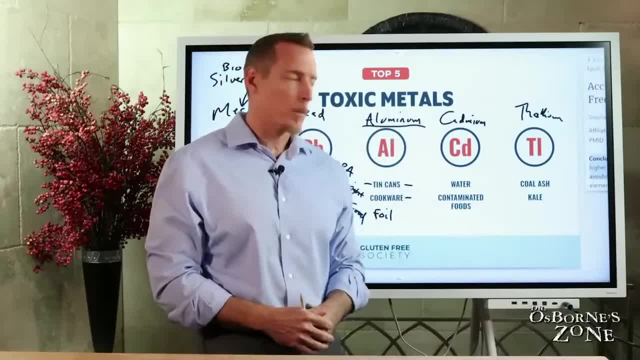 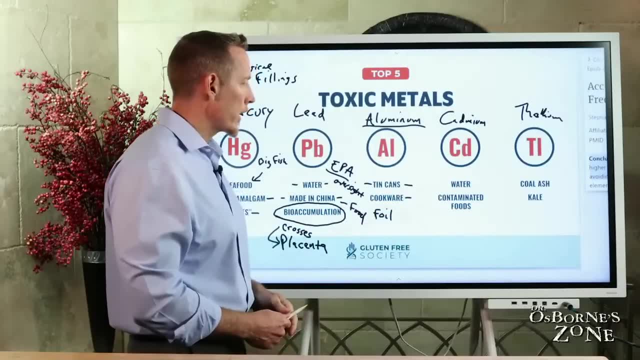 If you're wrapping a lid with foil and it's not actually touching or permeating your food, you're probably better off or okay. but cooking directly on the foil, I would be cautious about that for that exposure to aluminum. So we have cadmium. 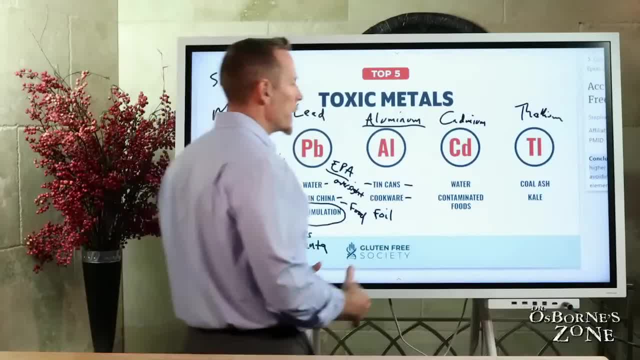 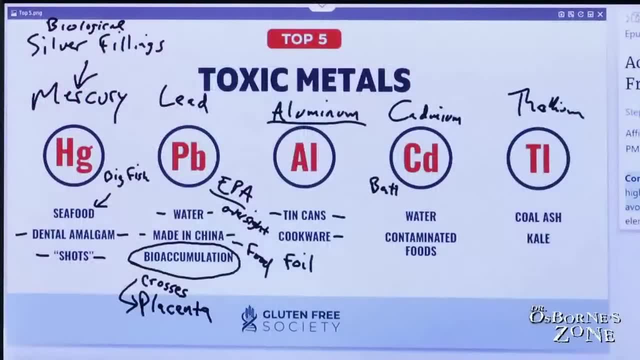 Cadmium, oftentimes found in the water. A lot of the batteries being produced today are cadmium-based, The DICAD batteries, And so those end up, those batteries. they bury them, They put them in the ground, and where do they end up? 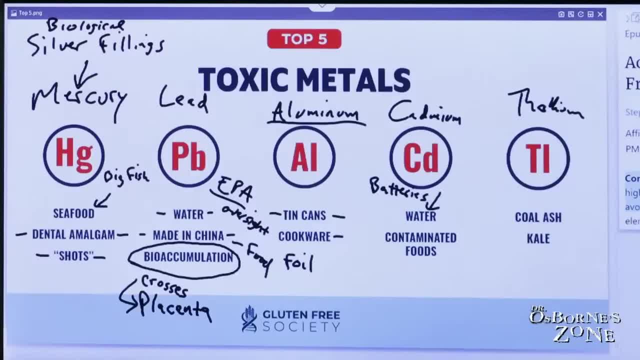 They end up in groundwater as well as soil as they break down. We also see a lot of cadmium in contaminated foods. It's a big one that we see Cadmium. also found a lot of it if you're a smoker. this is a good reason to add smoking cessation to your resolution list of improving your health, but smoking can increase you to massive quantities of cadmium over your lifetime or cadmium contamination. So what foods are richest or highest in cadmium? potential problems It would be rice. 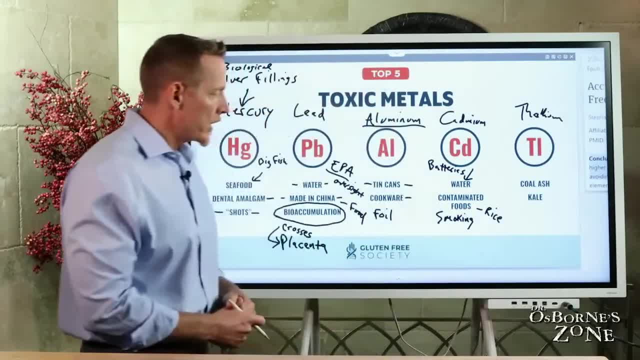 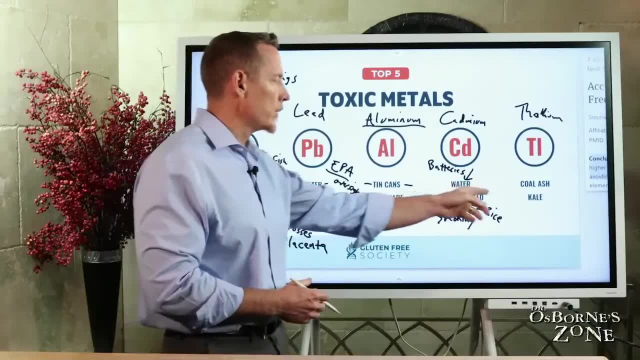 And this is one of the reasons why, you know, when I wrote No Grain, No Pain, heavy metals was one of the reasons to avoid all grains, not just wheat, barley and rye, because you know a lot of your foods that are high. 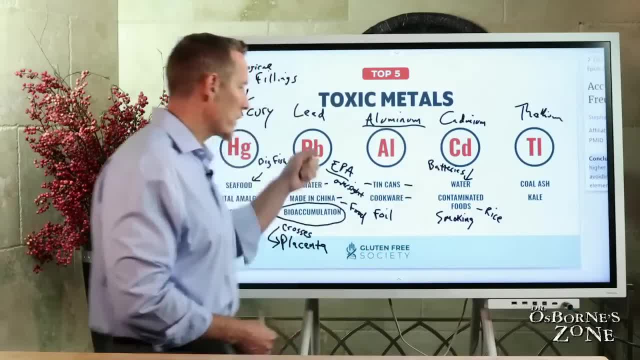 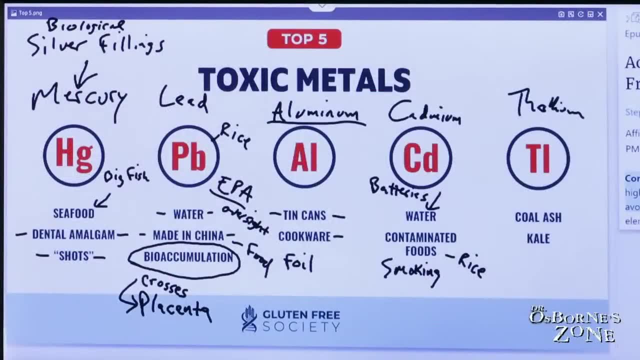 or a lot of your rice-based foods, I should say, are high in cadmium, also high in lead We get. rice can be contaminated also with arsenic, which is not on this top five, But we could put it as a bonus. 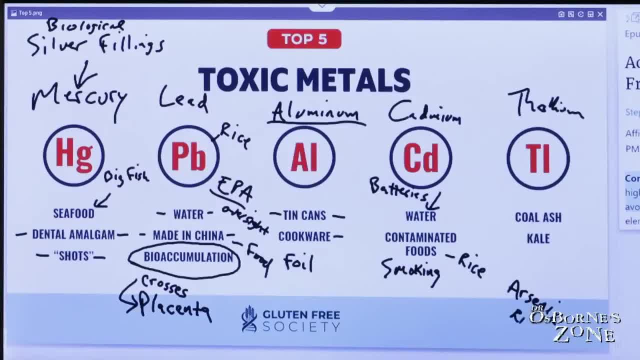 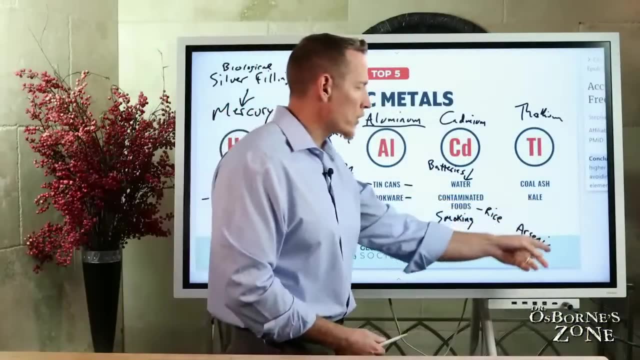 We could put arsenic on here and we could also say, you know, rice being one of the biggest sources of chronic bioaccumulative exposure, because a lot of arsenic is used to make pesticides which then end up in the soil, And so then when we're growing those foods, you know we're getting exposure to that. 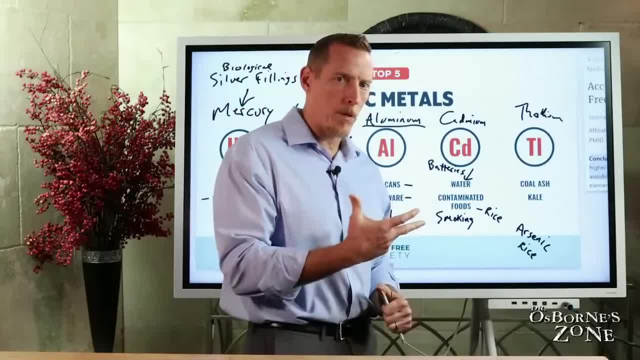 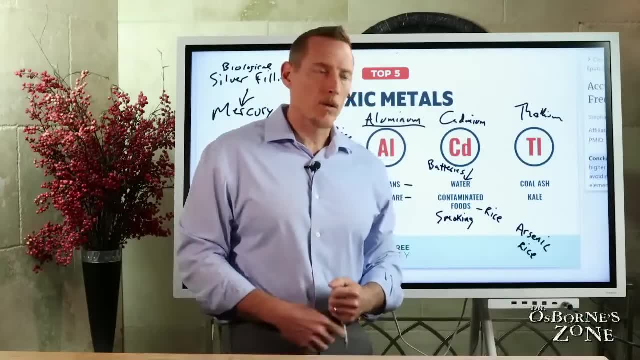 because those foods, especially rice, is really good at this. It pulls arsenic and cadmium and lead out of the soil into itself And then when we go to eat those things as staple foods and feed our babies- you know rice cereals and other things- 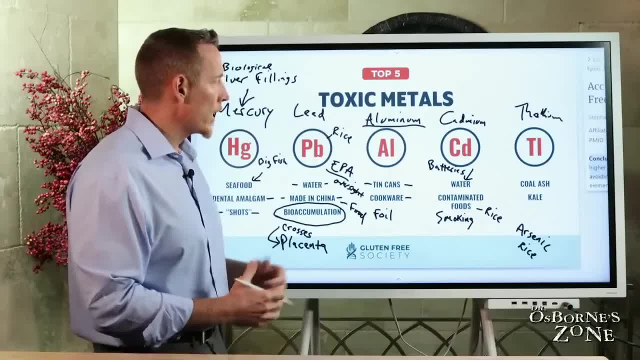 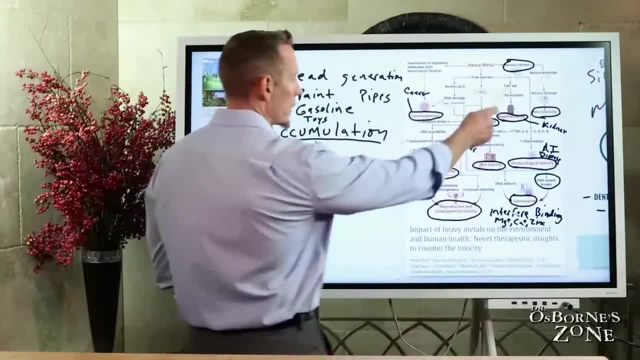 we're exposing them to high levels of these compounds early in life And that's no good because- remember what we say earlier- the impact and the effect is multisystemic: right Nervous system, kidneys, liver, potential for cancer, heart, skin immune system. 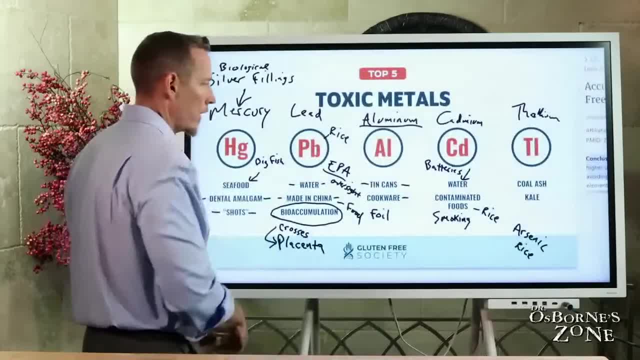 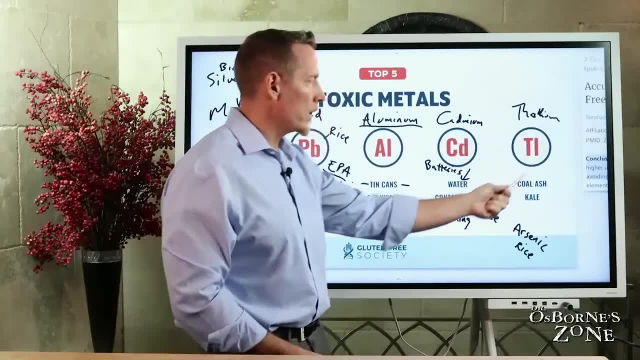 genetic issues- all can you know- can occur. So obviously you don't want your babies being exposed to high levels of these contaminated foods, And the last one over here on the right is thallium, And thallium is a toxic metal. 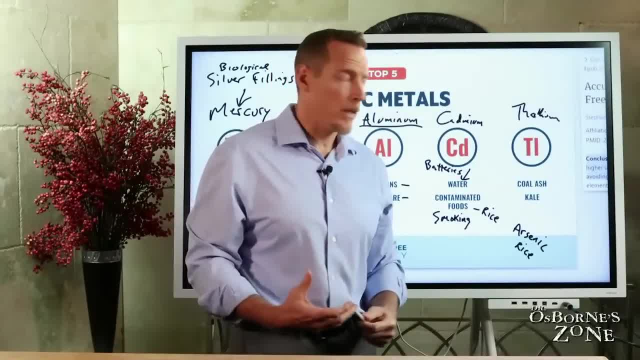 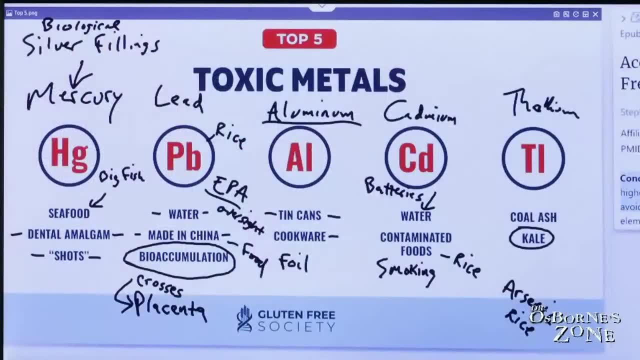 A lot of where we get today's exposure- where I see it, at least clinically speaking- is people. that- and again, I'm not picking on you if you are following a plant-based diet or a vegetarian diet, but where do we get a lot of kale from environmentally? 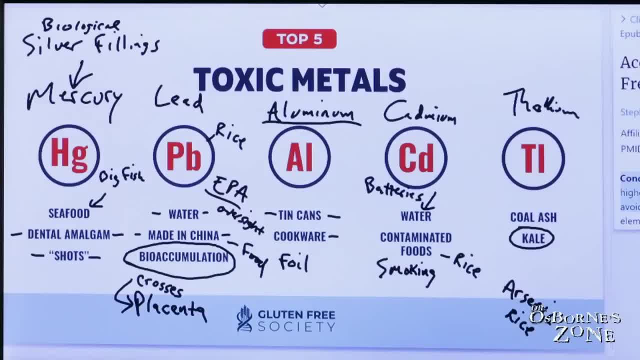 or not kale. where do we get a lot of thallium from? environmentally, It's from kale. You know, kale's a superfood. We always hear that Kale's this really, really healthy food that you should eat a lot. 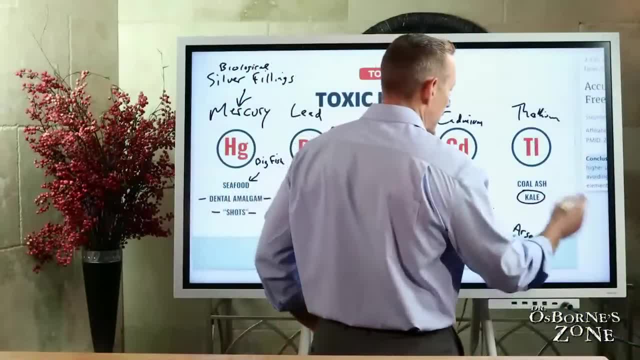 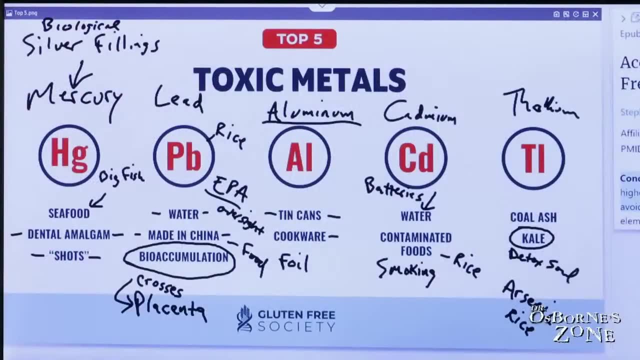 Well, the problem that we're finding is that kale is super at detoxing the soil. Kale can detox soil very well, And so one of the things that we find in soil is thallium. because of this right here, because of the coal ash- 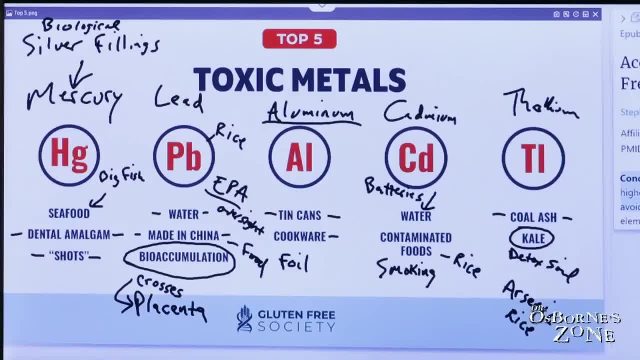 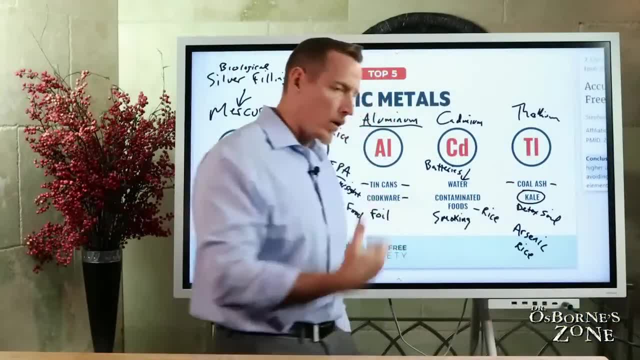 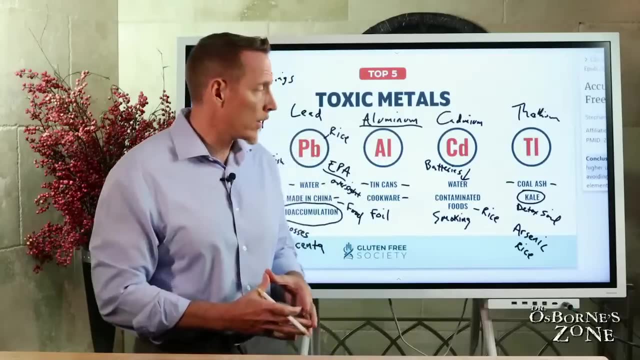 One of the things that happens in the organic farming industry is they actually take a lot of coal ash, which is a byproduct of burning coal, as fuel And they sell that to the organic farming industry and they use that as a soil amendment. 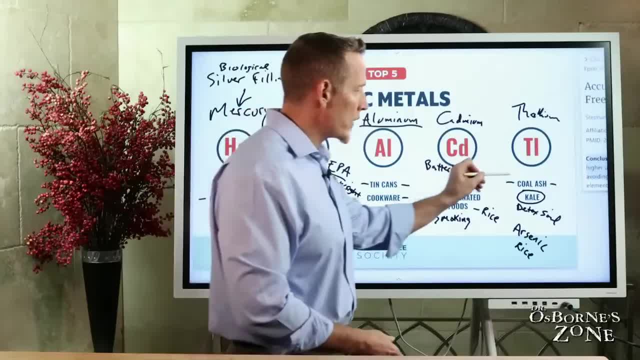 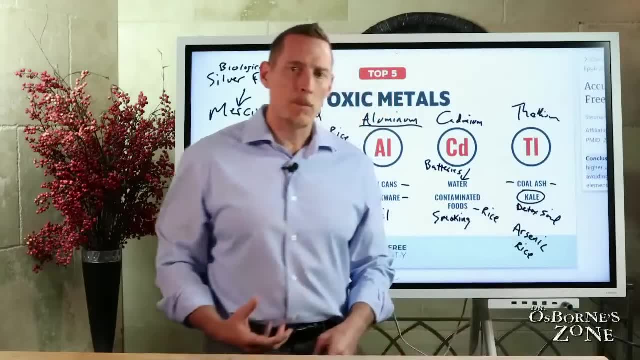 if you will, to improve the soil. But it comes that burn off comes with a lot of thallium. So you end up with thallium in that soil And if you're growing your organic kale in that particular soil, that kale super detoxifies the soil, pulls the thallium into it. 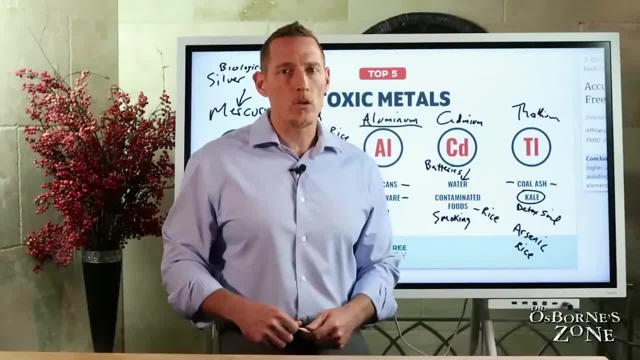 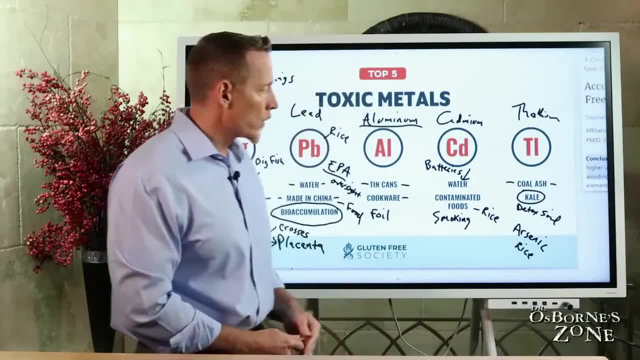 So if you're doing heavy kale consumption- and I see this a lot in juicers- not just plant-based diet folks, but people who do a ton, a ton of juicing where they're using kale as a primary source of that green juice- 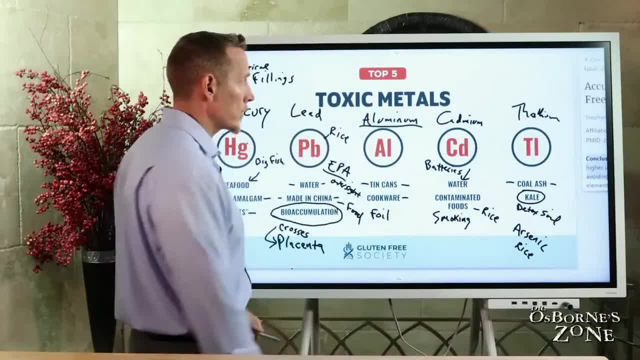 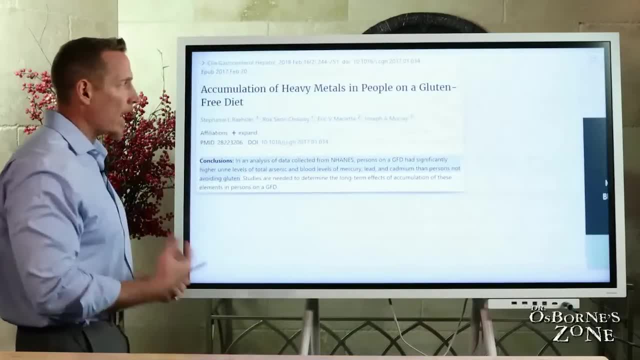 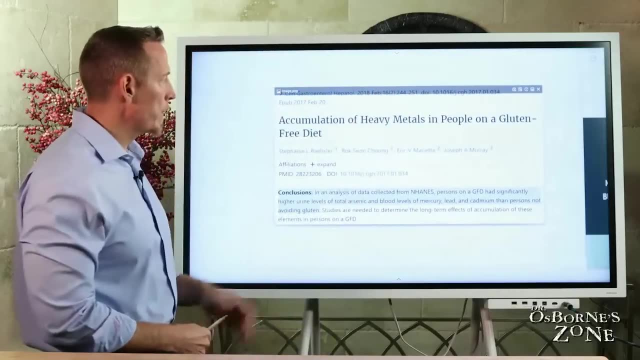 But we're seeing them come back super high in thallium and it can make you sick, So be careful. Now, one of the other places that we see people having higher risks of heavy metals is people following gluten-free diets, And I put this up here. 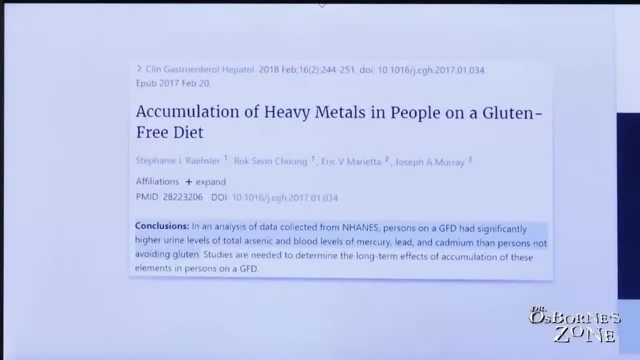 This was a review paper published in Clinicscom Clinics in Gastroenterology and Hepatology, And so what you can see, the title: Accumulation of Heavy Metals in People on a Gluten-Free Diet, And so, with this data, 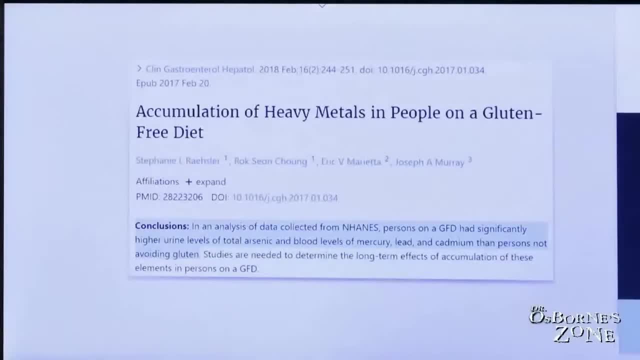 with this. data identified is that people following a gluten-free diet had significant higher urine levels of total. So again, what's key here? because a lot of studies are what we call epidemiological studies, And epidemiological studies are like: oftentimes they're popularized. 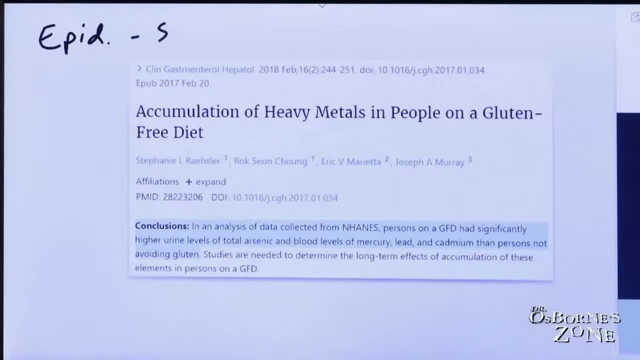 They're population-based surveys, So there's surveys a lot of times where they're asking people about things. This study was not a survey. It was actually an analysis where they measured output of the urine, So this is actually testing. They have found higher levels of arsenic and then blood. 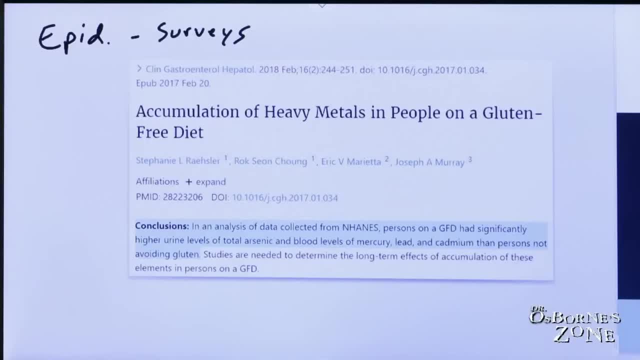 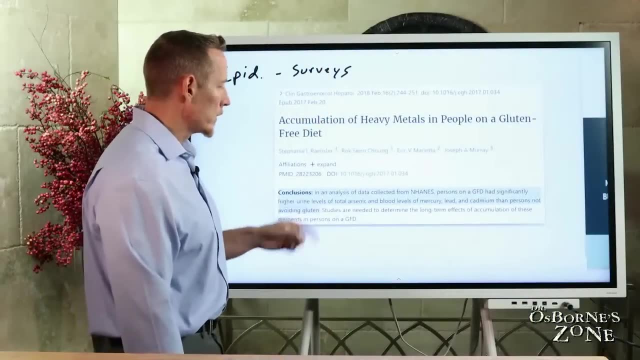 higher level of urine arsenic, So urine arsenic coming out in the urine, and then higher levels of blood mercury, lead and cadmium than persons not avoiding gluten. So why is that? Why is this happening? I can tell you what we suspect. 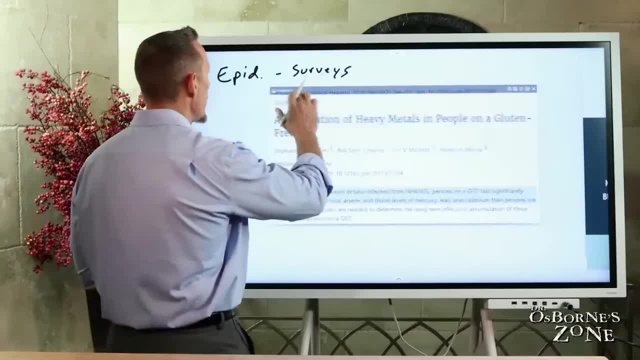 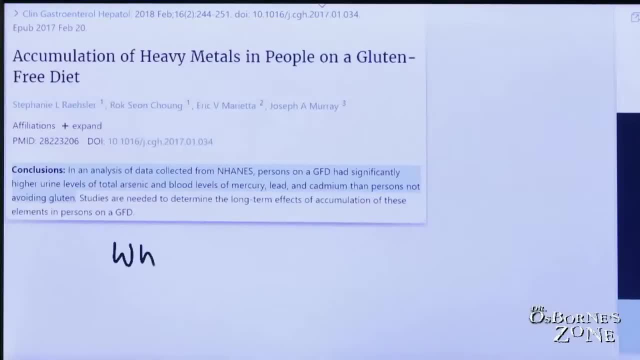 These authors didn't go on to conclusively say why people following a gluten-free diet are exposed to more of these heavy metals, But the biggest reasons are- and we found this to be true- is that wheat has higher wheat, as a food has higher levels of. 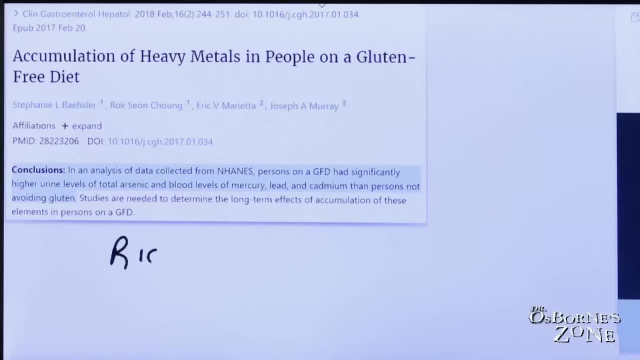 I'm sorry, not wheat rice, as a food has higher levels of arsenic, of lead and of cadmium, And so a lot of people following a gluten-free diet. what do they do? They gravitate toward this high consumption of rice. 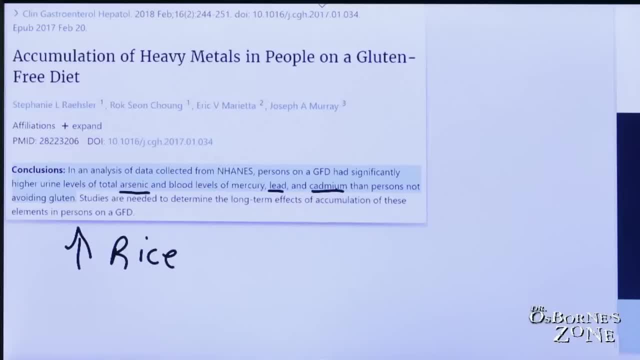 because it's one of their favorite substitutes to make breads, pastas, cakes and do baking with is rice, And then the other one is corn. They increase their corn, And so what they've identified with corn and corn byproducts is more mercury exposure. 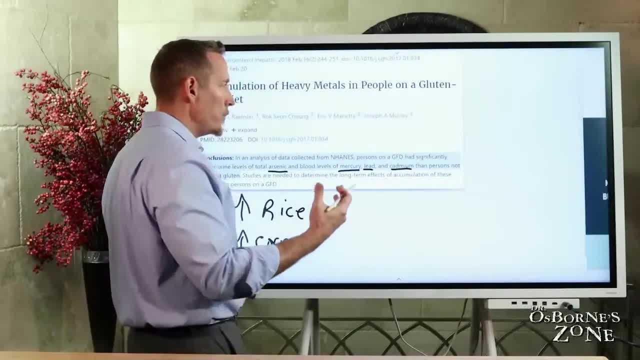 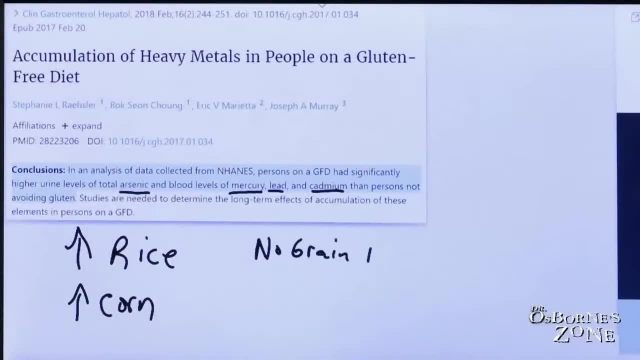 toxic heavy metals. and this is just one more reason why you probably heard me differentiate. you know, when i say no grain, no pain, the title of my book, it's not. the title wasn't no gluten, no pain. it was no grain, no pain. and this is one of the reasons why is the contamination of corn. 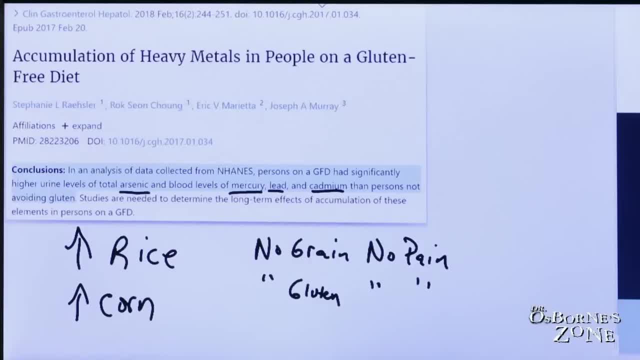 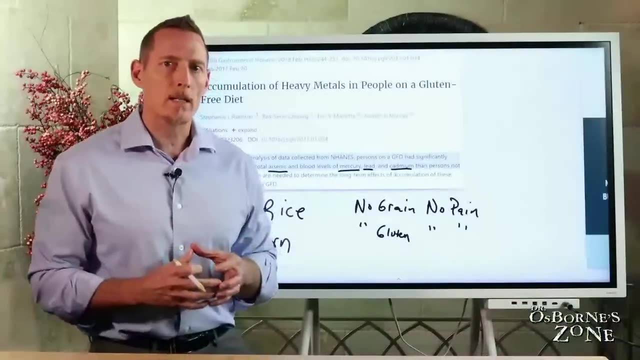 and rice with high levels of heavy metals that bioaccumulate in the tissues, leading to kidney and liver and heart and skin and all other types of potential damage. a lot of the symptoms, unfortunately, of celiac, like classic celiac disease where you have the gi tract inflammation and we've got increases of inflammation. 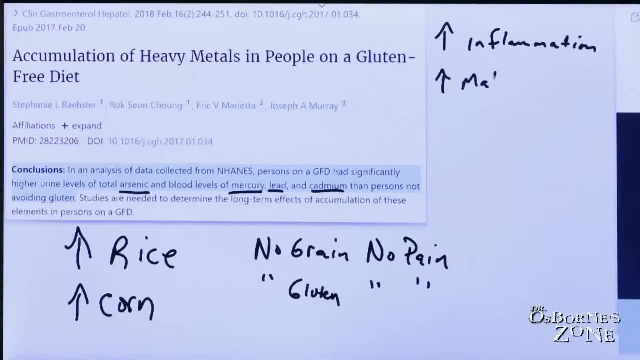 you can have increase malabsorption. so vitamin, mineral deficiencies and the problem- one of the biggest problems with with somebody who's got like a gluten sensitivity- not just celiac but also non-celiac gluten sensitive individuals- is these are very big problems for them and what happens is this malabsorption will affect. 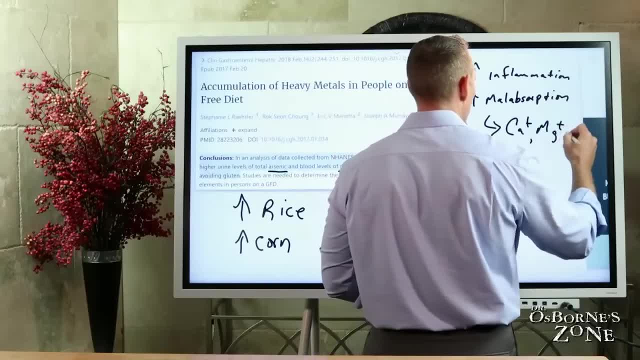 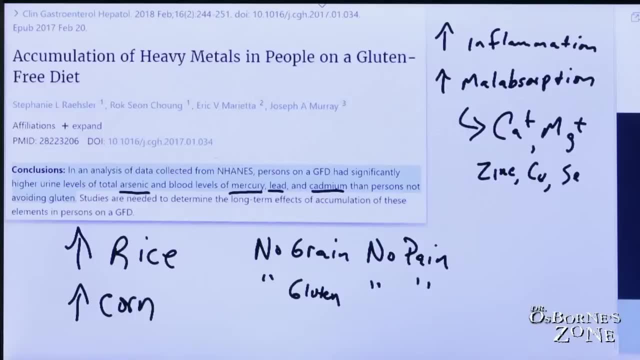 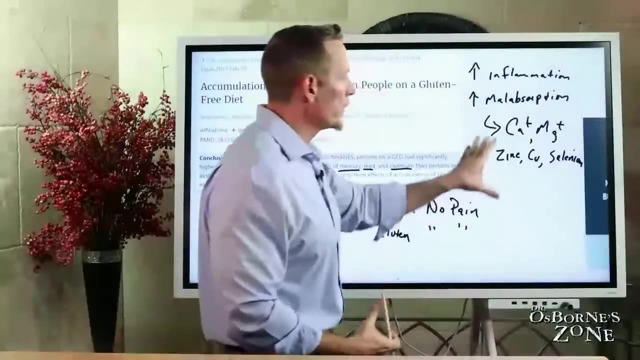 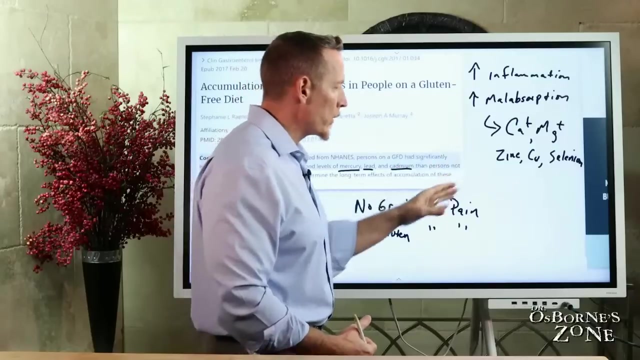 things like calcium and magnesium and zinc and copper and selenium. these are all very important minerals and what's been shown in research is that when people develop or when people have deficiencies of these particular minerals, then if they are exposed to heavy metals like mercury, lead, cadmium and arsenic, then these metals will 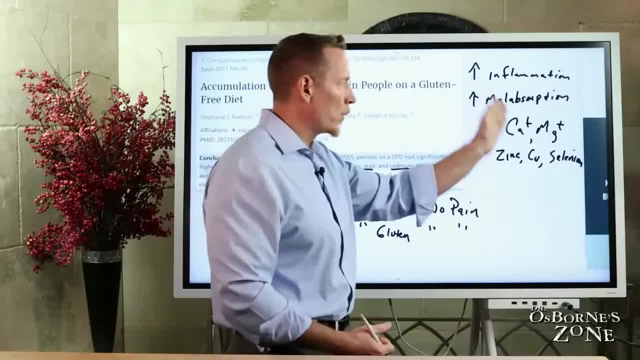 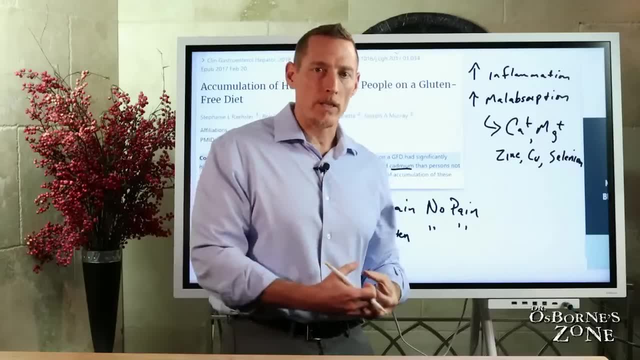 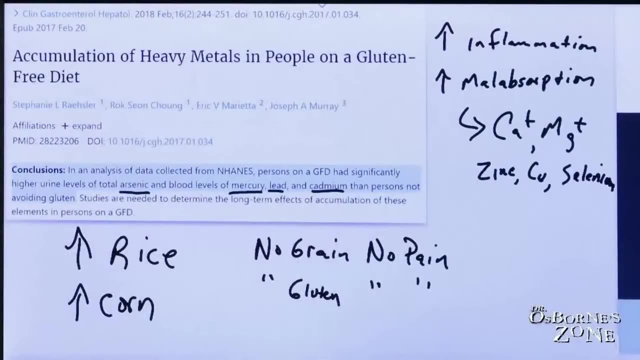 actually have a more profound effect. in other words, people with with poor mineral status are more impacted by heavy metals. they can actually become toxic more easily. in other words, healthy mineral status protects us in a sense from be over accumulating toxic metals because, remember, these metals compete with these metals. for 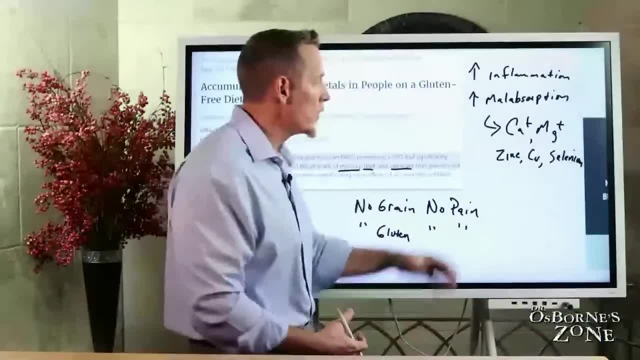 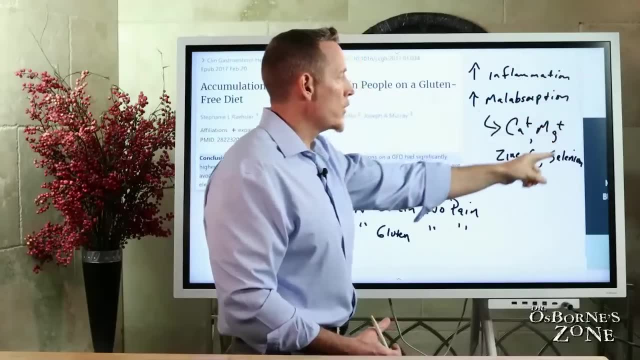 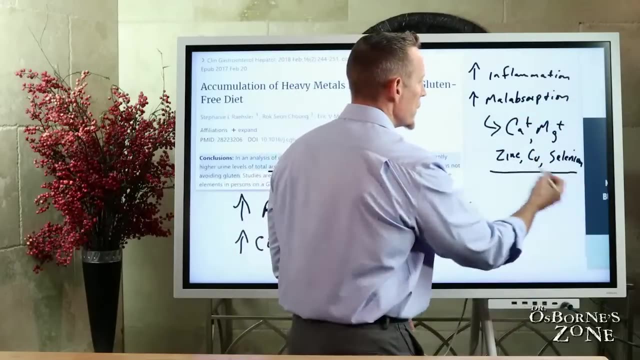 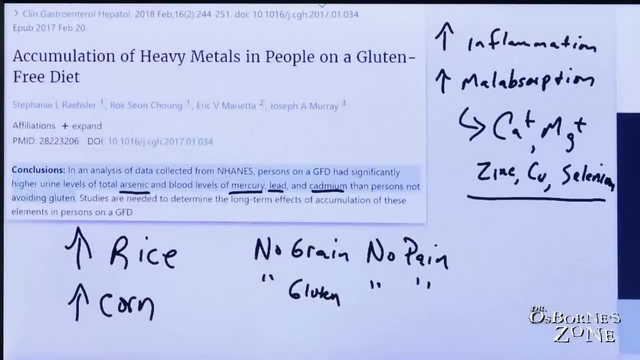 binding sites. this includes in the intestine for absorption, and so if you are malabsorbed here you you can pick up more of these things, especially- again, remember- if you're a newly diagnosed gluten sensitive individual or celiac individual. you probably already have some deficiencies in these minerals, and so you are at more risk for developing toxicity of these toxic. 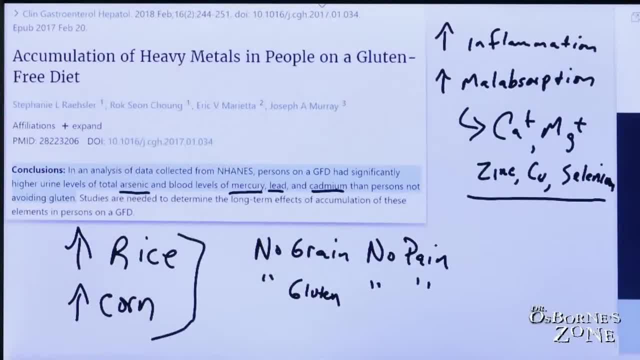 metals, and if you just jump on a diet that's high in rice and corn, you're going to increase your exposure to those things at a pivotal point, where you're most susceptible. so you have to be careful is why i put this up here, because i know a lot of you that follow and that watch us are. 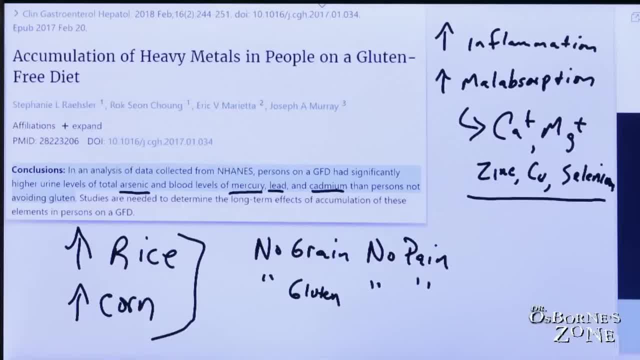 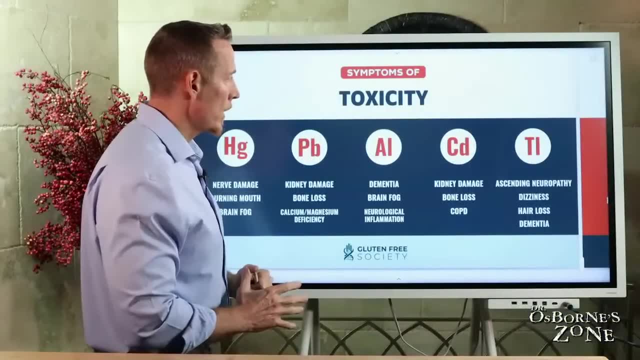 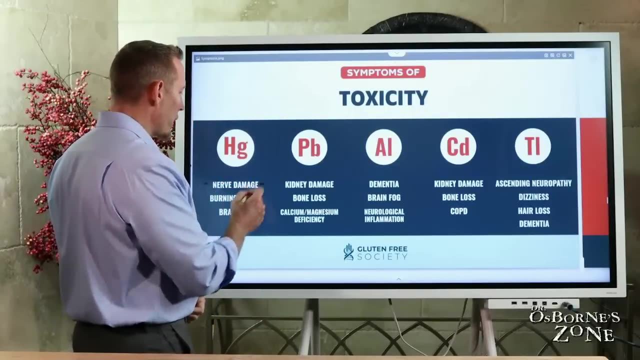 actual gluten sensitive individuals that that need to understand that that that's a potential problem for you. okay, let's talk about the toxicity symptoms of some of these metals. so if we're looking at mercury, mercury can cause nerve damage and a lot. i've seen this a lot where where people develop neuropathy. 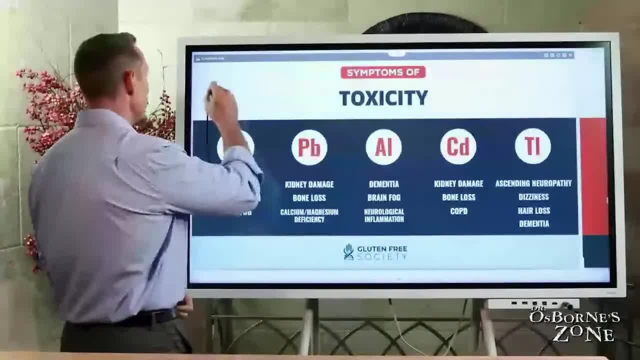 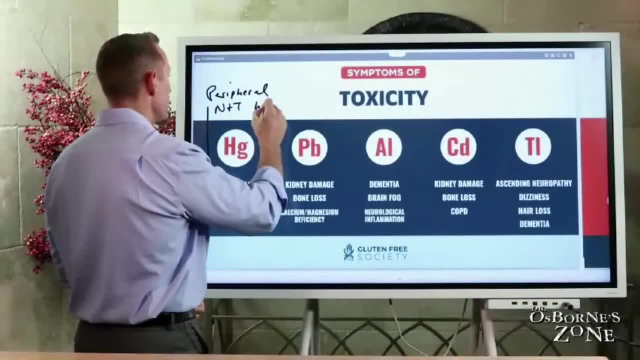 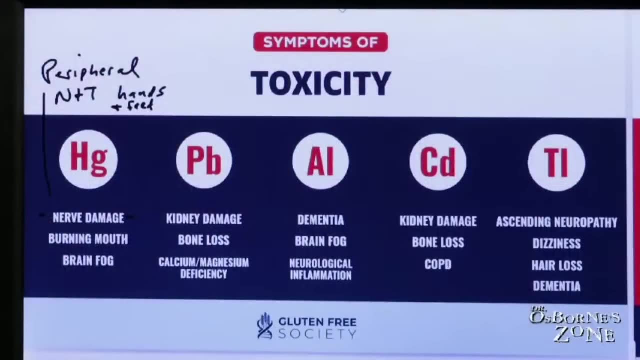 and then i've seen it multiple ways. so we see, we see like peripheral neuropathy, which would be something like numbness and tingling of the hands and feet. so we got to be careful with mercury, you know, because i mean a lot of times people get a diagnosis of you know. 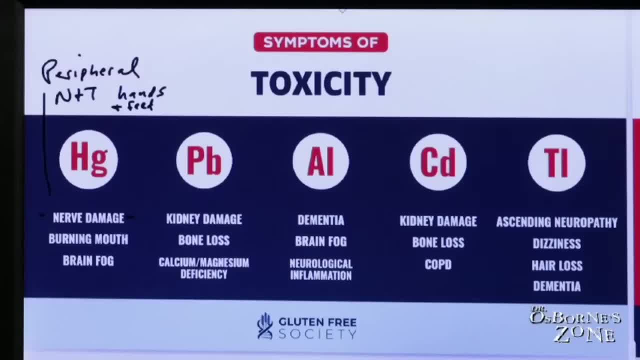 peripheral neuropathy. the doctors don't even, a lot of times don't even measure for mercury. you know some doctors will say, oh well, it's carpal tunnel syndrome or uh, or you have a diabetic neuropathy, because maybe they have some other disease complications. but looking for mercury is, in my experience anyway. 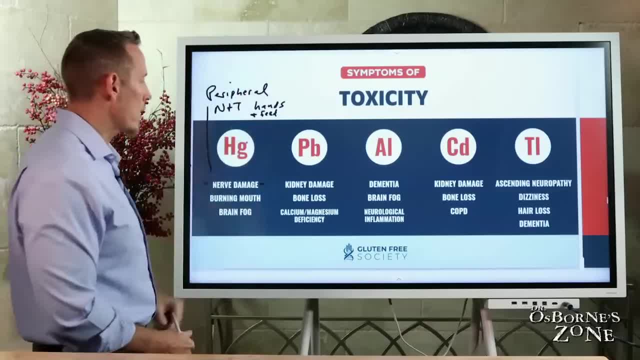 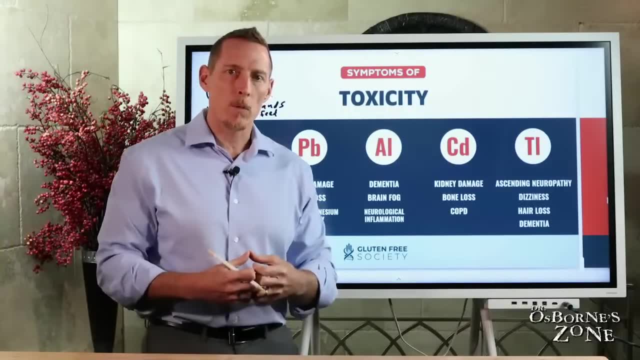 doctors very rarely actually look at it, but peripheral neuropathy is a very common manifestation. burning mouth- if you've ever felt like your mouth was scalding, like your tongue was felt like it was being scalded by burning hot water, or if you had a metallic taste, that's. 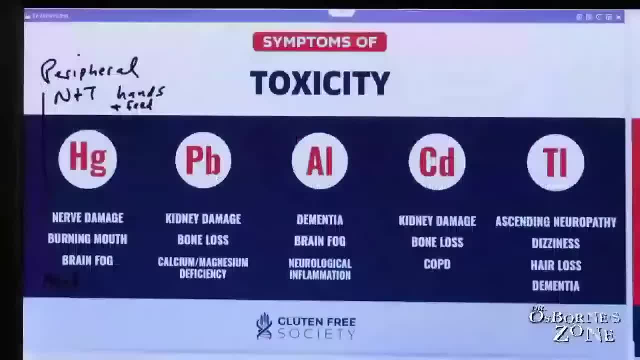 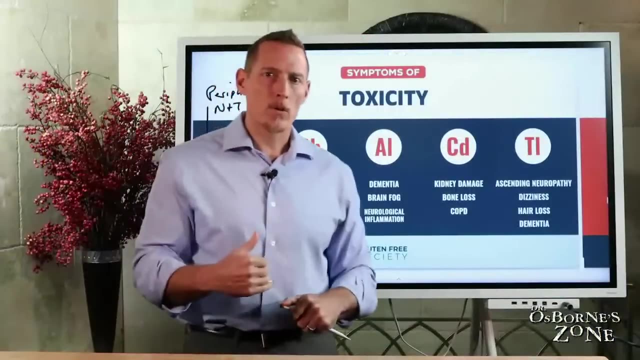 another one here. it's a metallic taste in your mouth. this can be a symptom of mercury. and then brain fog is a big one brain fog. i actually had a case one time as a woman who had silver. her problem was her silver amalgams. they were, they were, basically they were. they were leeching mercury through. 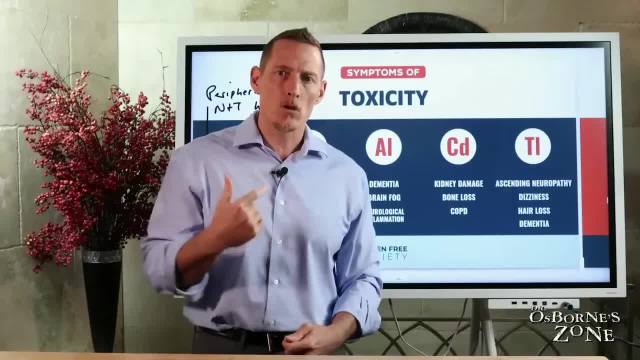 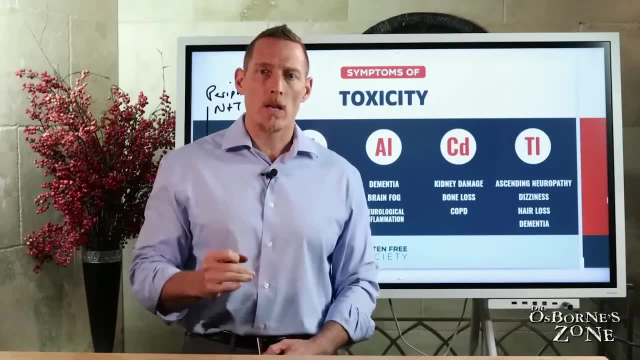 her cheeks into her bloodstream so every time she would eat, she was just slowly poisoning herself with her dental amalgams and she got to such a level where she couldn't remember her daughter's name. like her level of memory loss was, you know, was bordered on late stage dementia, and we've we. 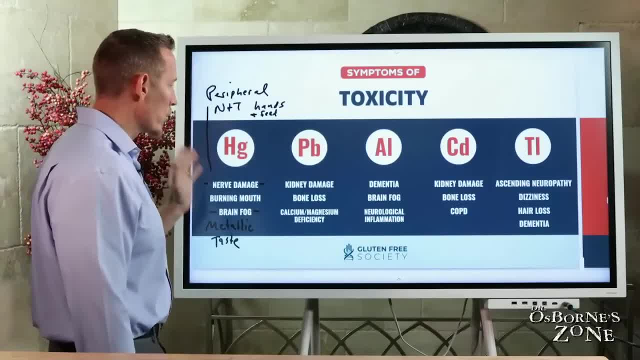 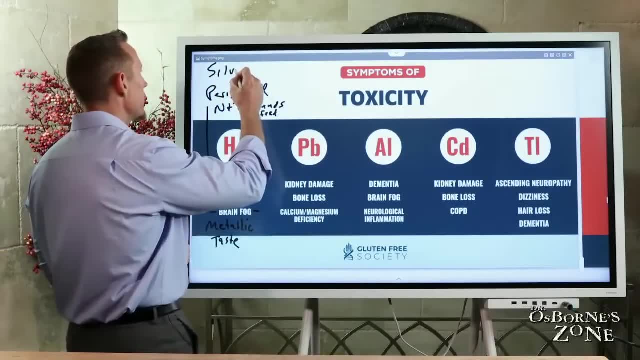 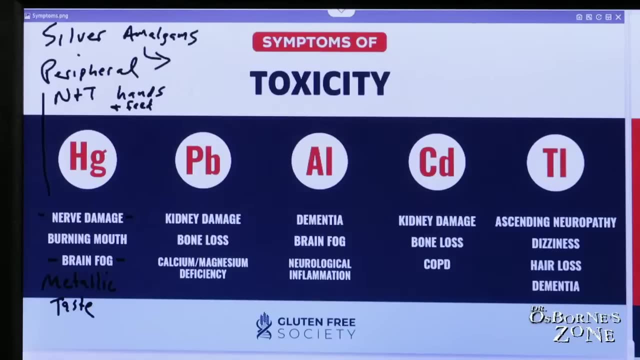 finally identified. her levels of of uh, of mercury were sky high and, of course, historically she had the silver amalgams, and so we sent her to a dentist and she had her amalgams removed again. silver amalgams came out and she made a full recovery. right, and that, that's the power of 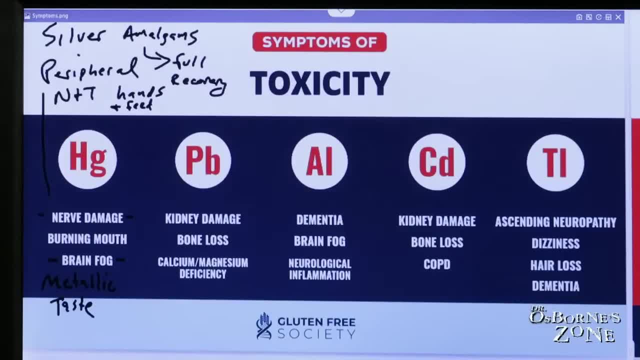 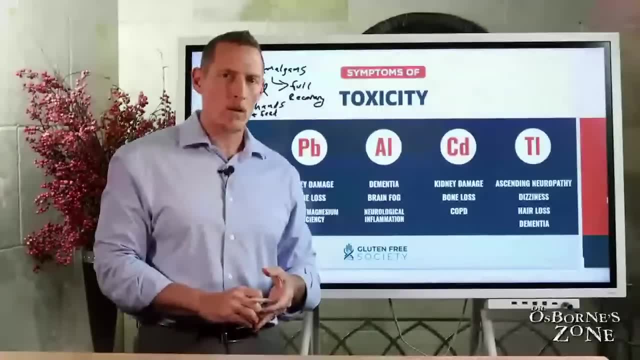 that's the power of knowing, okay, what the symptoms are. because if you, if you relate to these symptoms and you've, you know, done every other test and you've looked at every other thing and your diet is crystal clean and you know beyond that, this matches you and you've got. 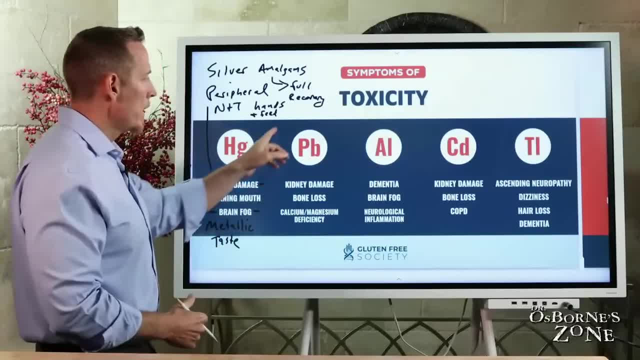 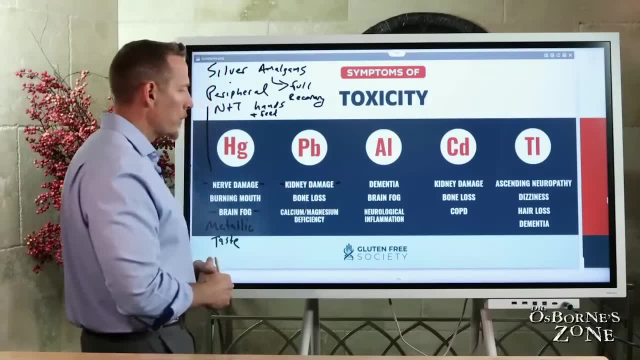 silver amalgams. you may want to go have that conversation with a dentist. we also have lead and lead, as i mentioned earlier, kidney damage is a major, is a major um problem with lead. so you know one of the tests, simple things that you can ask. you know if you've 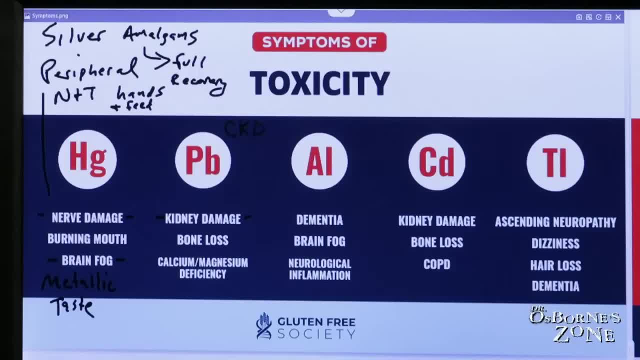 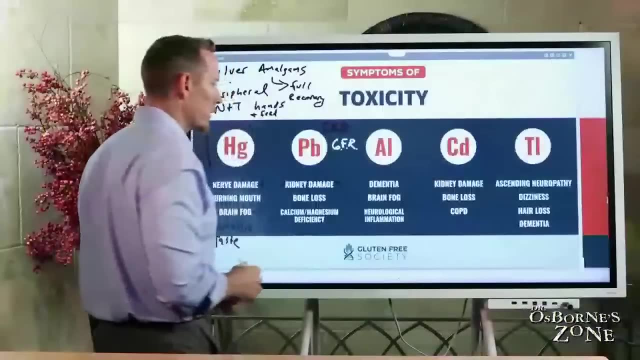 got chronic kidney disease, ckd, oftentimes abbreviated ckd: chronic kidney disease. one of the things that you know that den or not dennis, but your doctor will, will kind of monitor measure is something called your gfr- gfr stands for glomerular filtration rate. a lot of doctors 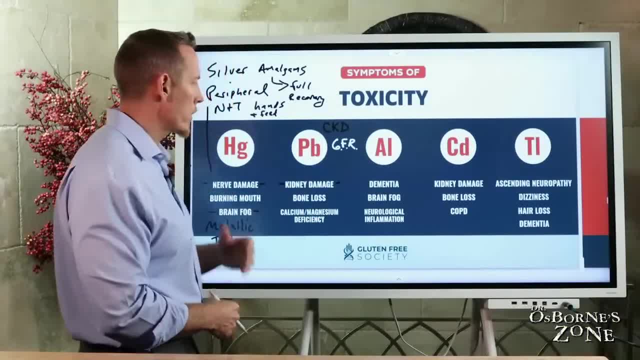 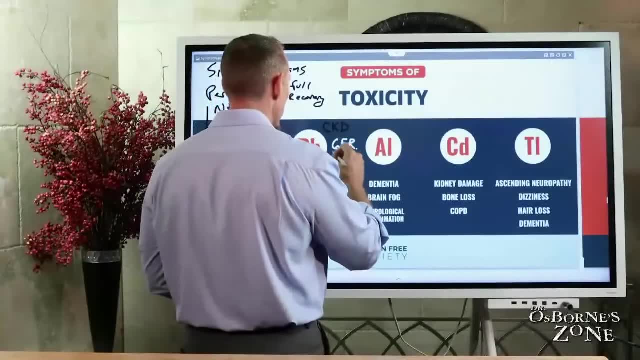 they'll do your blood work. they'll also measure creatinine and they'll measure your blood rea nitrogen or your bun. but gfr is a calculation and if your gfr, typically, if it's less than 60, so if it's below 60, then generally speaking they're going to call that some degree of kidney disease or chronic. 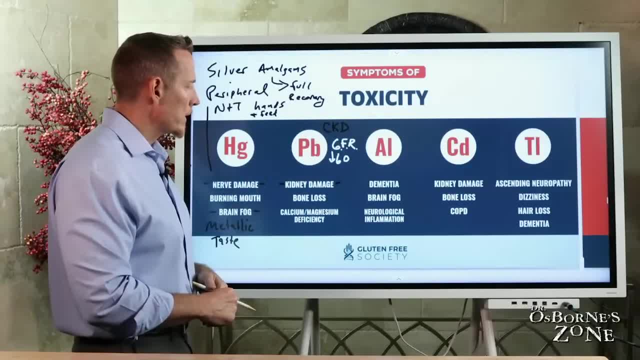 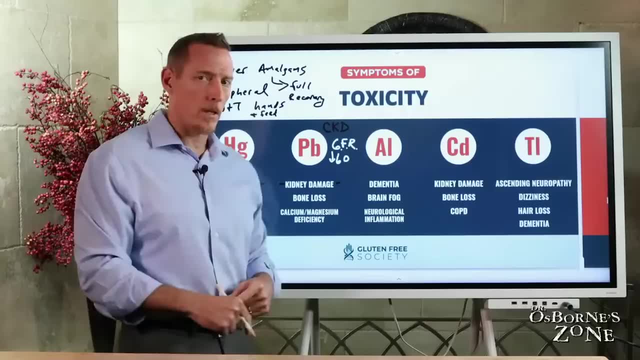 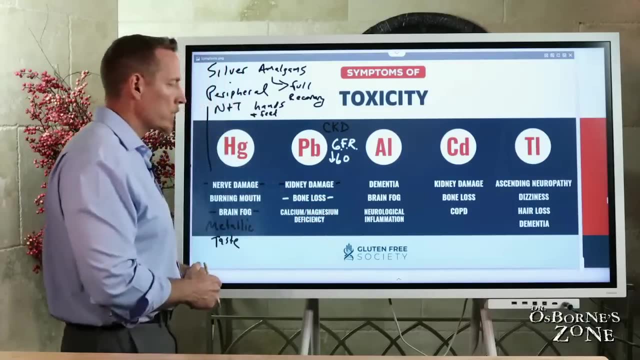 kidney disease or kidney failure, and this is something that's commonly seen in people with a historical. again, lead accumulation because, remember what i said earlier, lead bioaccumulates slowly and, especially if you grew up in the lead age and we'll see, lead also contributes to bone loss. it actually makes your bones more brittle and makes them less dense, and that's. 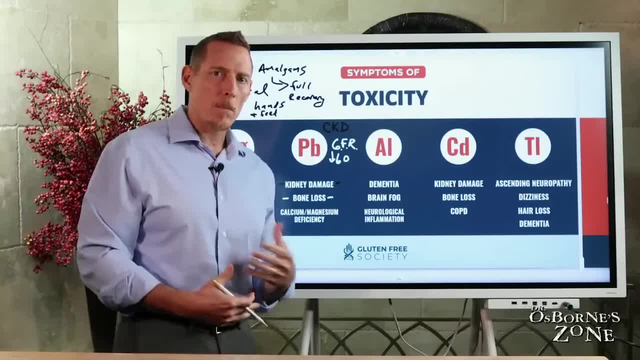 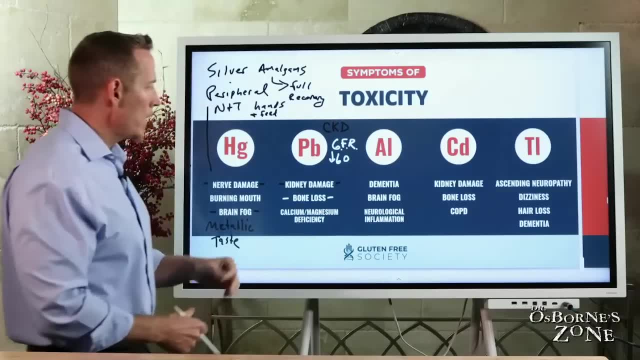 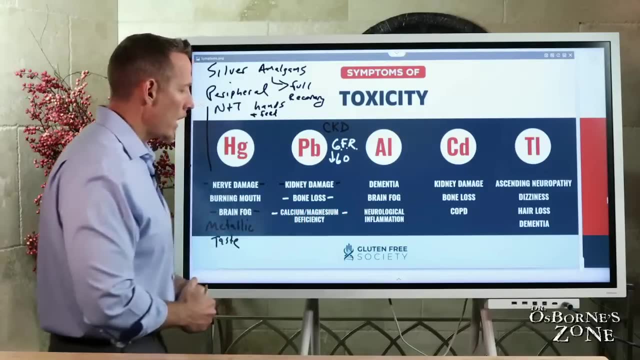 part of the reason why is it displaces calcium and zinc and magnesium from properly properly penetrating into the collagen matrix of bone and mineralizing it. so the other thing that we see a lot of times with lead toxicity is people that have calcium and magnesium deficiency and deficiency symptoms, and so what does that look like? that very commonly. looks like cramping in the muscles. you know toe and foot cramping, calf cramping at night can be symptoms. uh spasms, eyelid twitches, shoulder twitches. this is a very common problem. if you're involuntary, motor spasms or muscle spasms are very, very common. 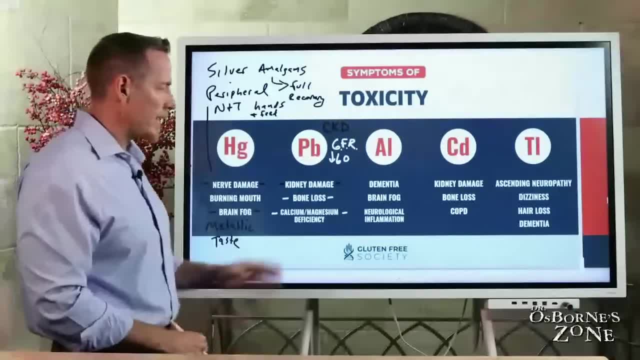 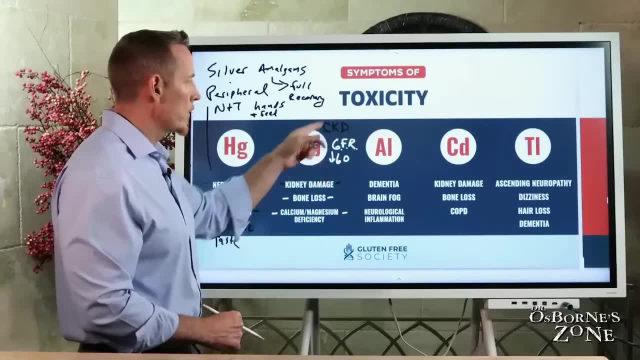 manifestation of calcium and magnesium deficiency. so if you've got that, don't know why your diets good, your nutrition is good again. you might want to have your levels of lead looked at, especially if you've got also unexplainable chronic kidney issues and don't know why. let's move on to aluminum. aluminum is a big 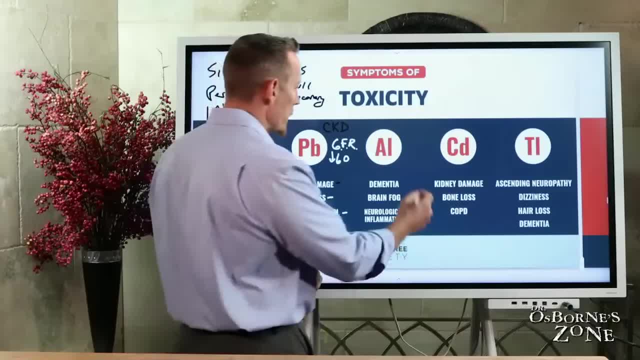 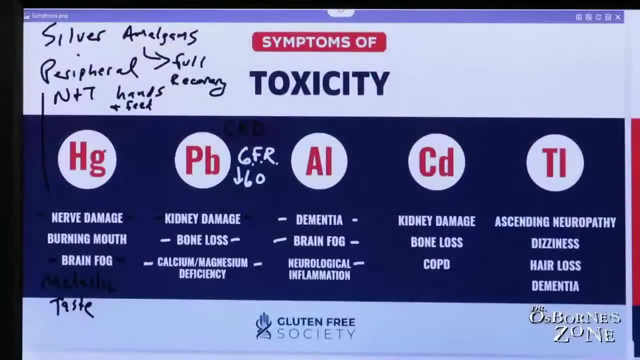 one that impacts and affects the brain. so we get dementia, memory loss, long-term, earlier term or shorter term. we get brain fog, neurological inflammation, and this can sometimes be found, you know, on an MRI. now there's a special type of MRI that's better at diagnosing brain inflammation. then then like a standard, 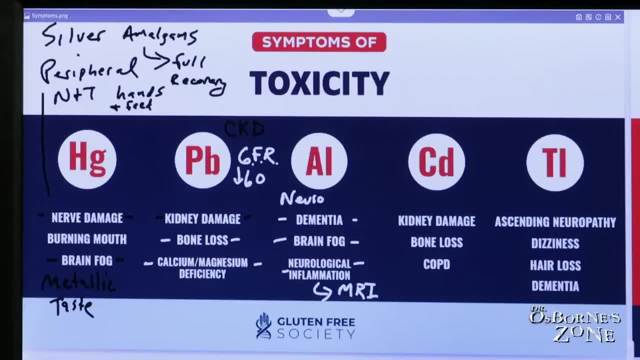 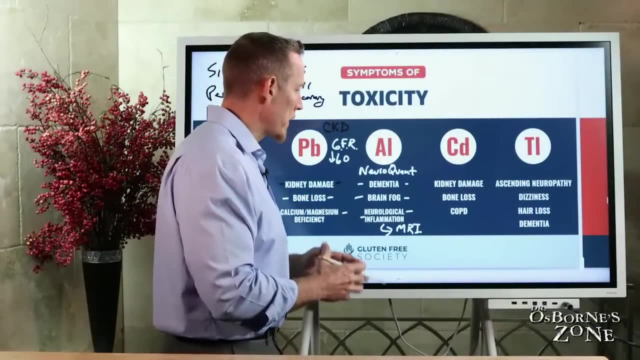 MRI and that you know. if you're talking with your doctor, you might just talk to them about this technology. it's called neuro quant and what that is is it's a three-dimensional MRI that can actually visualize the brain a lot better to pick up on nuanced inflammation- neurological inflammation. 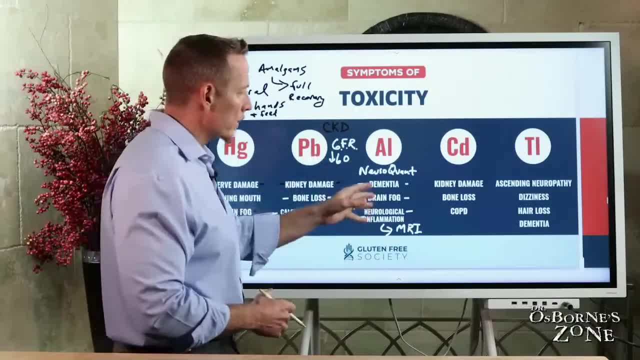 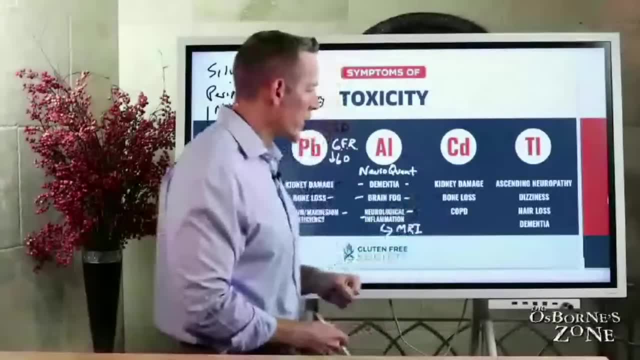 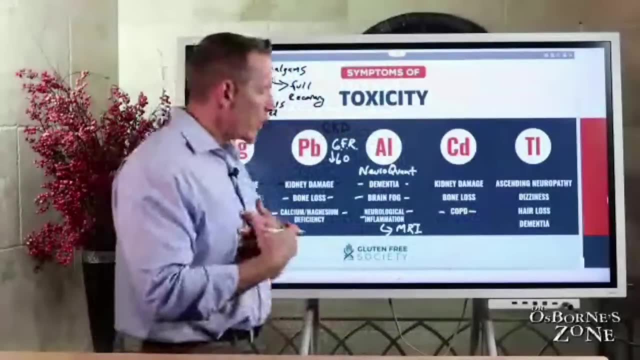 but aluminum very, very much. it impacts or affects the brain and we have cadmium. cadmium kit, like like lead, can cause kidney damage and bone loss. but one of the other symptoms of chronic cadmium exposure is chronic obstructive pulmonary disease. things like shortness of breath or air hunger are kind of 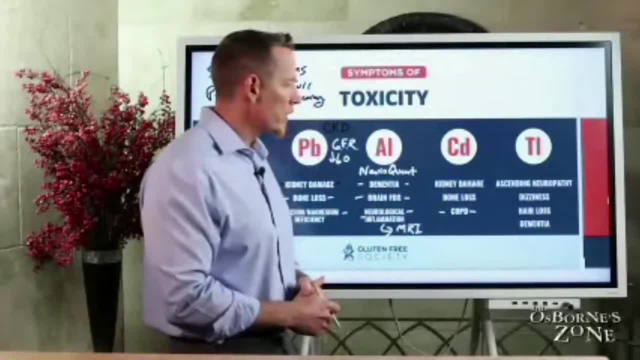 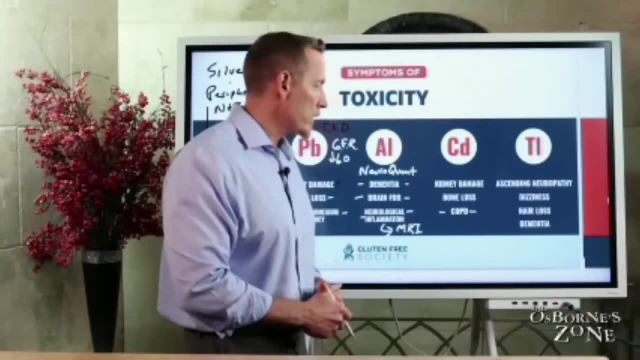 earlier warning symptoms of this. if you've got a chronic obstructive pulmonary disease, if you've got a chronic obstructive pulmonary disease, if you've got a been diagnosed with a type of COPD and you also have kidney disease and you've also been told that you have bone loss or or osteoporosis or osteopenia, you know. 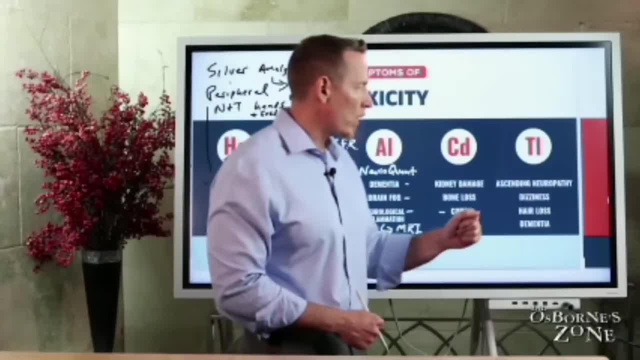 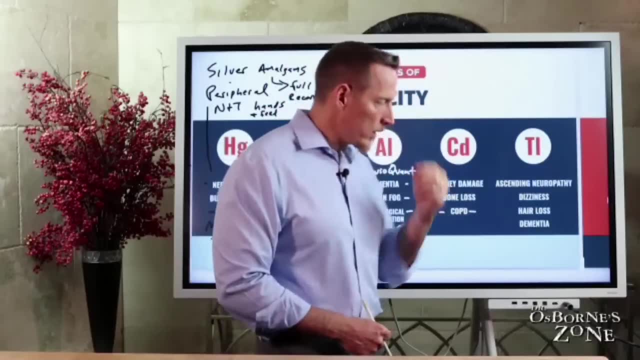 check it out, cadmium might be something that's contributing to that problem. and then we have thallium and thallium- one of the one of the hallmarks- actually saw a case of thallium toxicity years ago, and this was in a case where a young 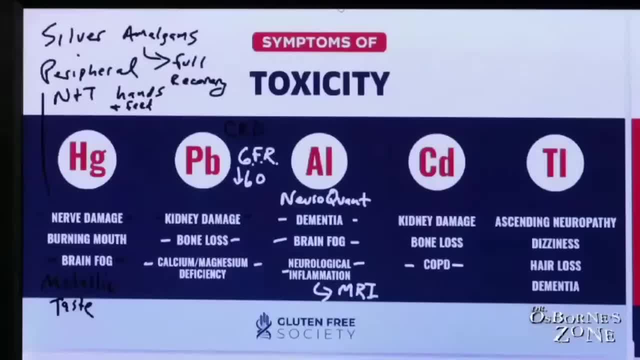 woman had ascending neuropathy, where where the neuropathy started in the toes and it moved its way up, you know, moved its way up the legs, and hence the term ascending. it's going up. it's moving its way up as it gets worse. the problem starts low and it works its way high. she actually, by the time she made it to me, 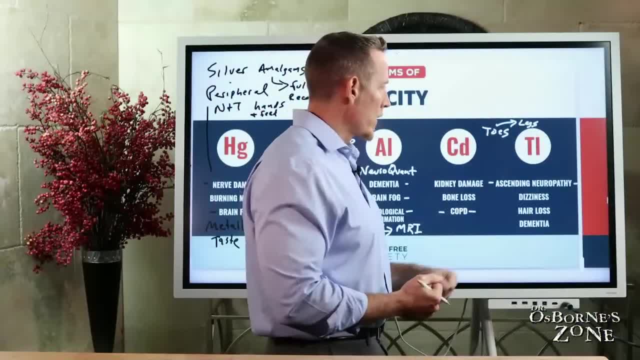 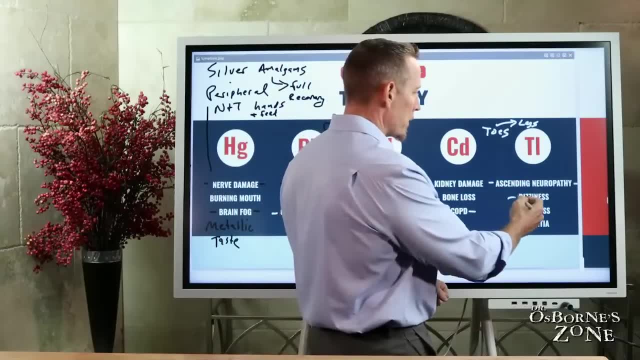 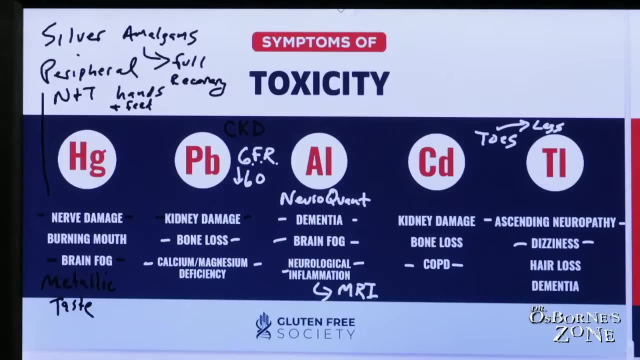 she was in a wheelchair. you know we were able to reverse this, but thallium was playing a big part of this issue. dizziness, you know, without with unexplainable dizziness can be a symptom of thallium toxicity: hair loss, as well as dementia as well. since we talked about arsenic, 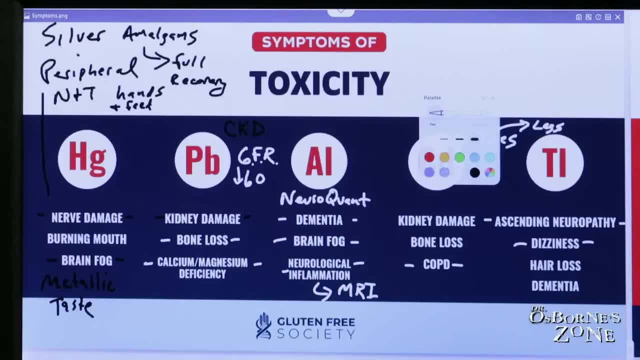 earlier I said we'll add it as a bonus. let's just fill in some things with arsenic here. so arsenic can lead to a number of different problems. it's been linked to bone loss as well, but on the skin it'll oftentimes lead to. 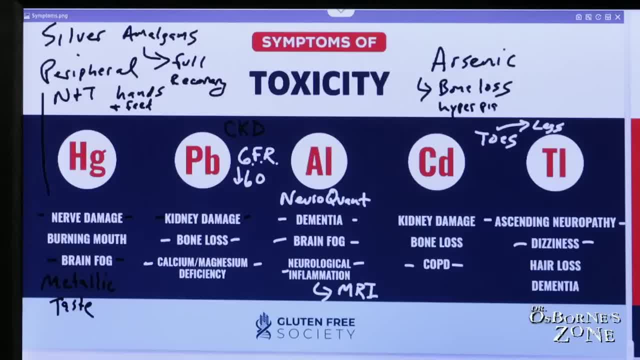 hyperpigmentation. hyperpigmentation of the skin of the feet, particularly black foot disease, can be a manifestation of chronic arsenic exposure. now again difference between acute and chronic, but black foot hyperpigmentation of the skin not uncommon to see. and then we also see with arsenic you get a lot of nausea and GI symptoms as well. and 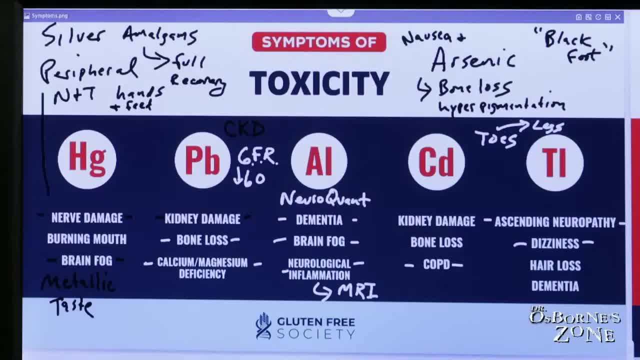 there's a, there's a, there's a marking that can appear on the nails, and so if you look at like a, like a, like a fingernail, so let's just imagine that's a fingernail, okay, and there's a little moon in the nail, but you'll get lines. 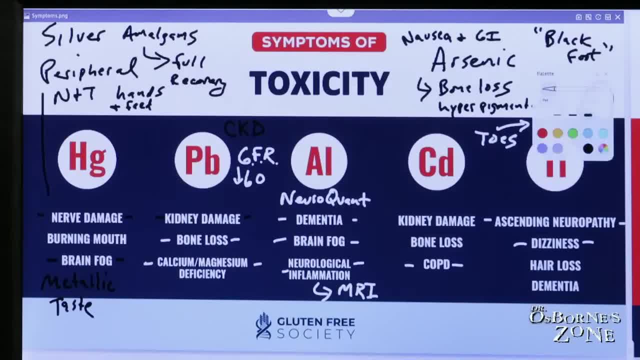 going across and they'll be horizontal. let's make them a different color. horizontal lines kind of going across the nail. so you'll see this pattern where they're kind of growing this way and those are called Mies lines. M-E-E-S apostrophe Mies lines. 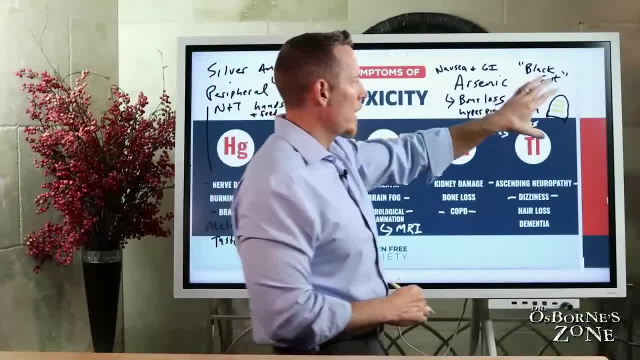 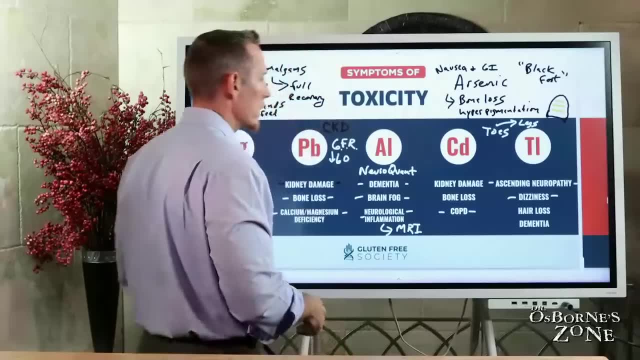 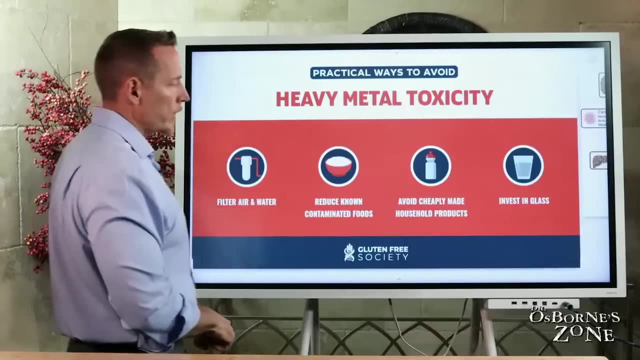 but those will be white. I drew them as yellow because we're on a white background here, but lines like that patternistically horizontal, going across the nail beds, could also mean arsenic poisoning or arsenic toxicity as well. okay, let's talk about how do we avoid it, so we know what to look for. what are the? 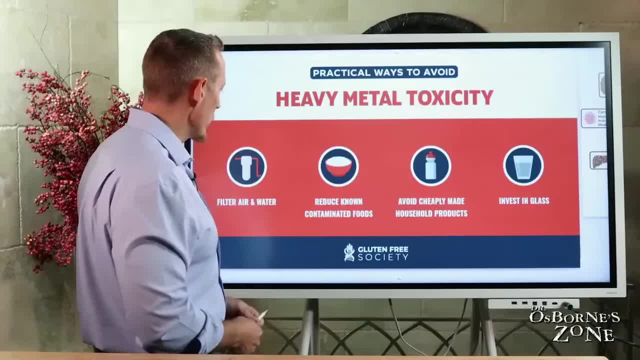 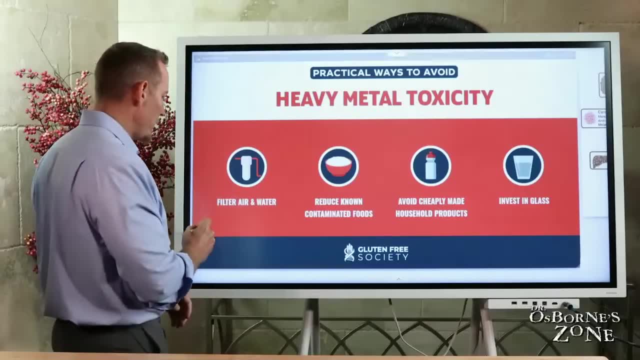 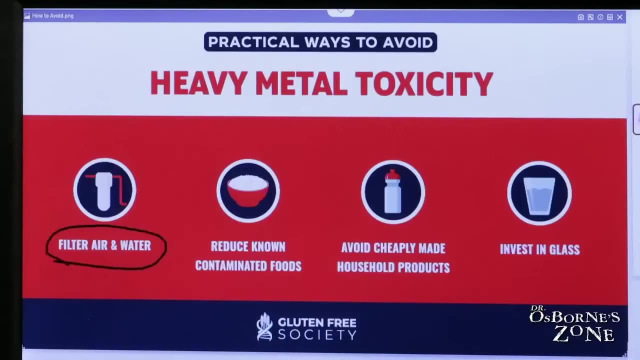 symptoms. but now what do we do to avoid exposure? so the number one thing that you can do- in my opinion, everybody living in an industrialized area should filtering air and water. you know best types of filters. you know my opinion: filtering the air you want, like a HEPA filter, is a really good place to start. 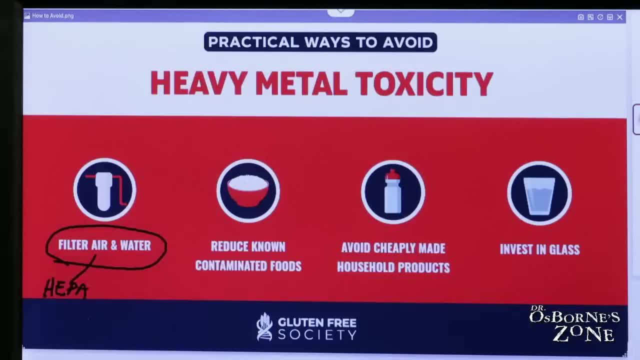 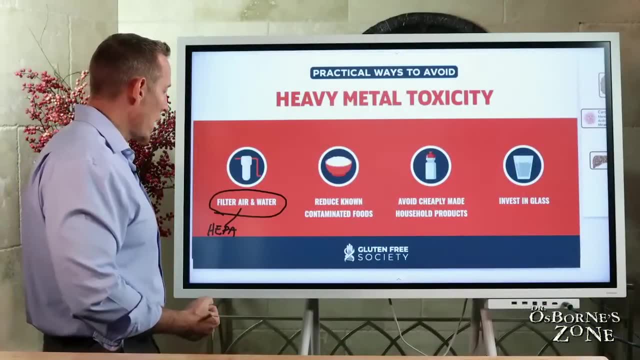 it's relatively inexpensive for most people. you can get a HEPA. you can buy them at Walmart. you can buy them, you know, at the local store for you know a few hundred dollars. you know you can actually. you know that's if you don't have, depending on where you live. you live in an apartment, you don't own the. 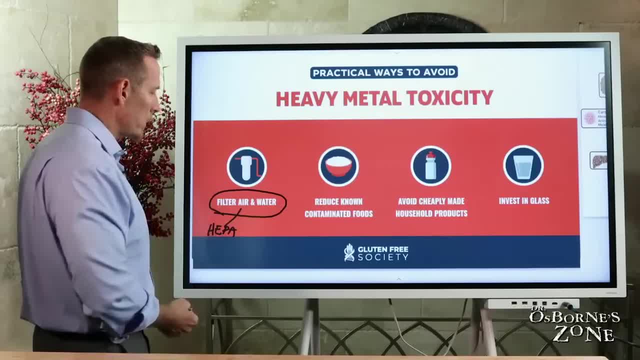 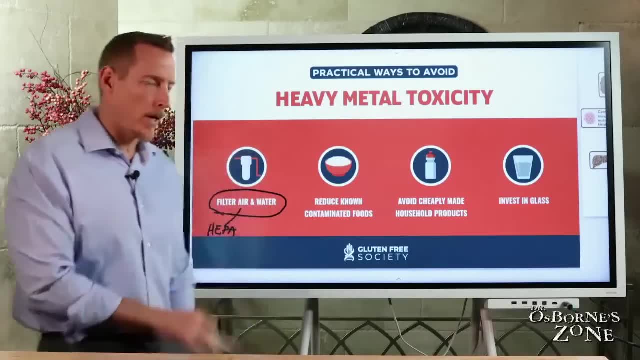 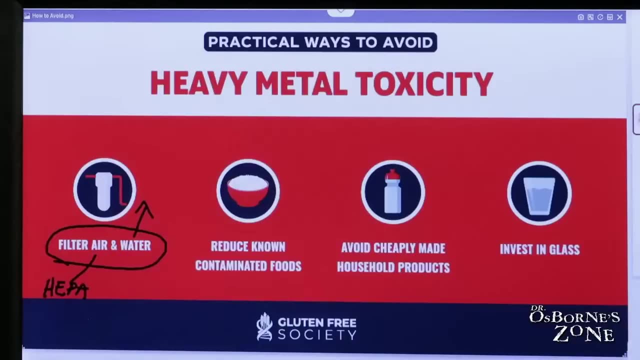 building. you obviously want to have a standalone filter that you can use. now, if you only have yet you own your own home. you may want to look at some more advanced filtration that you can add to your HVAC system, but this is a really good place to start, and then water and, if you live in the city, probably the 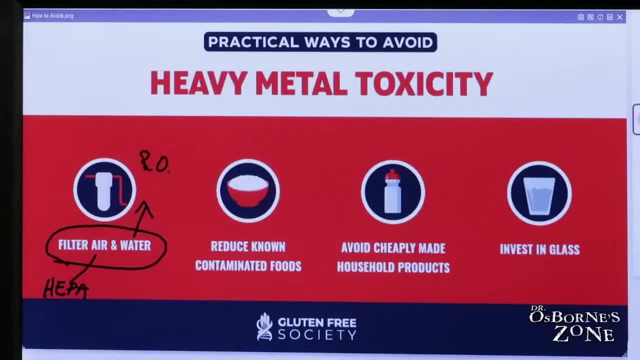 best way to filter your water is reverse osmosis. the reason why is RO will pull out all the metals and one. you know the carbon does good too. so you know RO is not the only option here. you could look for a carbon. actually, specifically, granular activated carbon and KDF do a good job as 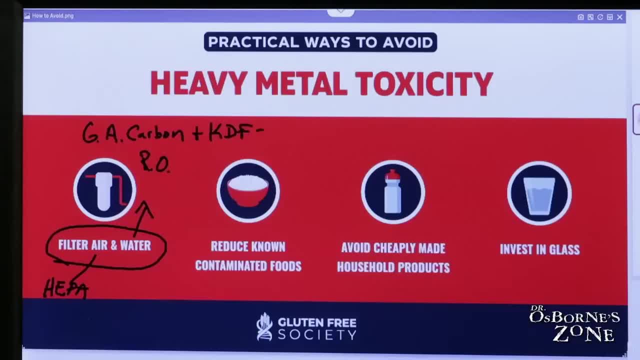 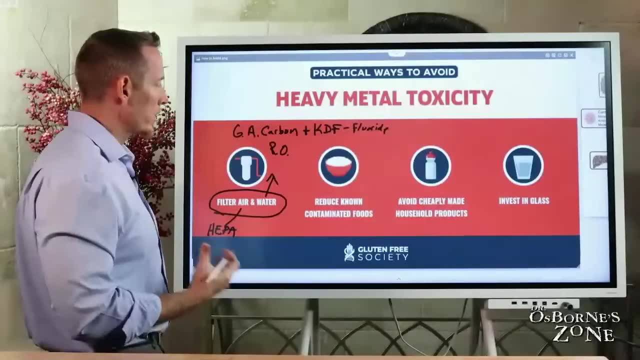 well what? what? carbon and KDF don't pull very well. they don't pull out fluoride, which we're not talking about. fluoride today, although fluoride is, it is a metalloid or a type of metal that's a toxin that's oftentimes added to water and can be problematic as well, but RO pulls fluoride. 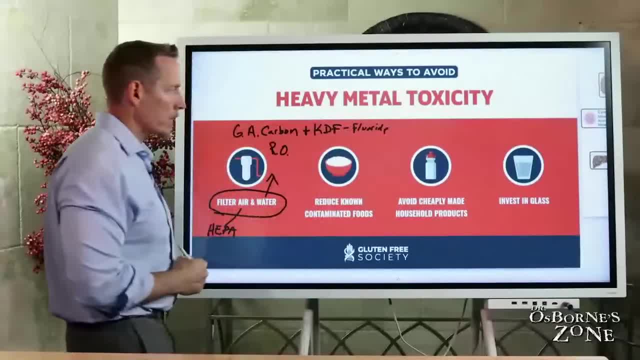 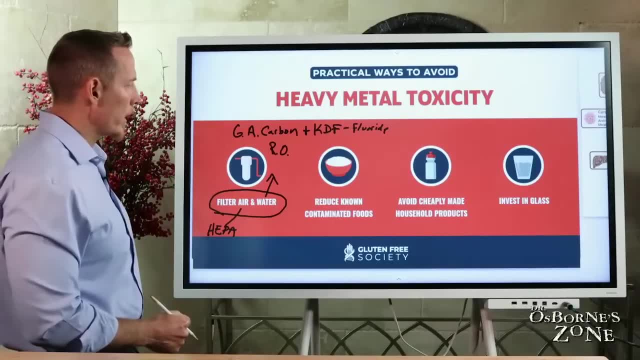 carbon and KDF will pull out a lot of the the other contaminant metals, but RO does a better job all the way around. so RO, in my opinion, if you live in the city, is a great type of filtering device. just remember, if you use RO, you want to add. 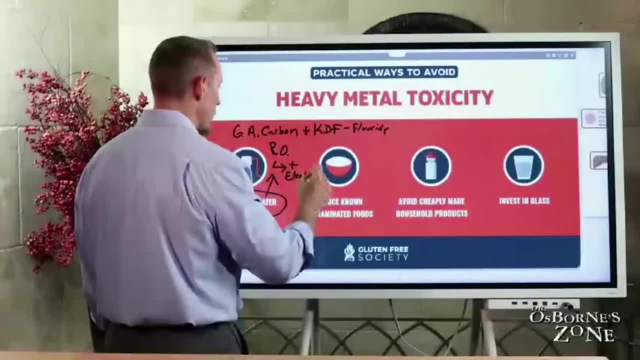 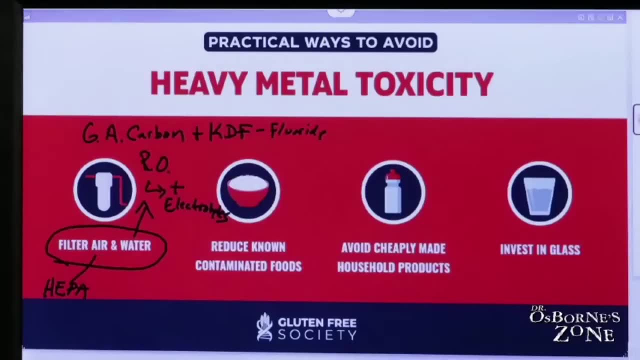 electrolytes back to your water. we have something called ultra electrolytes- a gluten-free society that you can check out, but it's a good idea to add electrolytes back to the water if you're going to use RO as a filtration. but filtering your air and water is going to help protect you. it's just a. it's a. 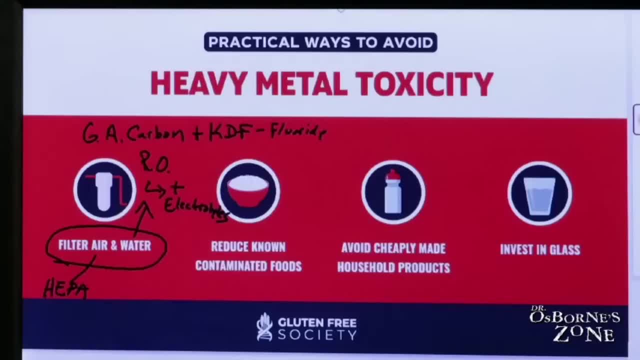 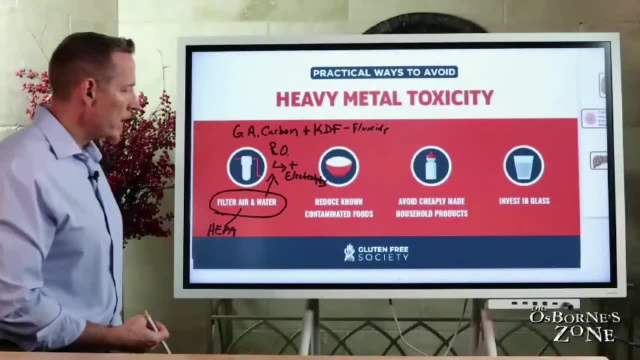 shield to protect you from what we know is already happening. our environments are contaminated with heavy metals- the air, the water, the soil- and that's not going to change anytime soon. I don't see all the the the big companies and big corporations saying: oh, we're gonna stop poisoning things and quit making money. I 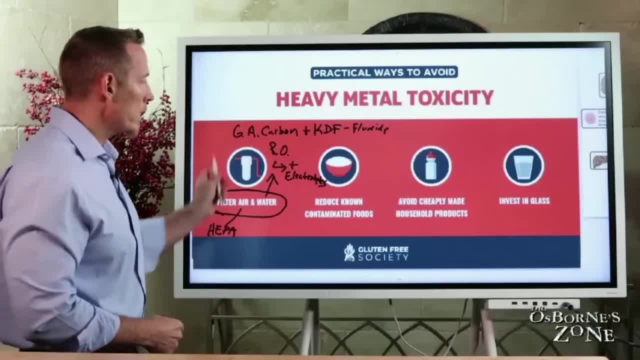 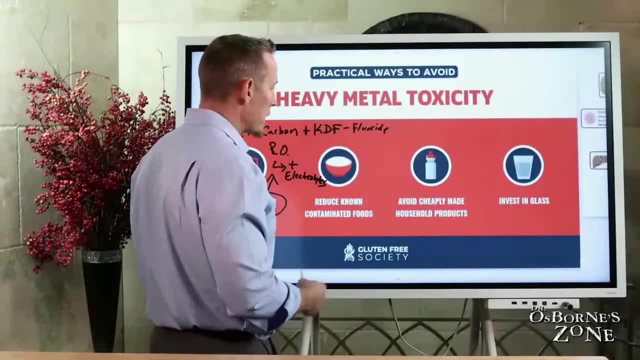 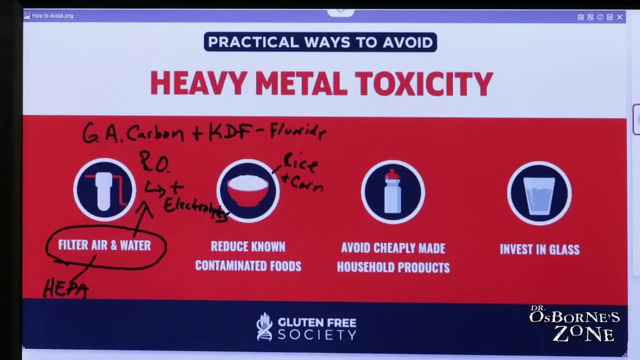 don't see that as a realistic possibility, so we're gonna continue to be exposed to these things, so the best you can do is filter. the other thing is to reduce known contaminated foods and not make them staples. rice is probably arguably one of the biggest rice and corn. as I mentioned earlier, there's some recent, you know. 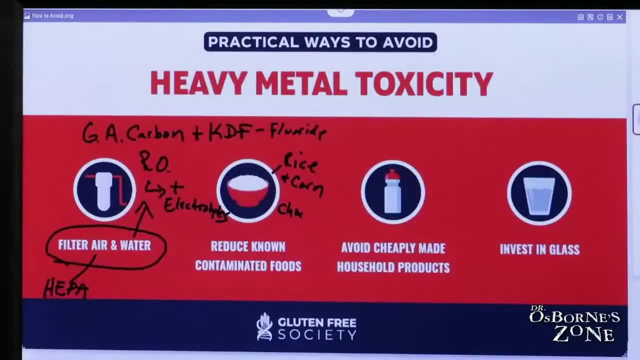 noise about chocolate as being contaminated with some lead, and so I would, I would say, proceed with caution. I think I think with chocolate, nobody should be eating chocolate as a staple food anyway, and this- and you know that the case with foods is, you know, if you're gluten sensitive, I recommend you avoid these anyway. but if 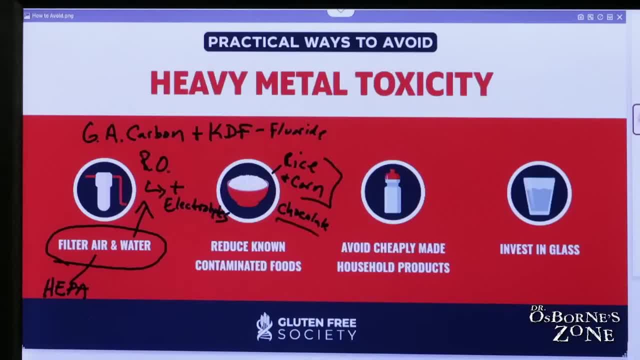 you are a chocoholic or if you're not gluten sensitive, but you just eat rice at every meal. you just need to be aware that there's a heavy potential for contamination there, and if you're struggling in your health, you may be creating problems or you may be contributing to those problems by using. 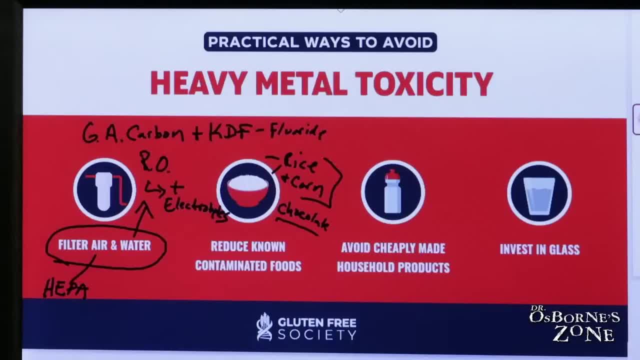 those as staple foods. avoid cheaply made household products. you know you get what you pay for is that old adage, and I know, with inflation and everything, the way that it's going. this is for some to say and harder for some to do, but really honestly, when it comes to 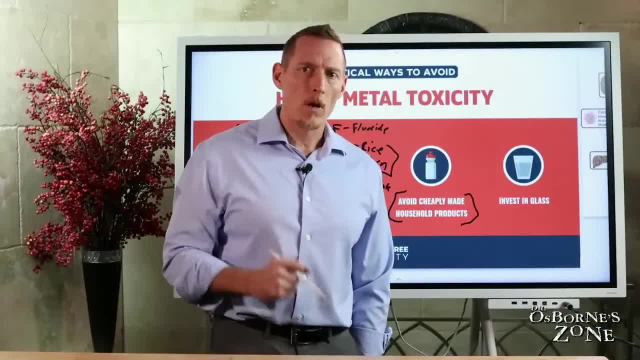 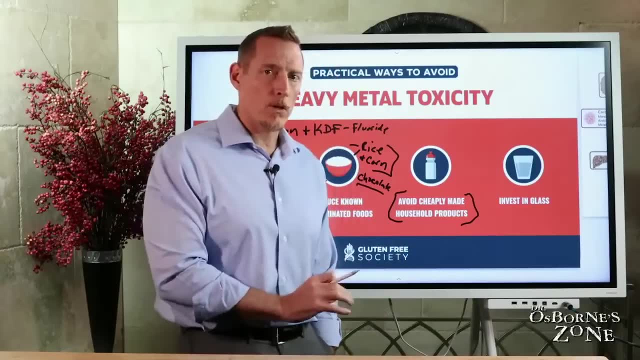 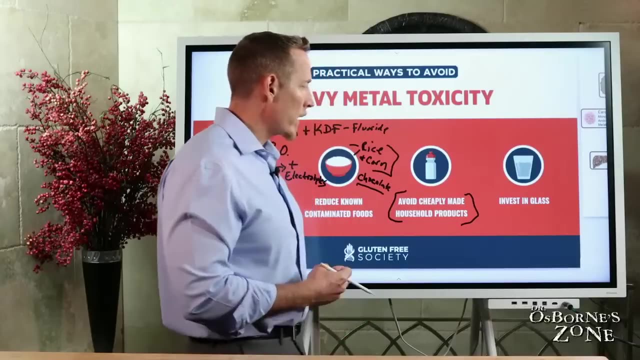 the things that you eat off of, eat out of or cook or prepare your foods in. you know, prioritize those things first, because you want to reduce your potential that you're going to ingest, eating or consuming heavy metals, because by ingesting them you increase the risk of creating a problem. the other thing is 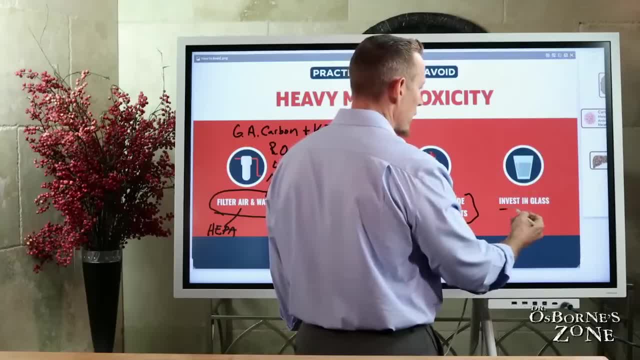 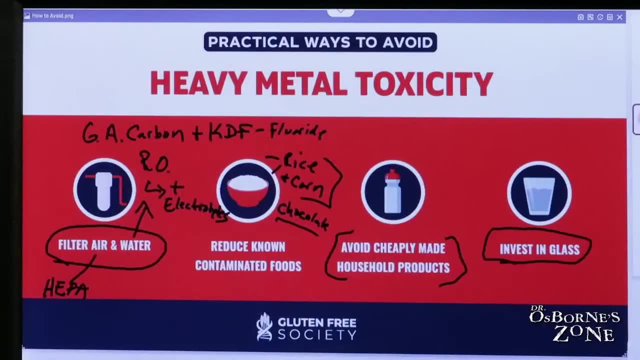 a lot of your said- eating and drinking and cooking- invest in glass. glass is cheap, right, so this is no more of an expensive thing. but if you're drinking out of plastic cups or like cheap metal cups, again produced in foreign countries like China and India, you run a risk of heavy metal contamination because 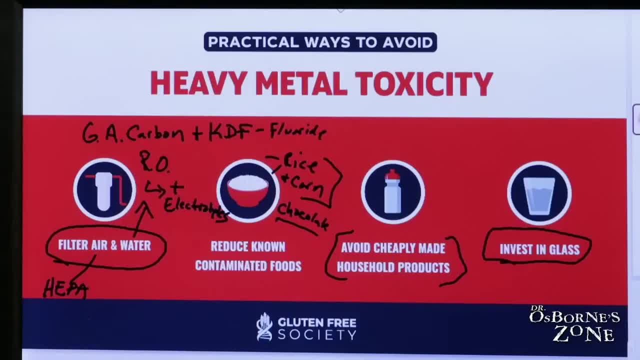 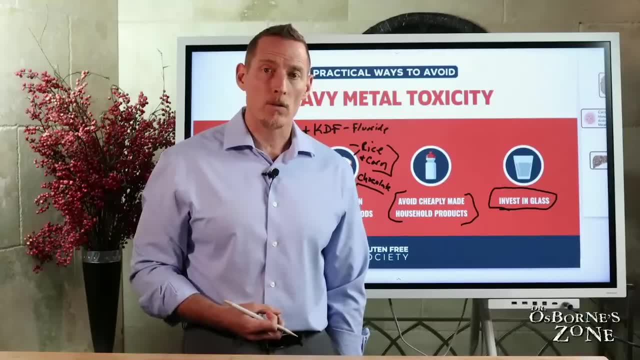 there's lower standards and there's lower restrictions. environmental restrictions: if we look at, you know, environmental pollutants produced, you know per capita, China and India are at the top of the list. the us is very low down on that list because we have really pretty good environmental restrictions. 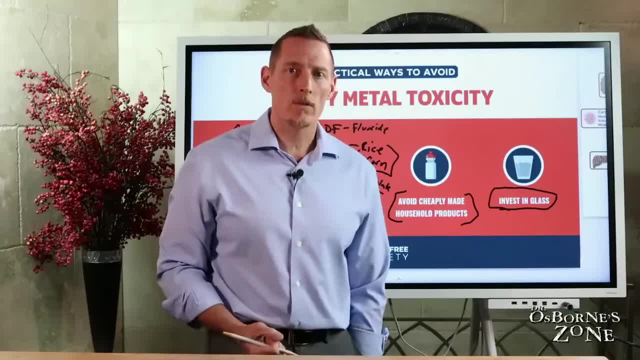 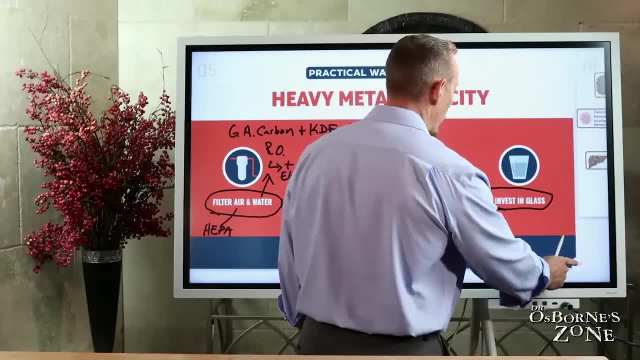 and standards, and we're actually less polluted a day than we were in the 70s because of those restrictions. but again, a lot of our manufacturing has gone overseas and so we're just bringing this poison back to us. so try to avoid that. some things that. 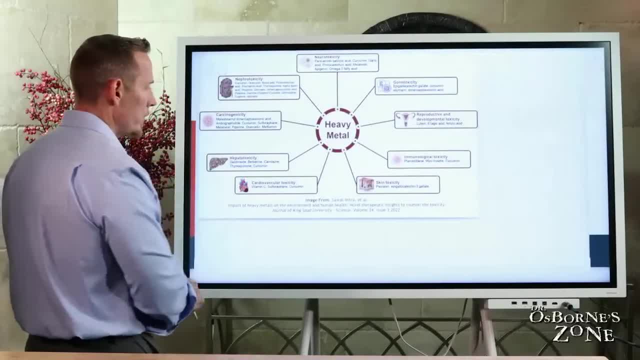 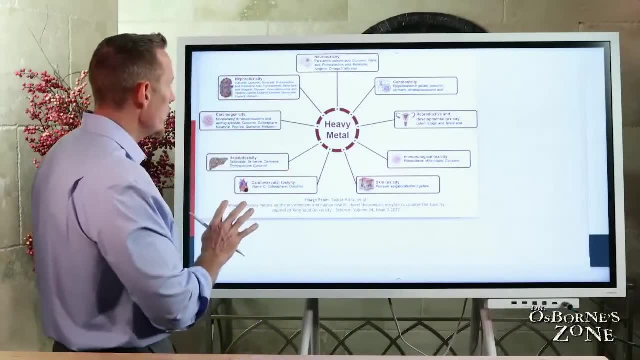 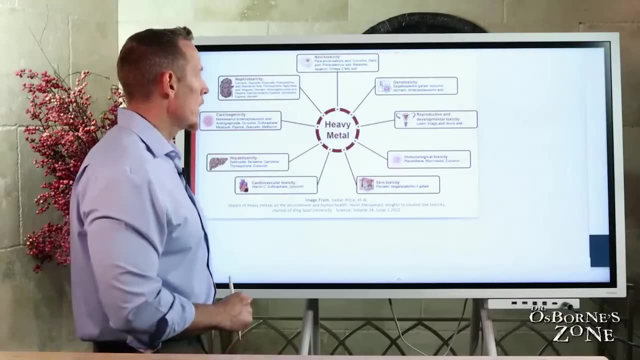 you can do so. one of the one of the things that these authors did, you know, in this particular paper was- and this was was it was just published in 2022- is they kind of accumulated, all the different types of things that we really things that you could do, whether it was through your diet. 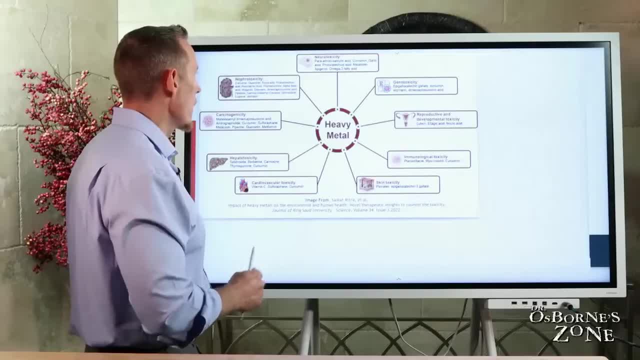 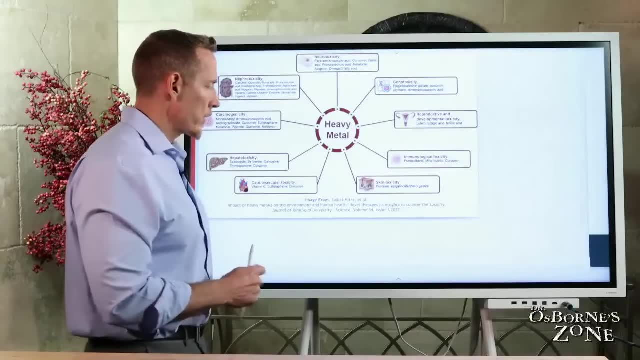 or through different types of medications. they were trying to summarize how you could offset the different toxicities that came from different heavy metals, And their concern was that, because there's a way that in medicine heavy metals are actually- oftentimes they're treated. 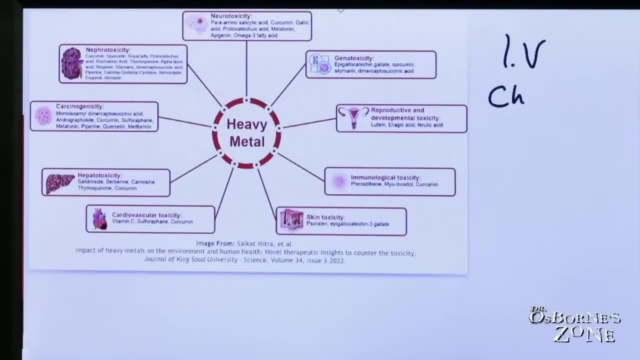 through something called IV chelation. Some people wanna pronounce it chelation because it's C-H, but the C-H is actually pronounced kuh, like key chelation, And so IV chelation with substances like DMSA and DMSO. 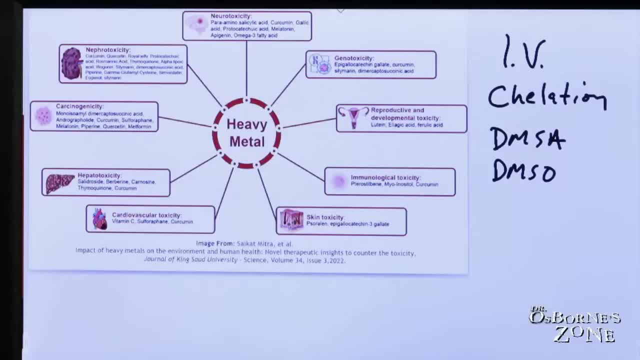 are very common choices medically to pull metals out of you. So these are IV treatments. They will run these chemicals through your body and these chemicals work as binding agents. They will bind onto toxic metals and then pull them out of you. 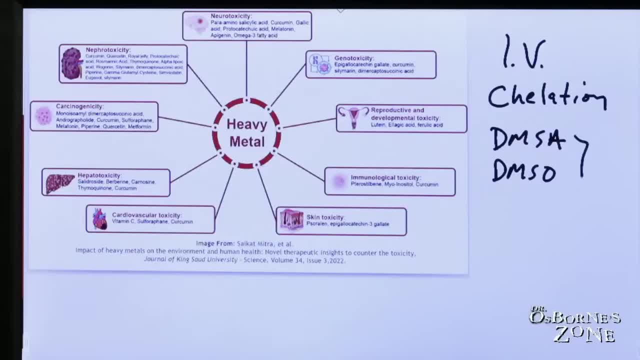 And so doing that, though these two, these two compounds are not specific for bad guys. They will pull not just lead and arsenic and mercury and cadmium and thallium, but they will also pull calcium and magnesium and zinc, And so you have to be aware that when you do IV chelation, 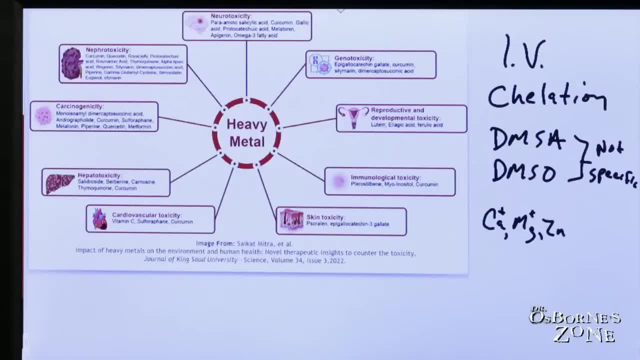 you should also your doctor that you're working with should have a plan where he is also remineralizing you, making sure he's adding minerals back to you to prevent mineral deficiency, because that's one of the risks with doing IV chelation. 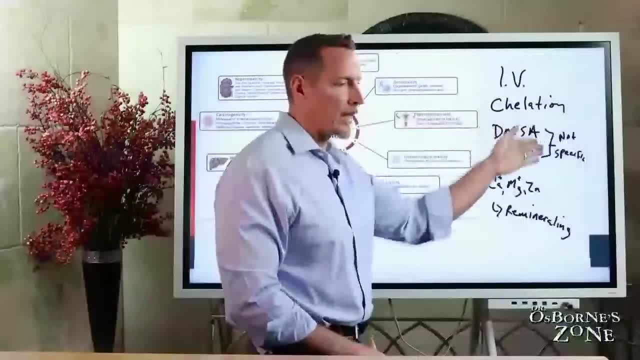 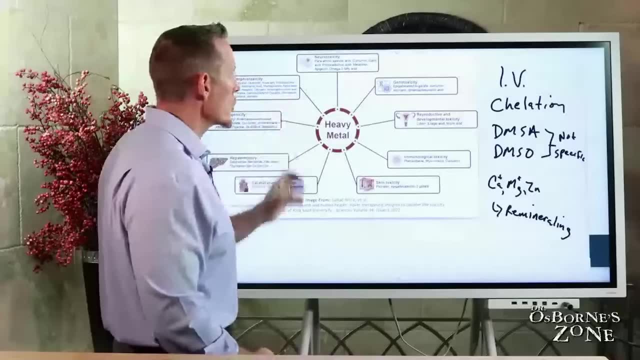 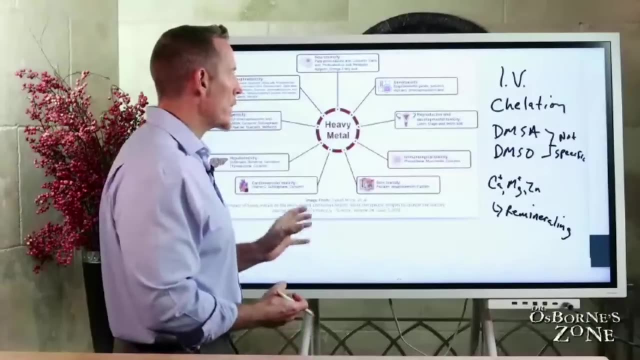 is that you cause mineral deficits. in the process of pulling out the bad stuff, you're also pulling out the good stuff. These scientists got together and said: well, how could we make nutritional recommendations or lifestyle recommendations to mitigate some of the potential poisonous effects of heavy metals? 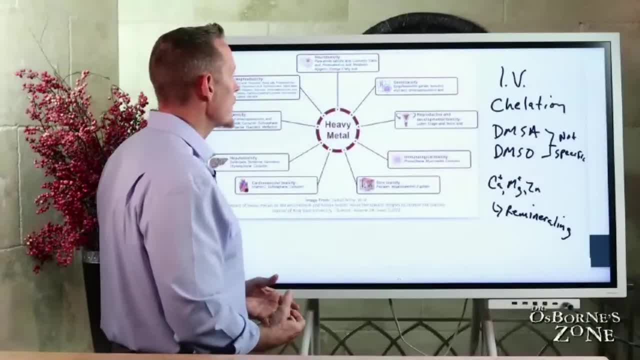 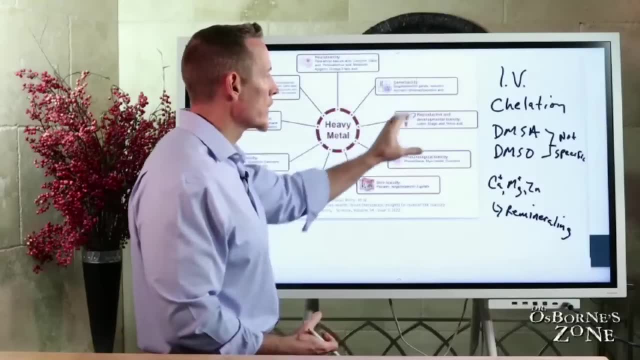 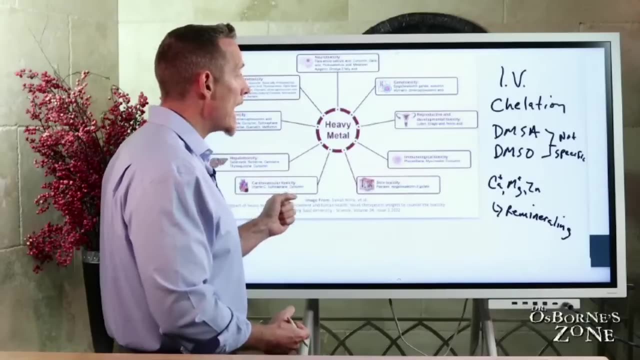 And so they came up with certain food-based items that have known protective effects, And so I would say this is more along the lines of: if you have the damage from heavy metals, these are natural things you can do with your diet or lifestyle. that would allow you to negate. 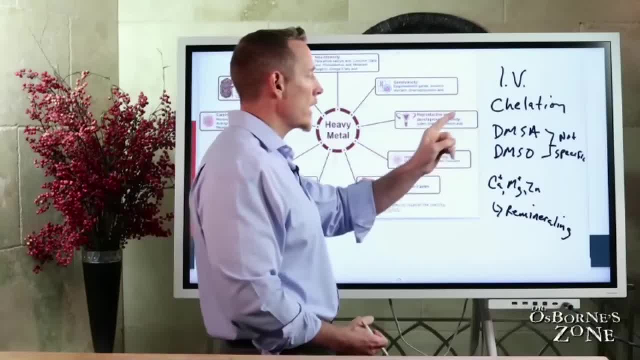 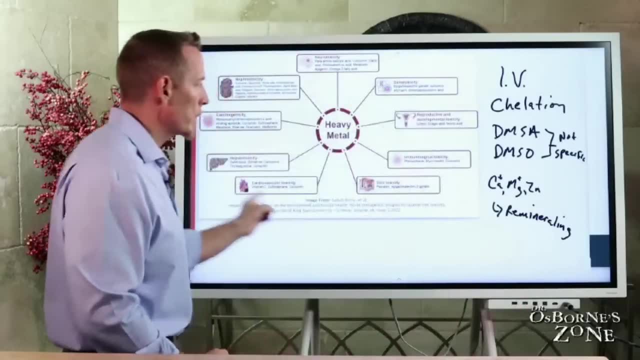 some of the toxic effects. But again, at the end of the day, I agree that I think that chelation you gotta get the metal out of you. If you never get the metal out of you, you're stuck over here just using a bunch of supplements. 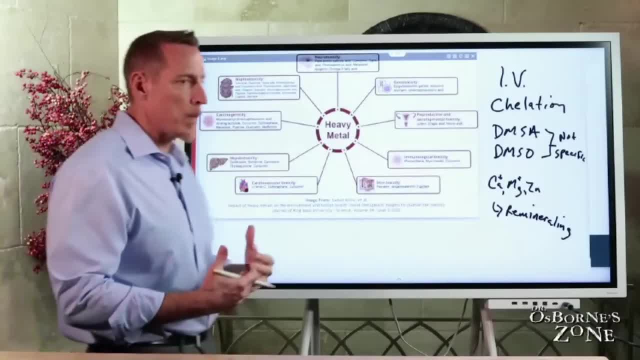 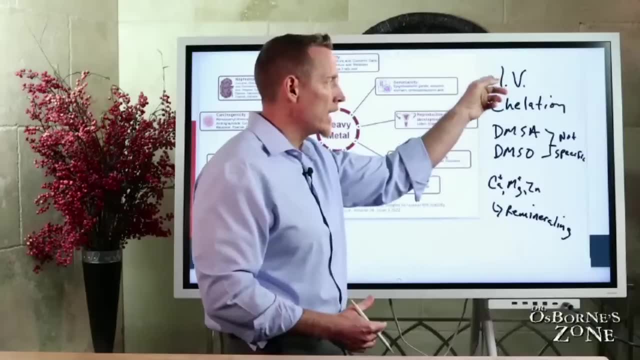 or food-based items, And so I think you're gonna need to get the metal out of you just to try to offset the damage. But remember, metals will bioaccumulate and stay lodged in your tissues and you really, if you're high, you wanna get them out of you. 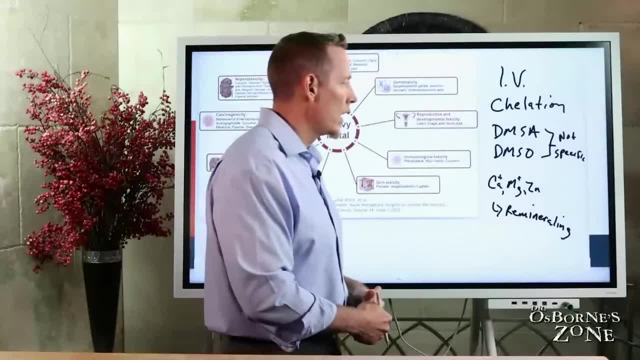 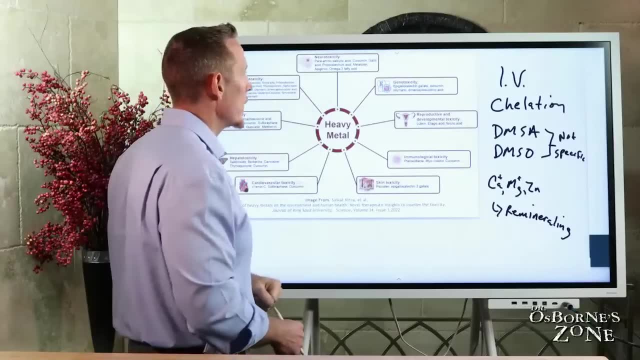 And although IV chelation is not the only option for chelation, there's nutritional chelation that can also be done. that will help pull and bind a lot of those toxic metals and support your detoxification as well. But let's just talk about some of the things. 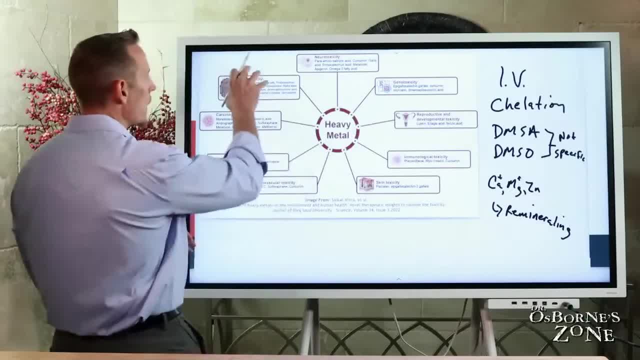 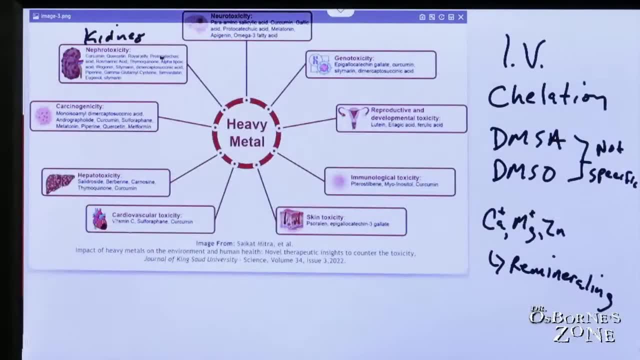 that can be done. I'll point a few of these out without reading. So for the kidney, you know their recommendation. there are a few things on this list that I think are worth pointing out, One of them being alpha lipoic acid, another one being silymarin, which comes from milk thistle. 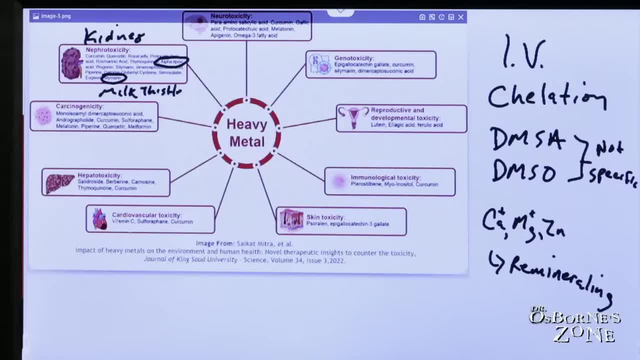 So these are just things that you can do to support your body's healing and repair in terms of kidney damage caused by metals. They also mention quercetin, curcumin right and royal jelly as options. I like quercetin as an antioxidant bioflavonoid. 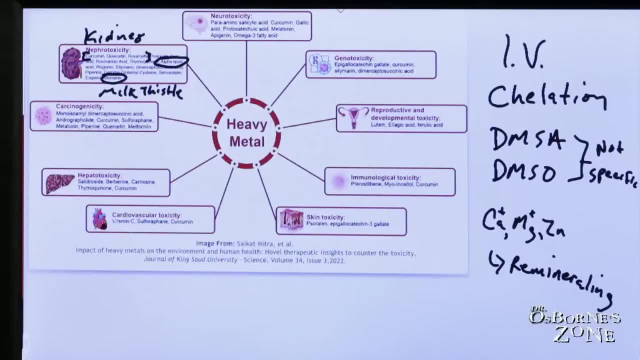 It's one of my favorite to use because it's so potent and so powerful And you can see for the carcinogenic effects. they're recommending some similar things here: curcumin and sulforaphane, which is an extract from cruciferous like broccoli. 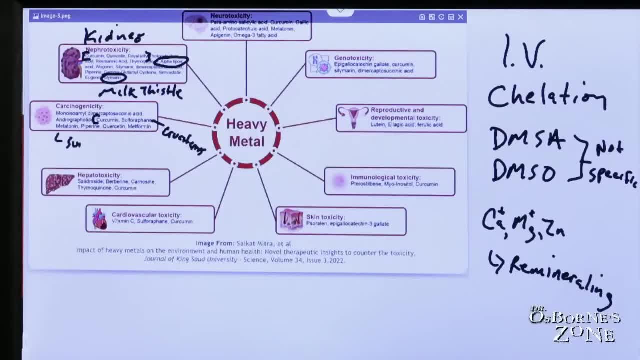 Melatonin which we get from sunshine. Best place to get melatonin for free is sunshine and getting plenty of it. And then again quercetin, Again there And then down. here you can see for the hepato or liver toxicity, curcumin okay, and berberine and carnosine all options here. 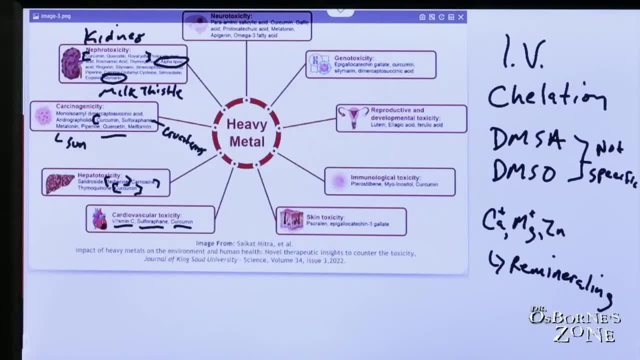 For heart toxicity, vitamin C, sulforaphane and curcumin, And for skin toxicity, epigallocatechin 3-gallate, which is generally- this is green tea- okay, founded green tea. So if you're a green tea drinker and you like your green tea, that's a way to get epigallocatechin. 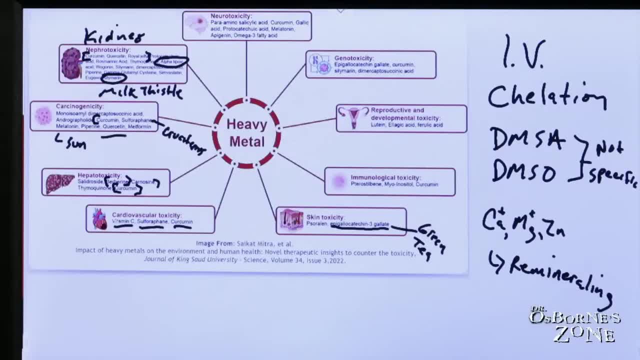 You can get it from apples. The skin in the apples contain that same substance as well. And then immunological toxicity, myo-nositol, nositol, which is a B vitamin compound, and then curcumin- Again, you see curcumin on a lot of these. 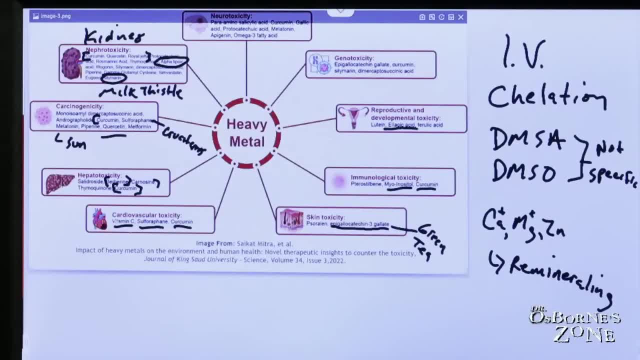 And then for reproductive toxicity, olagic acid, which is found in things like pomegranates and strawberries and some nuts, And then up here for genotoxicity, you can see again epigallocatechin, and then curcumin and silymarin. 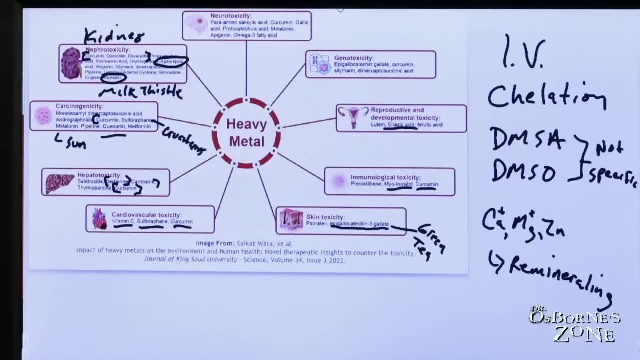 And then for the neurotoxicity, Neurotoxicity, again curcumin. So you see, if you're trying to hit all the right notes with all these things, I think a really good walkaway would be turmeric right, curcumin. 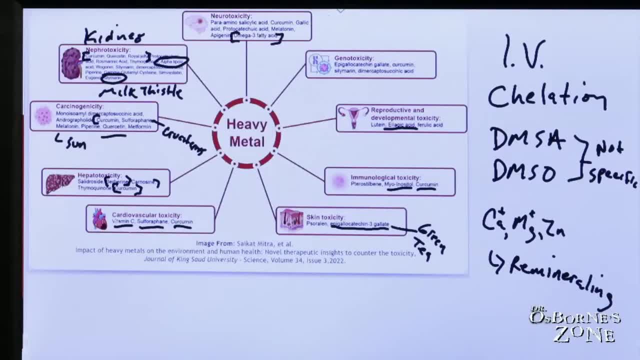 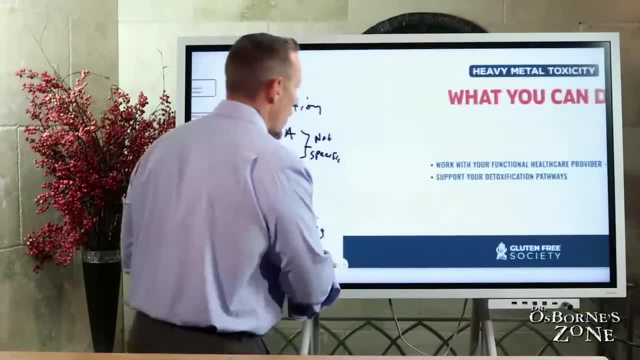 as a potential to give you some benefit of protection and support in terms of heavy metal toxicity. But I'm more of a fan of you. know what do you do in the long haul? What do you need to do long term? You've got to get the metal out of you. 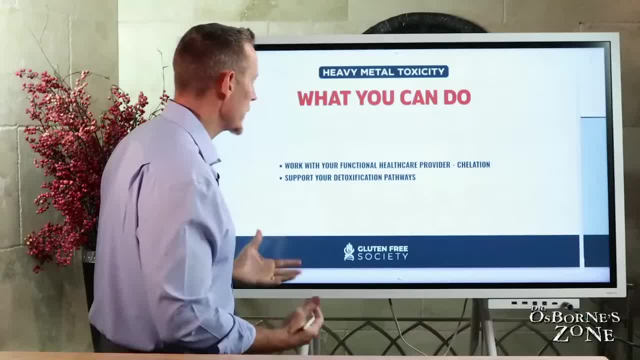 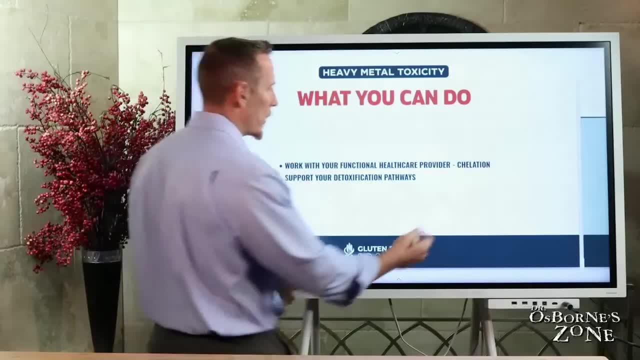 You just can't let it stay in you, And getting it out of you is. you know how do we detox? right, What can you do? Well, one of the things that you can do. One of the things that you can do is work with a good, functional healthcare provider and do a process of chelation. 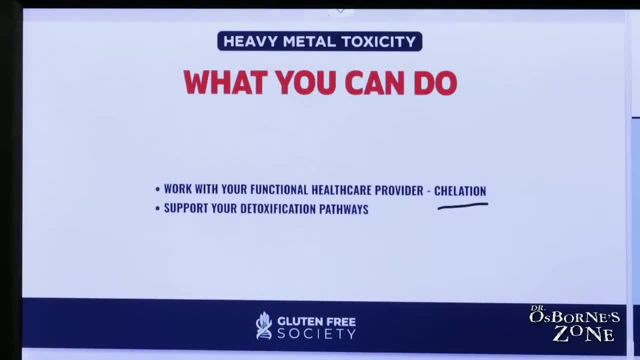 And I recommend, if you're going to do that, you work with somebody who knows what they're doing and can really help you. But what you can do is you can make better decisions that help support detoxification pathways. So how do you do it? 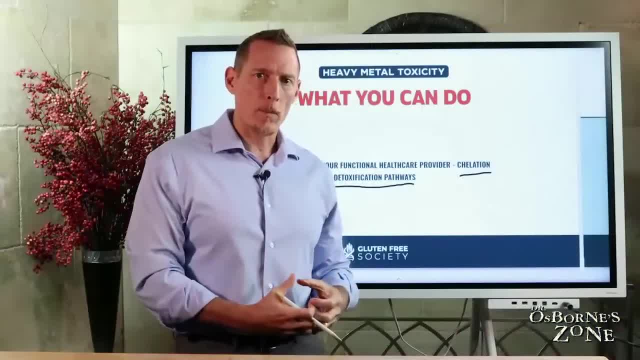 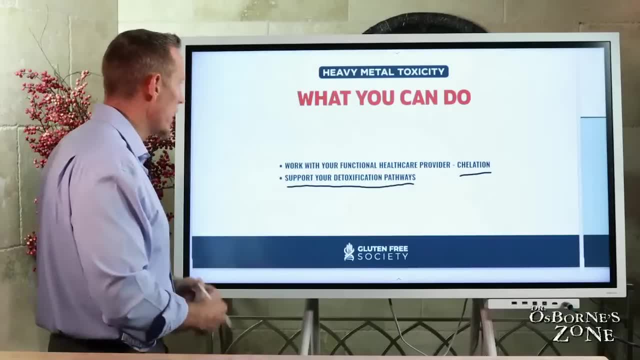 How do you make this kind of? how do you help yourself, protect yourself from heavy metals and help to get heavy metal out of you naturally? How do you support your body's ability to do that? Well, let's talk about that, Because there's different primary pathways for detoxification. 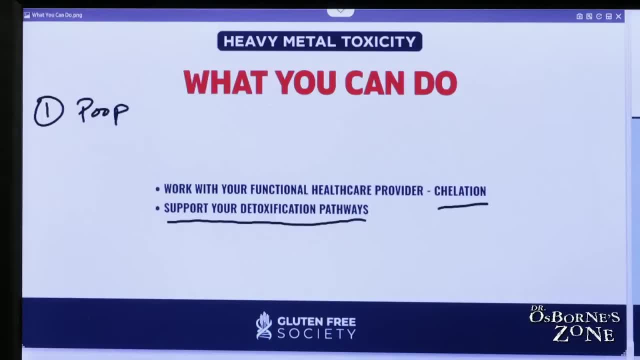 And number one is poop right, We have bowel movements, so we poop it out, And there's a process whereby our liver helps us to excrete toxins and poisons into the GI tract and we can poop those out. So you know, the enemy of detoxification is the opposite of pooping regularly, which is constipation. 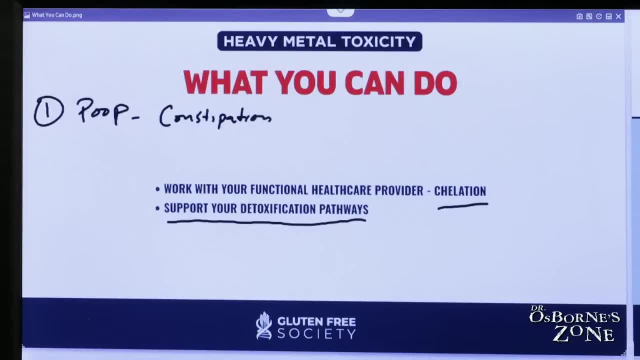 So if you are constipated, this is you know- you're blocking one of your primary channels of detoxification And so focus on that. Focus on making sure that you're doing everything to have healthy, regular bowel movements. Now I've done an entire show on constipation that you can go through and you can watch. 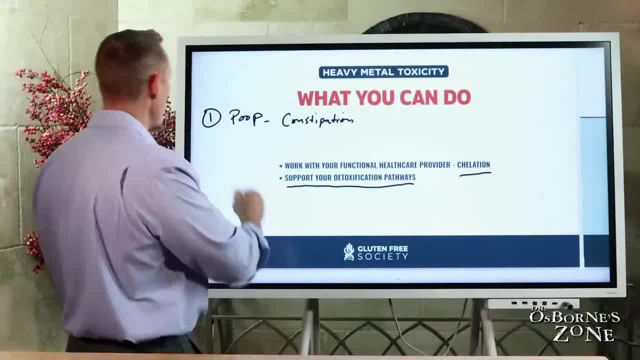 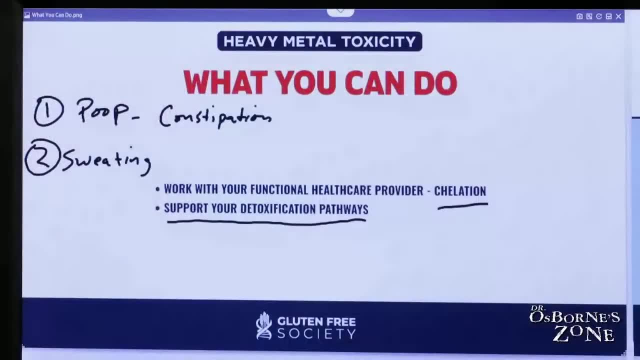 You just type that in on my channel and you'll pull that up if you want to dive deeper into that. Number two is sweating. We get rid of a lot of toxins through the skin itself. That's why a lot of the symptoms of heavy metal toxicity, as they're coming out through the sweat, can be inflammation of the skin. 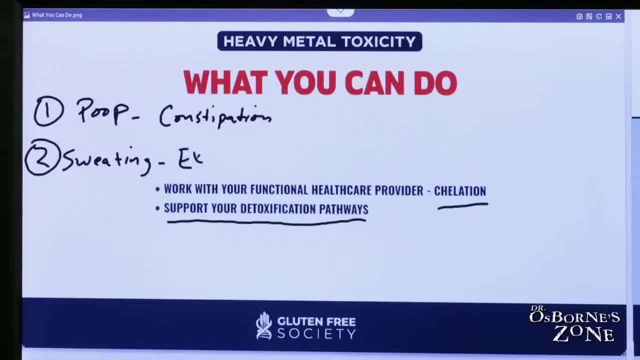 So sweating on a regular basis? Well, you know you can do that with exercise. Now, some people you know often talk about saunas, And you know one of my favorite types of sauna is infrared, because it goes deep. 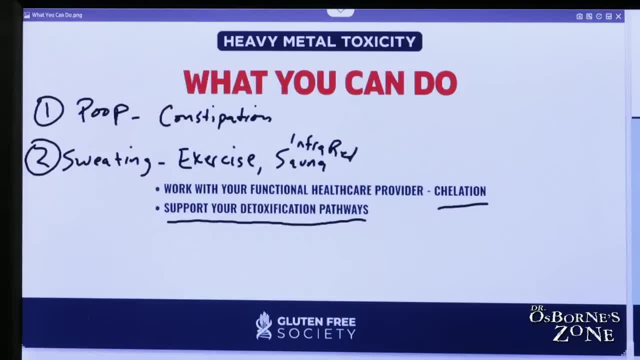 That light penetrance goes deep into the skin and can really pull toxins out and support that. So infrared sauna being a good way to sweat, exercise, in my opinion, being one of the freest ways and cheapest ways to sweat. You know, sunshine, going out on a hot day and being exposed to sun. 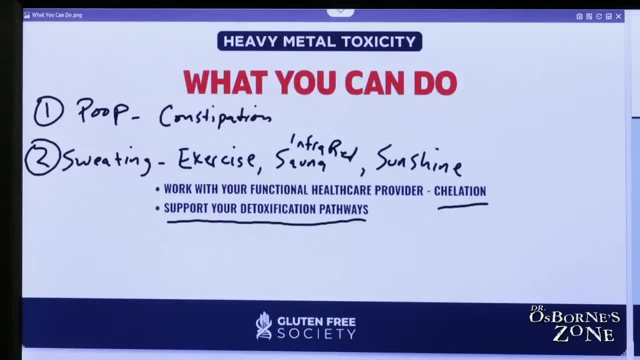 You know, sunshine Is one of the freest detoxification agents that you could expose yourself to on a regular basis. And the sunshine the distinction being: get good, adequate sun without burning. Don't go out so long enough to burn. And then number three is we pee it out. 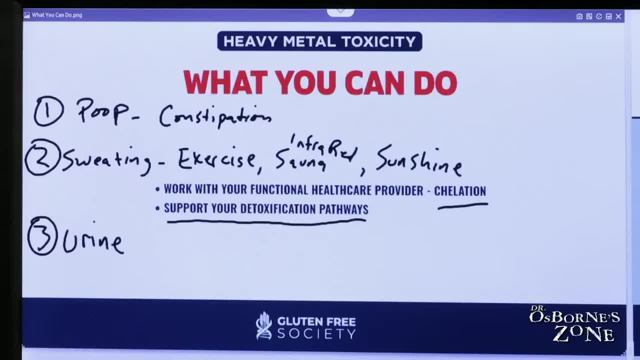 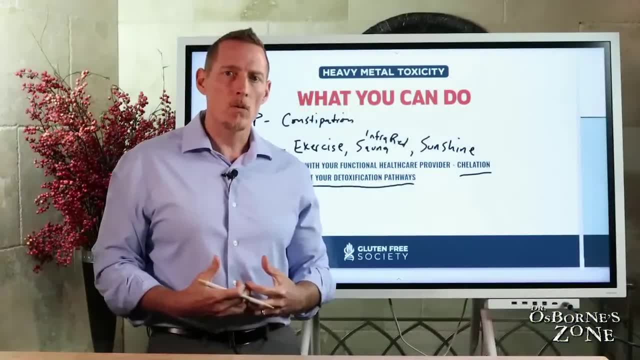 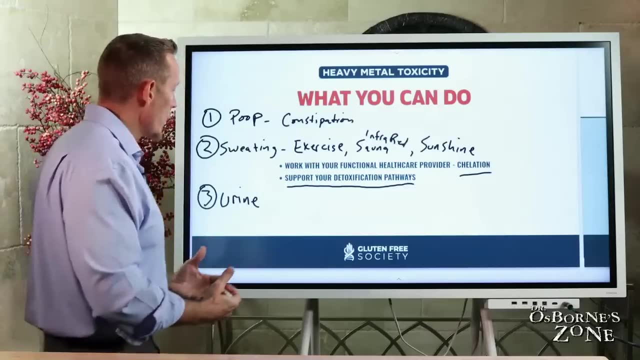 So urination is one way that we get it out, And this is where, like eating the right foods that act, as there are a number of different natural things that act as binding agents to heavy metals, And so you know, having these as a regular course of your diet, you know, one of them is foods rich in alpha lipoic acid. 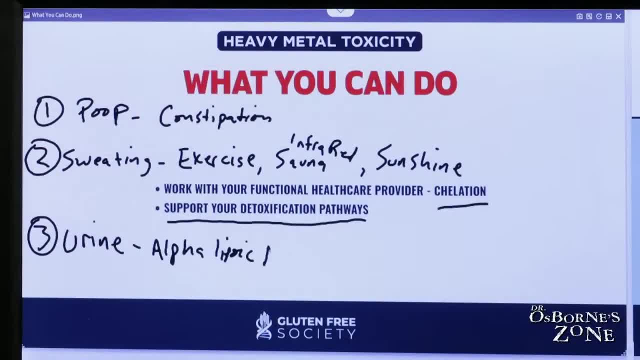 And there are a number of foods that contain lipoic acid, But also, in addition, is foods that are rich in NAC, N-acetylcysteine. These are sulfur containing foods, So cruciferous vegetables would be an example there. 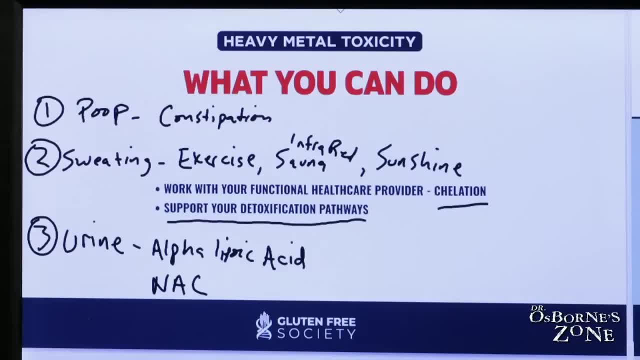 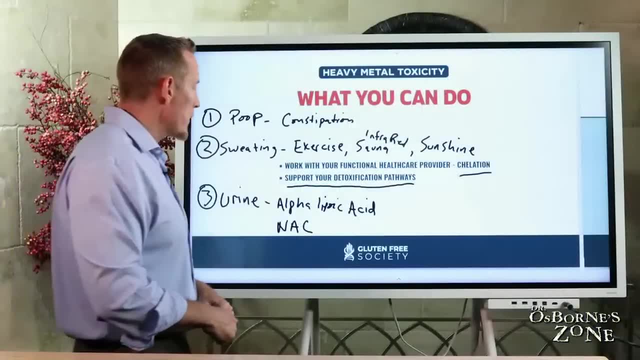 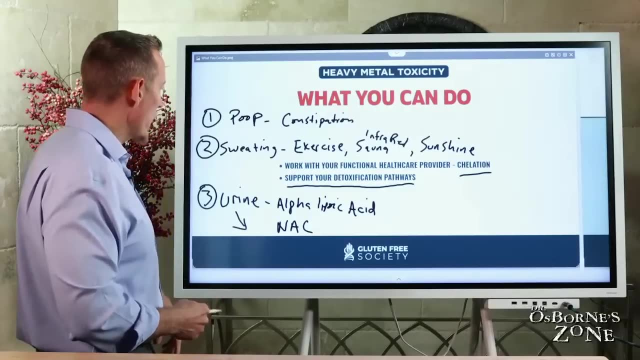 Eggs would be an example there. But you know, consuming foods that are high in nutrients that we know have binding agent properties or detoxification properties to help your liver, you know, basically metabolize these things into water-soluble agents that can be excreted out of the urine, and then the fourth way is through. 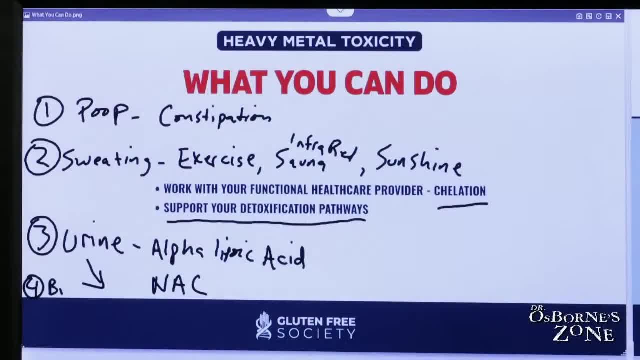 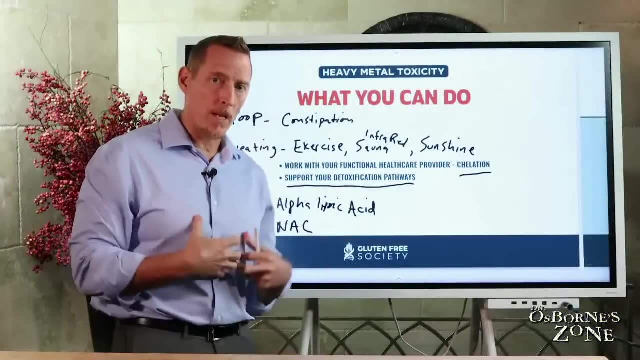 breathing. a lot of people forget about breath work and breathing as being important for health, but your lungs have a just a very, very powerful antioxidant system that is designed not only to prevent chemicals from that we breathe in, from damaging them, but also from allowing us to expel chemicals as they're. 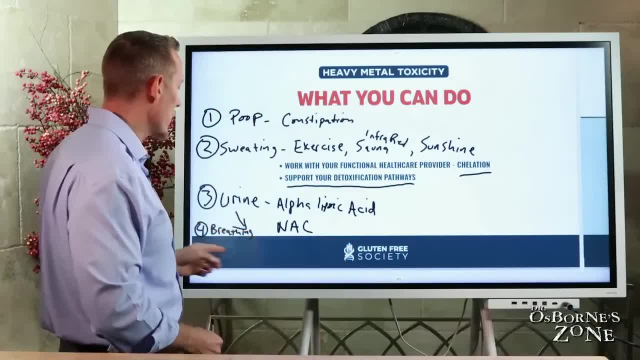 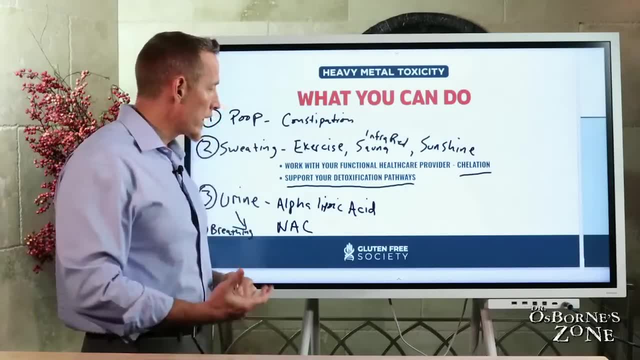 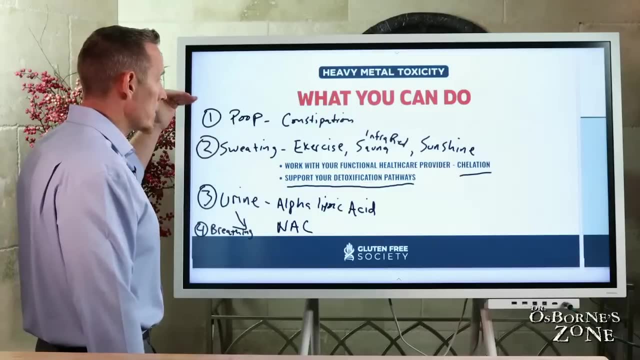 being metabolized through in our bloodstream and then find their way back to the lungs. so deep breathing can be very, very valuable tool in a detoxification protocol. so don't forget to breathe. so these things you can do pretty much all these things here are free for the most part, because they're 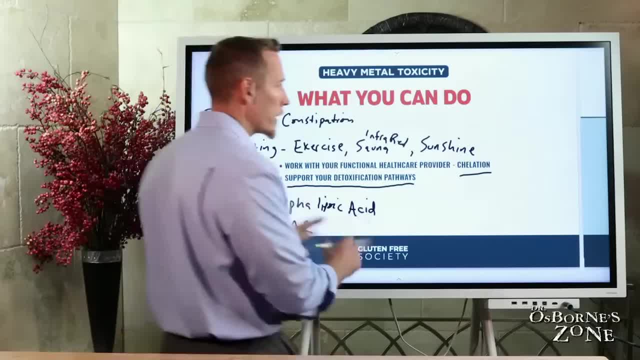 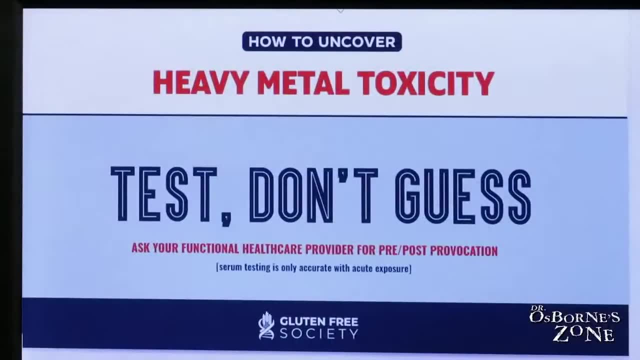 just choices that you get to make every day. now, beyond that, if you're working with a good functional practitioner, you know the key, that the key message I can give you right is right here: test, don't guess. you know, I get a lot of times where people say, yeah, my doctor wanted to do chelation. 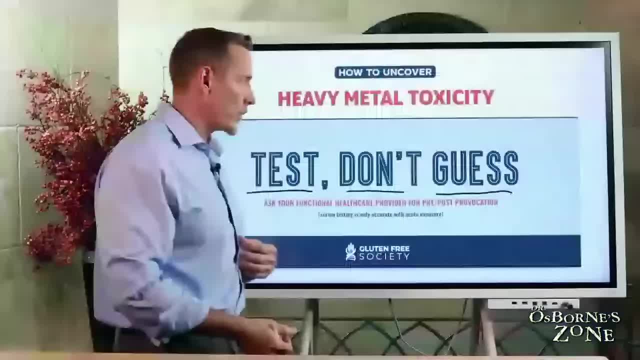 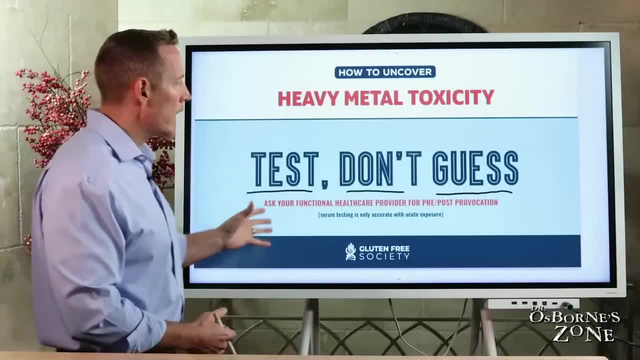 and they never even did a test to see if they needed to do chelation. remember that, that the testing gives you the knowledge and the confidence to know you're doing the right thing, and so what kind of testing is best for heavy metals, in my opinion, and 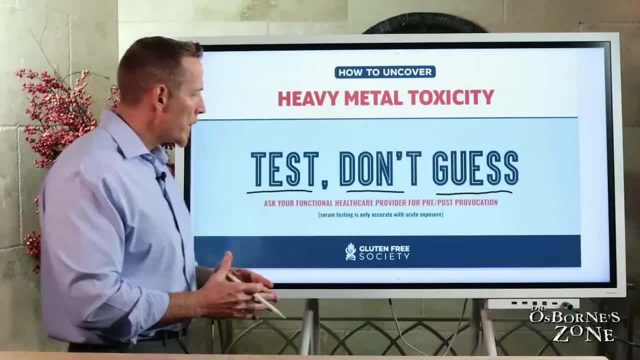 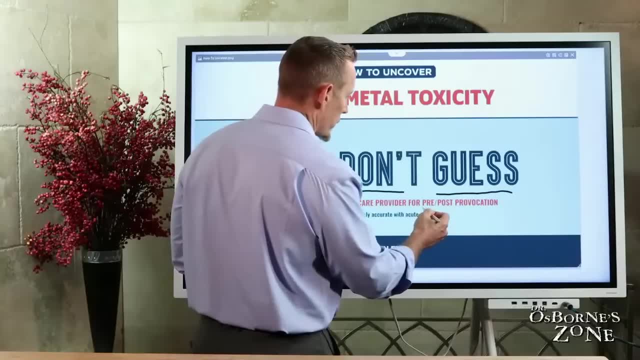 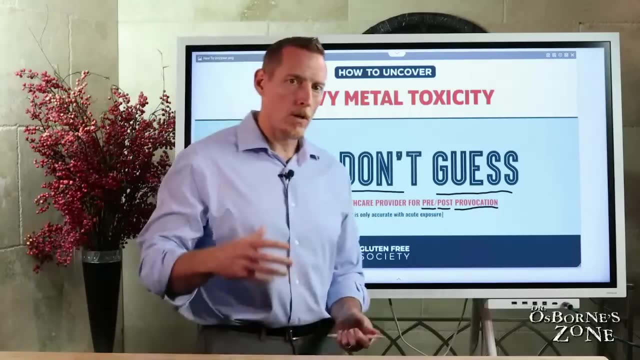 there are different opinions out there. I'm going to share mine with you. the best way to test for toxic chronic bioaccumulation of heavy metals is this: right here is called a pre post provocation test, and this is where you it's a urine test, and so you give a urine sample and that's pre. so the first. 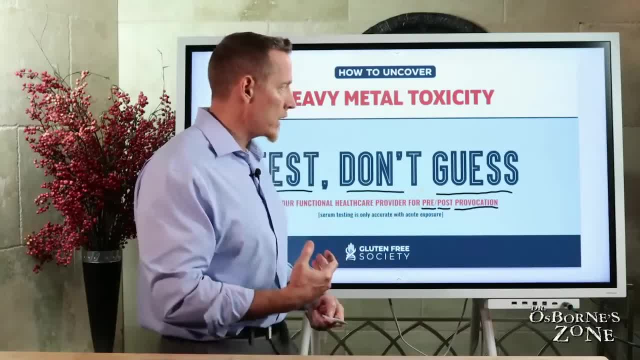 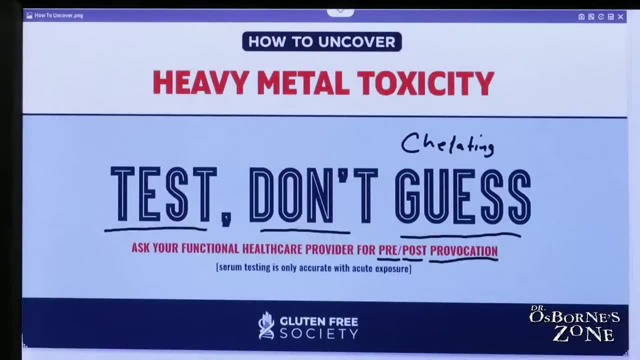 thing you do is a collect urine and then you take chelating agents again chelation chelating agents. one really good one that's over-the-counter that many people take is something called EDTA, which is a natural chelating agent. mix that with 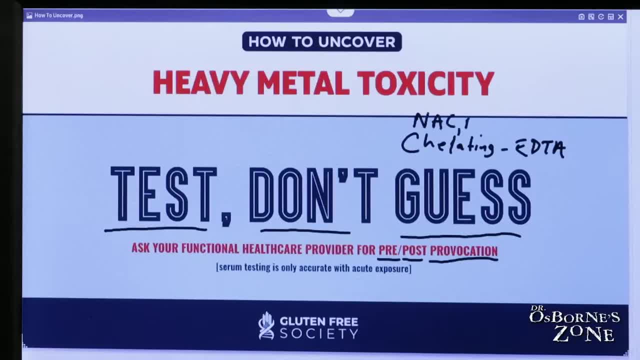 some knack and some alpha lipoic acid and some garlic and you've got a heck of a chelating oral oral pill that that you know. that would suffice for the second part of this test, which is the post, which is where you take a dose of these things and then you collect urine for. 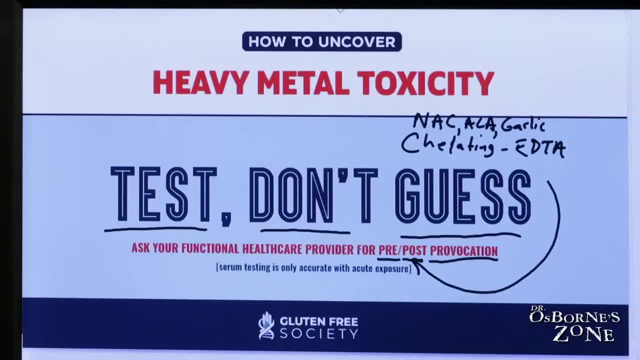 several hours, and then you're measuring to see what kind of heavy metals are coming out. this again pre and post provocation. the pills they contain. these types of substances are the provoking agents, or what are called provoking agents, and so if you're working with a healthcare provider, they'll know what. 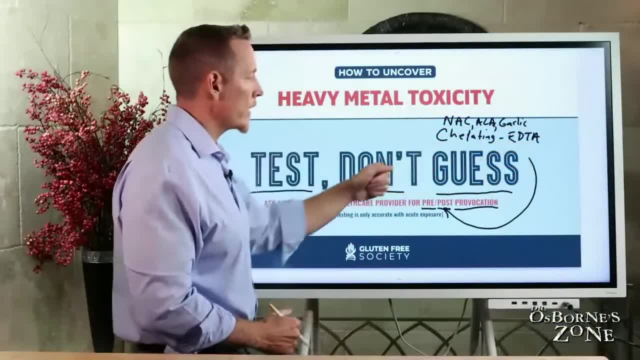 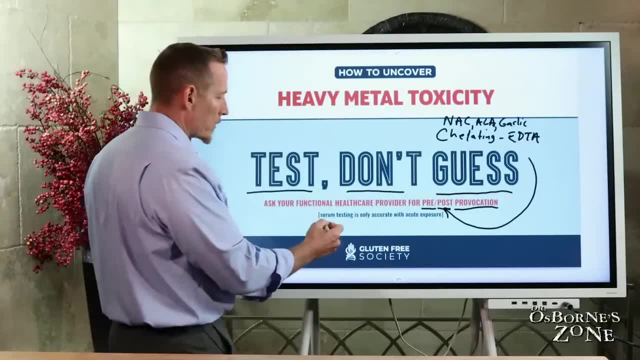 that means and they'll know and probably will have an idea of what they would want to use to test you. so test, don't guess now serum testing. a lot of people bring this to me and they say, yeah, my doctor tested me for mercury or my doctor tested me for lead, and they bring back a. 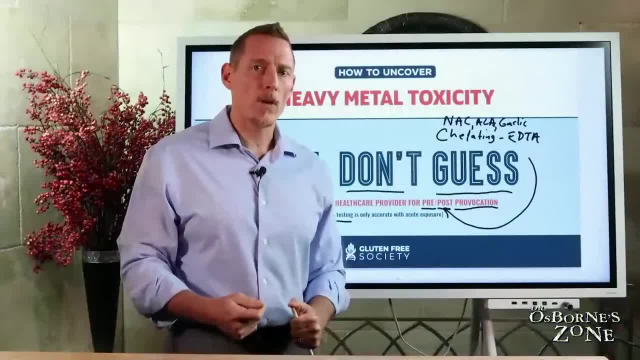 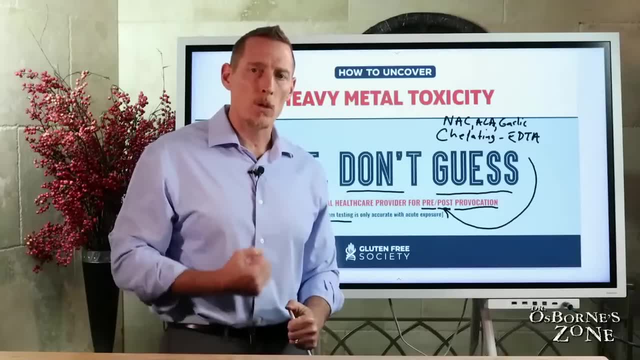 serum test, and serum tests are really only accurate if you've had an acute poisoning. they're not real super accurate because your body will take the metals that you're slowly exposed to and it stores it into your tissues to get it out of the circulation. it doesn't want it in the circulation because metals are. 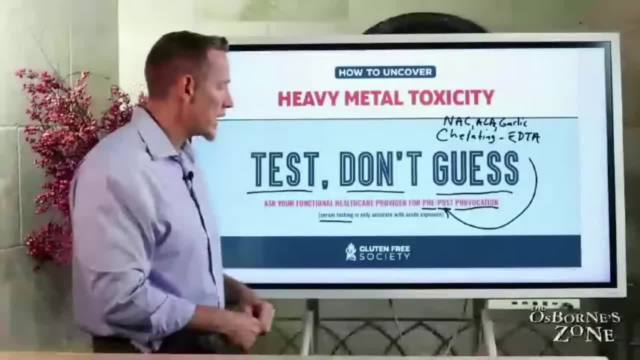 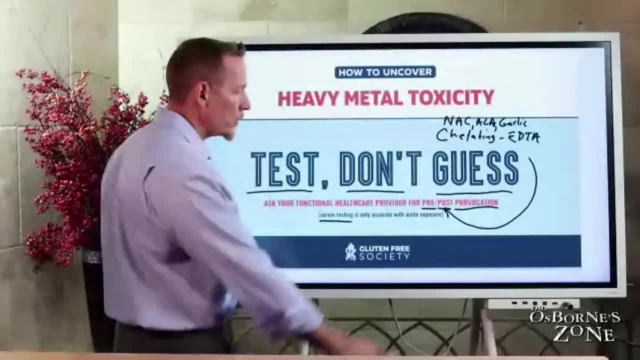 reactive and toxic, so your body will store it in tissue to get it out of the circulation, from preventing it from creating a lot of bad bacteria and it's going to cause a lot of bad bacteria and it's going to cause a lot of bad bacteria getting a reaction, and so serum testing is only accurate when you have an acute. 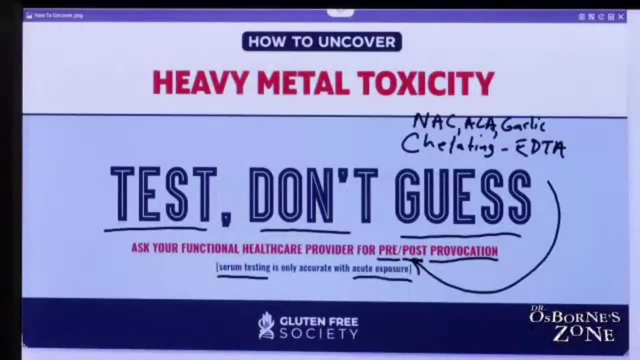 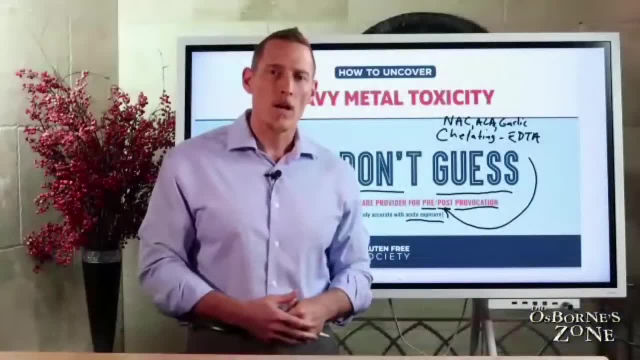 poisoned exposure. so if you suspect somebody's trying to kill you- you know, you've ever watched these criminal shows on TV late at night where the husband's maybe trying to kill the wife with arsenic, or you know something like that- that then maybe serum testing might be a kind of a more accurate way for you to. 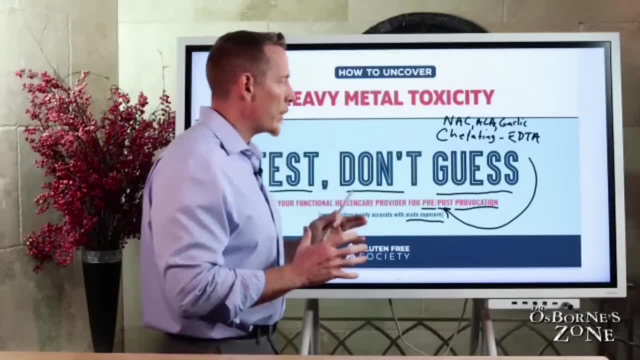 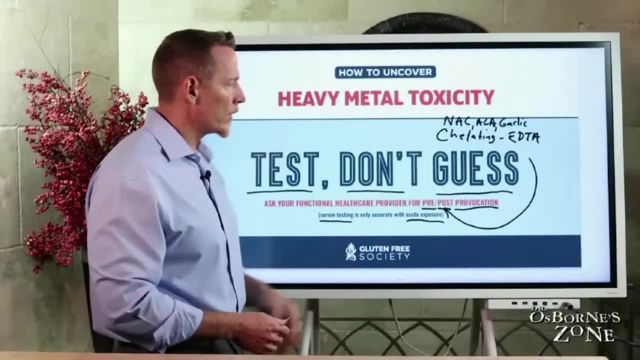 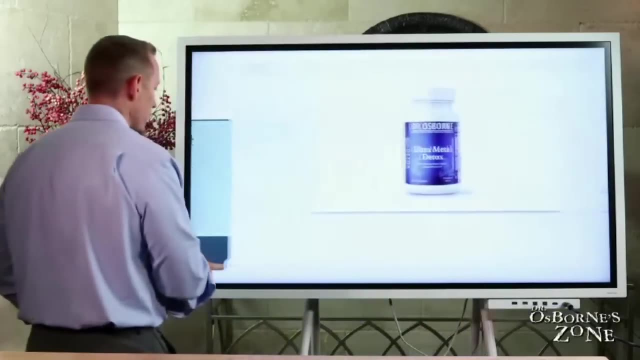 get that answer. but at the end of the day, if you're trying to understand about bioaccumulation, pre and post urine provocation testing is hands-down one of the best ways to investigate for heavy metal toxicity in my experience and in my opinion. so test, don't guess, and then work with that expert. now, if you're just looking for, 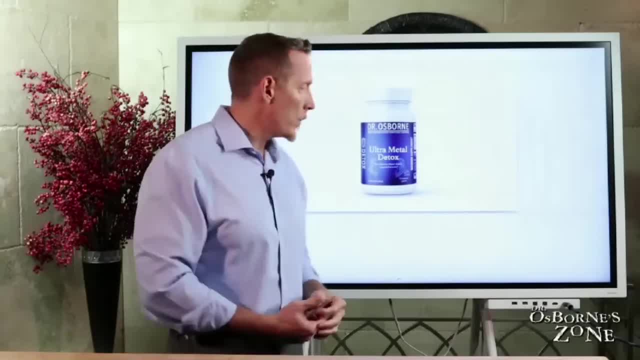 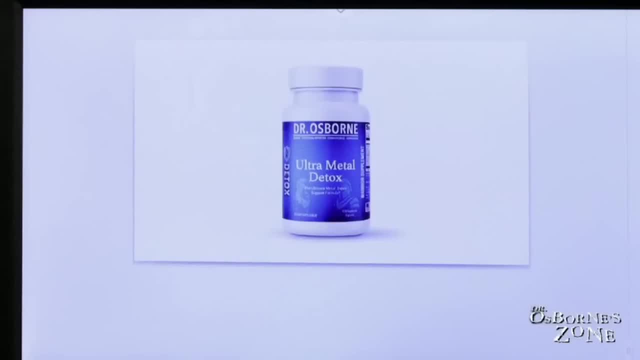 some natural detoxification support. one of the things I created is a formula called ultra metal detox, and so what this does is it just helps with liver detoxification. it helps your liver, support your liver in doing that. it helps with kidney function and it also contains, instead of 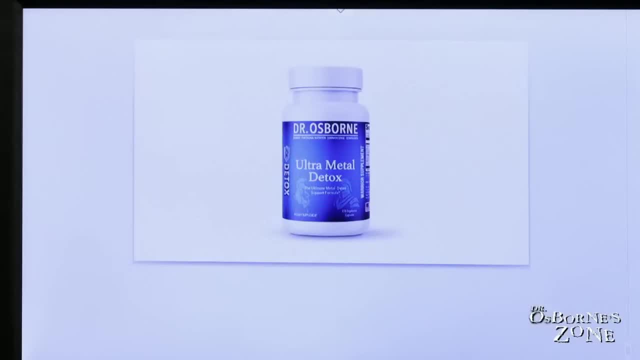 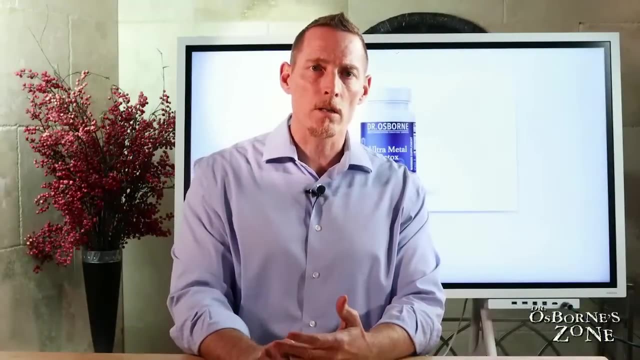 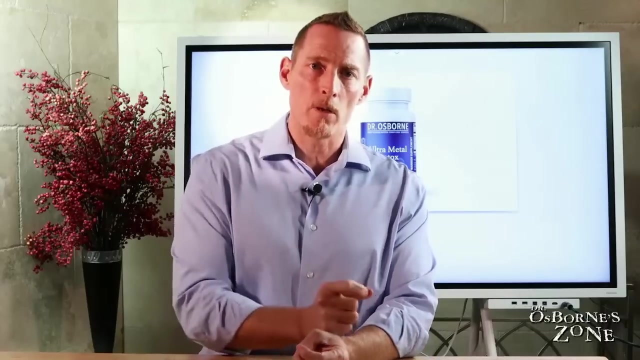 just pulling. remember I said that, that any kind of chelating agent doesn't select for good or bad metals, it just pulls metal. but but this formula has something in it called Sheila jeet, which is a very, very mineral, dense substance designed to help support remineralization of the body, if you're. 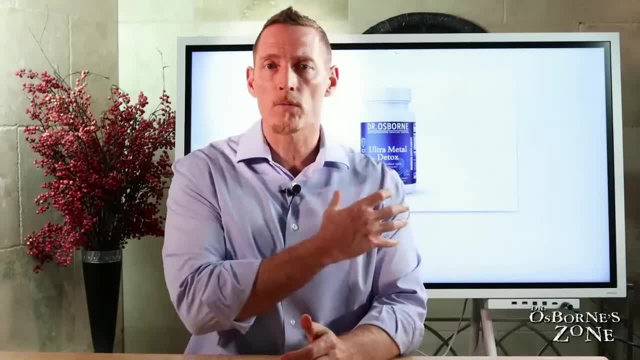 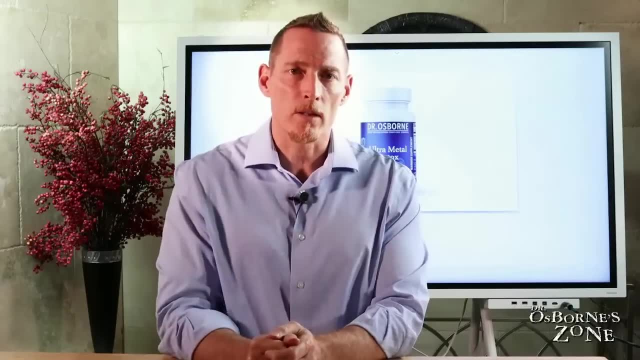 doing any type of chelation. now, if you're doing something like this, it's more for support. you just want to be cautious. you don't want to just take a you know an overabundance of it indefinitely not, not ever investigate deeper. but if you are just trying to take a, 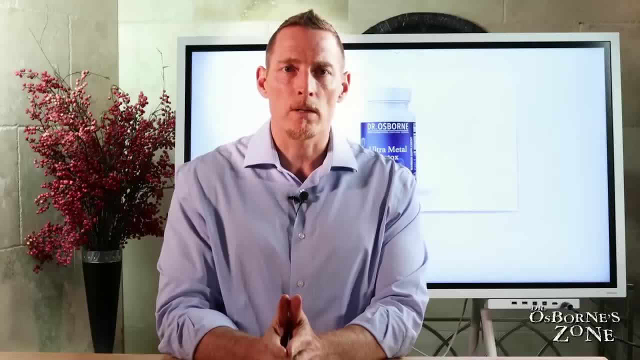 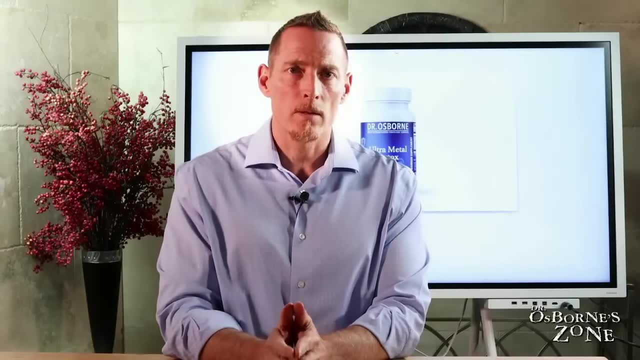 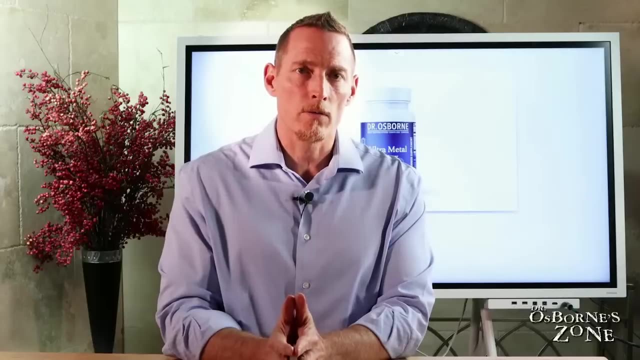 supplement that supports your ability to detox metals is something you can take- one to two capsules of a day- and it's just part of your support program. but at the end of the day it's always best to test, not to guess. if you suspect you've got a heavy metal issue, you need to probably get in and work with a good 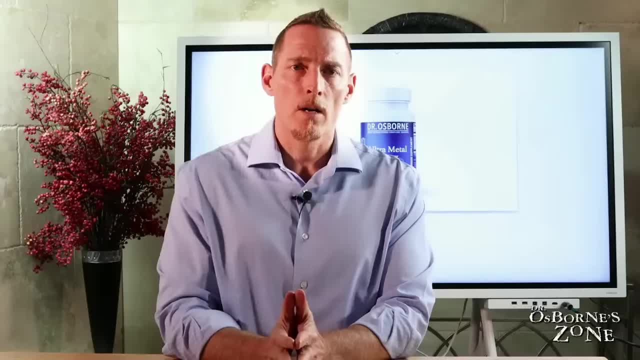 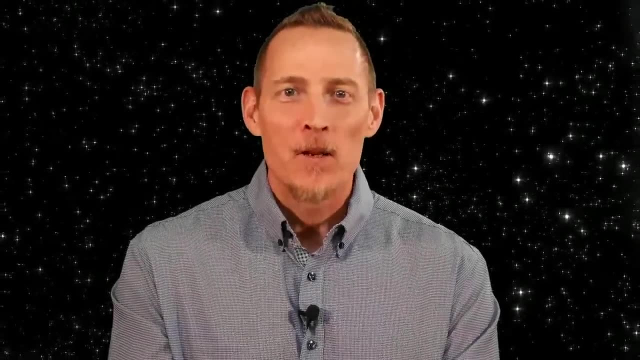 functional doc or somebody well versed in this stuff to get the help that you need, so that you're not just wondering or trying things that may not be helpful for you in the long run. thanks for tuning in to the dr Osborne zone. don't forget to share, like and subscribe. 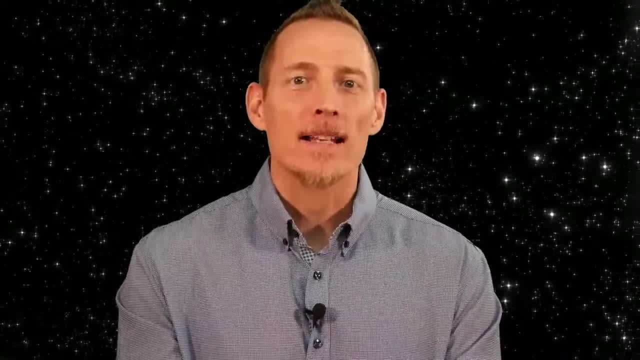 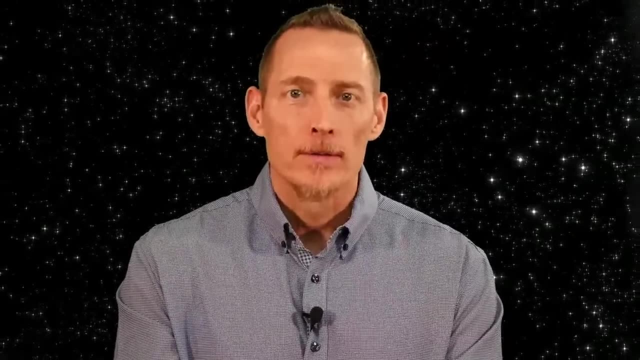 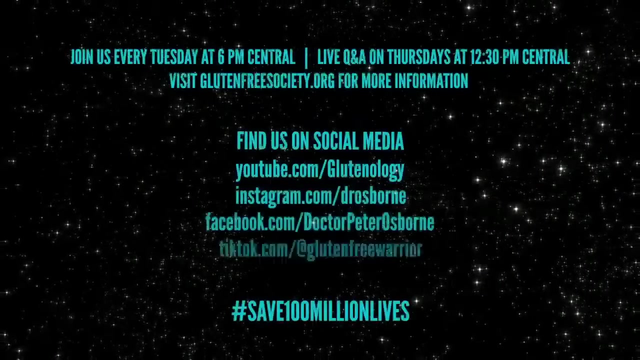 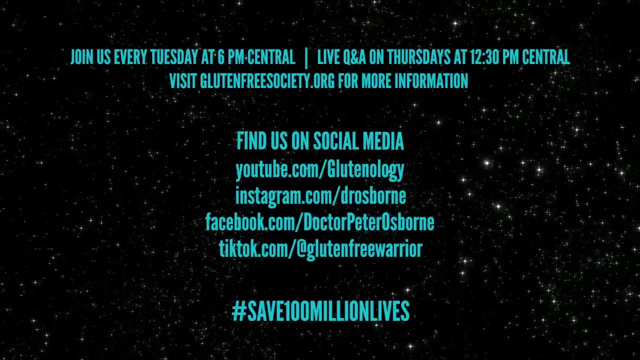 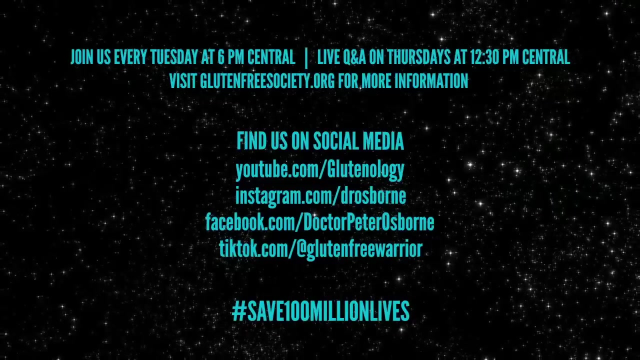 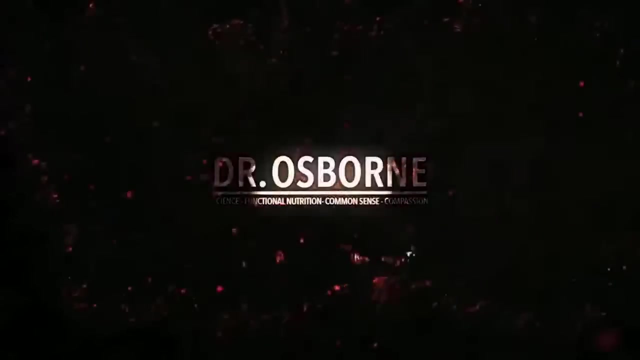 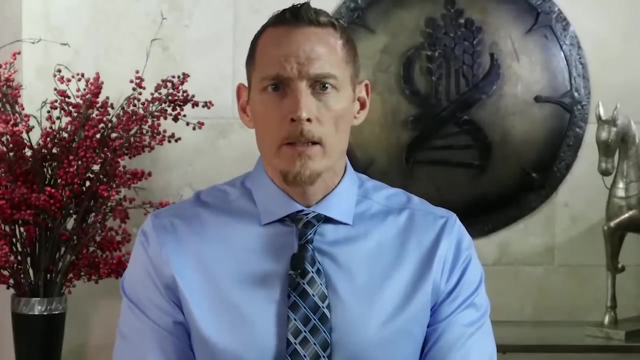 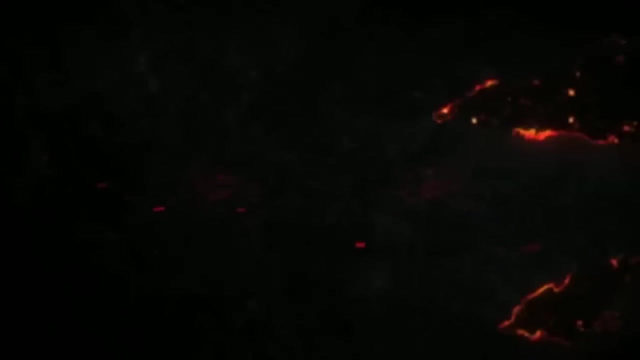 for more content like this and make sure you come back next Tuesday at 6 pm Central Standard Time and Thursday at noon 30 for more episodes. did you know that research shows that heavy grain and gluten consumption can contribute to high tissue levels of heavy metals like mercury, arsenic, lead and cadmium? that's